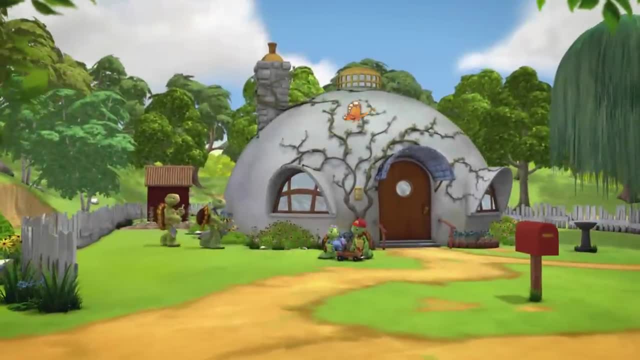 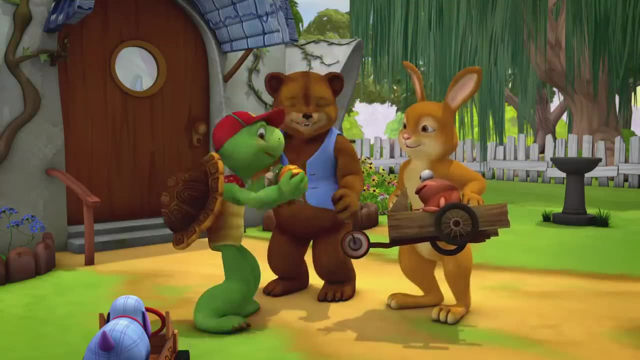 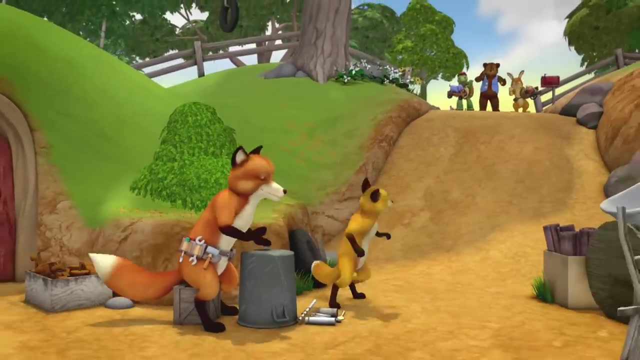 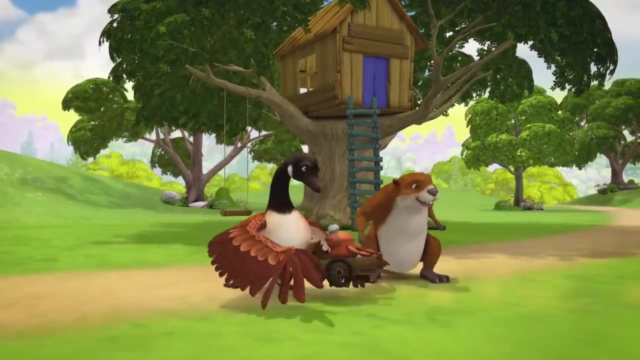 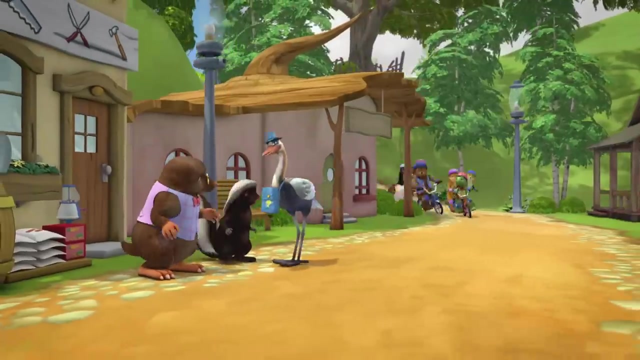 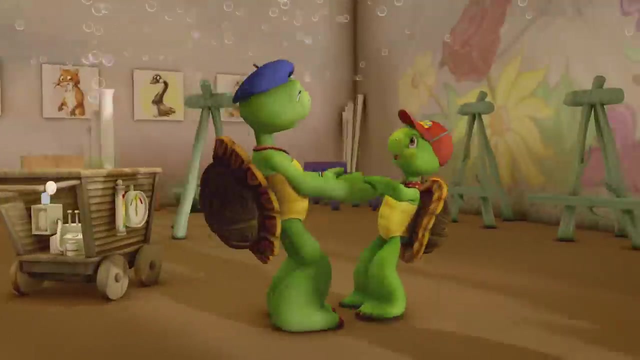 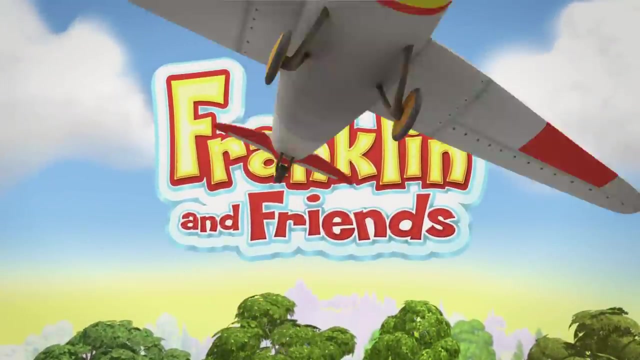 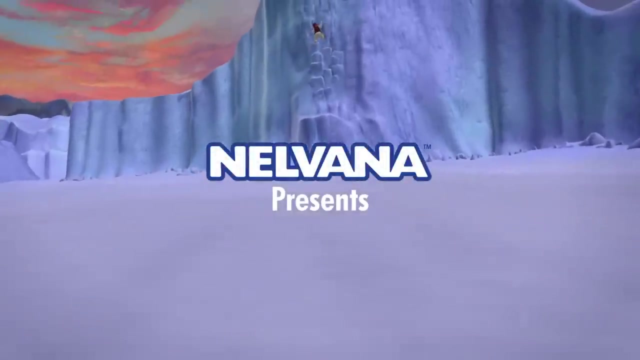 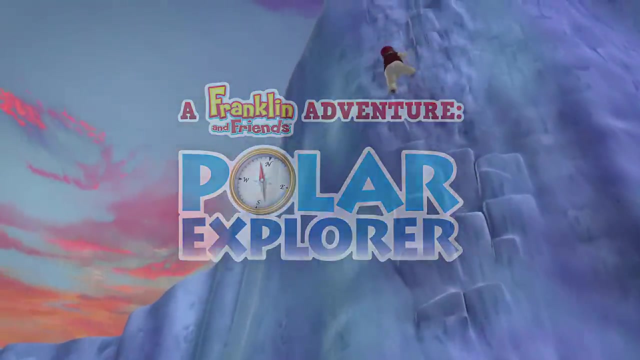 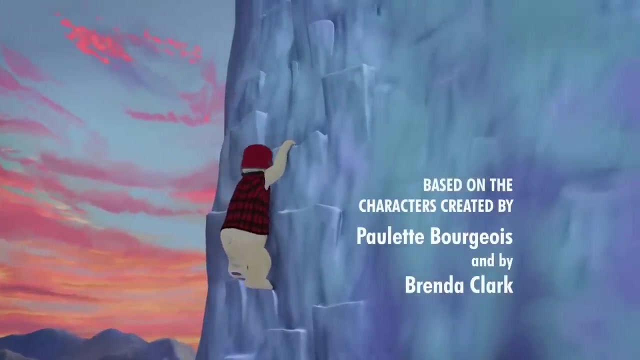 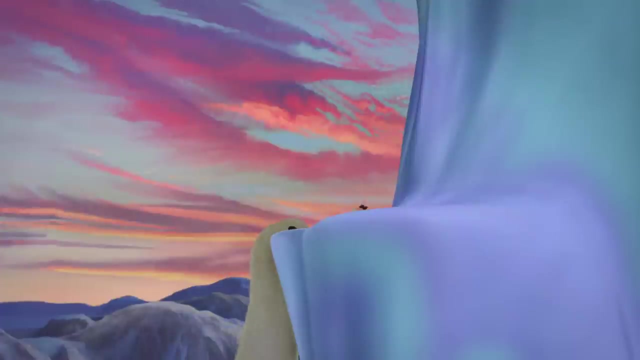 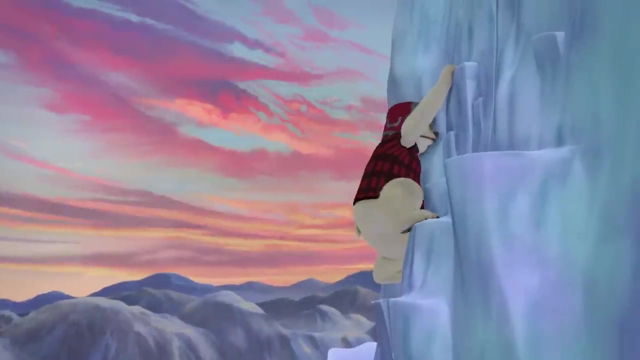 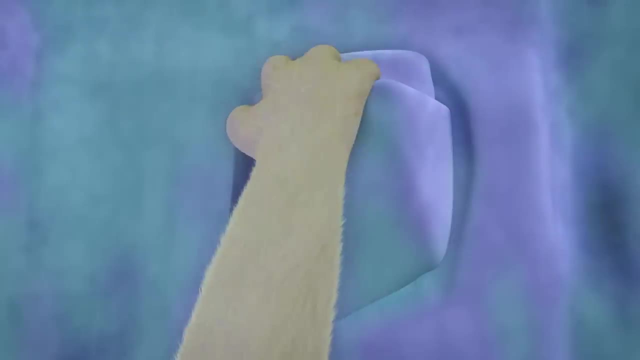 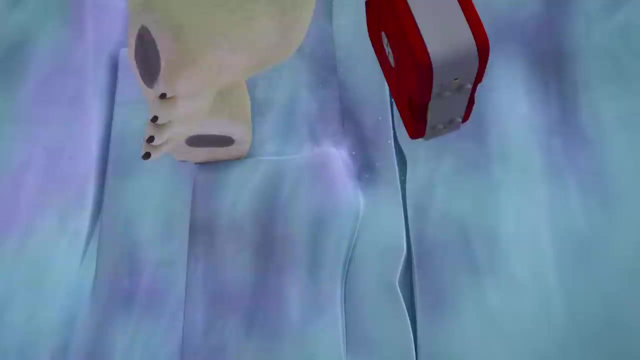 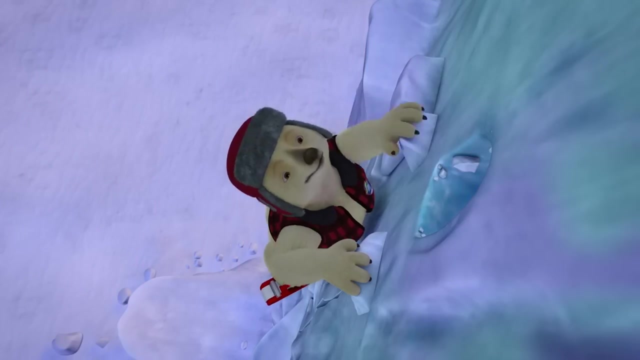 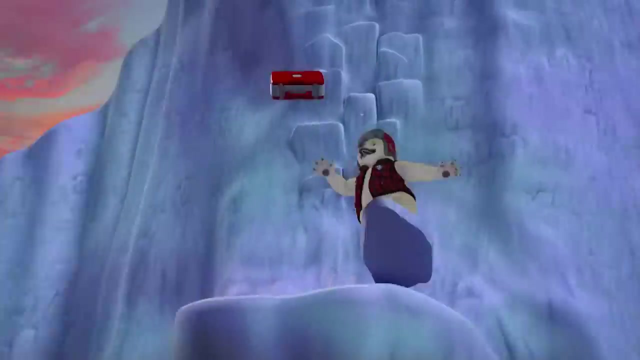 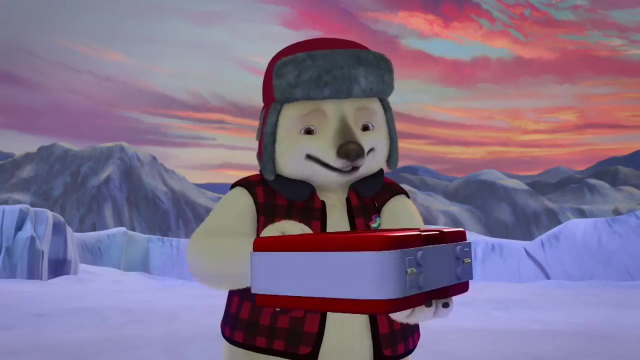 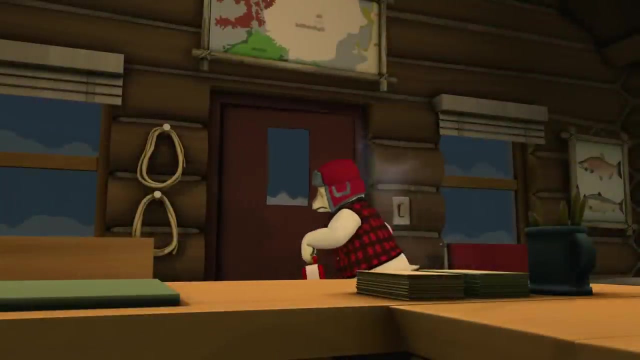 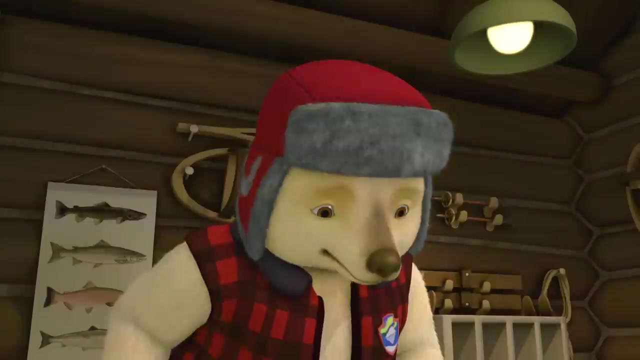 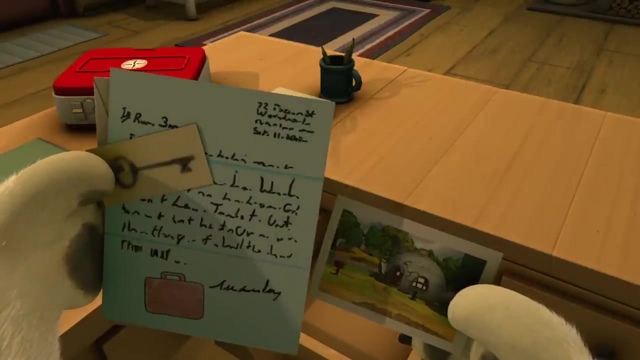 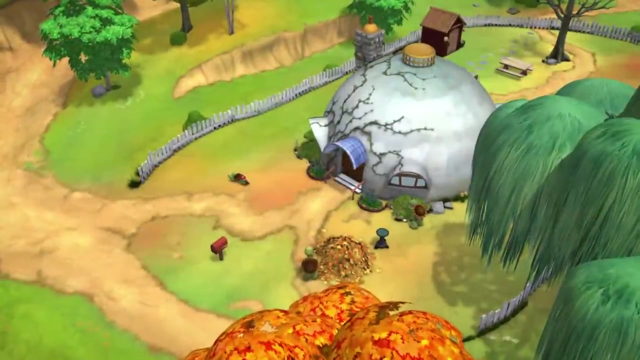 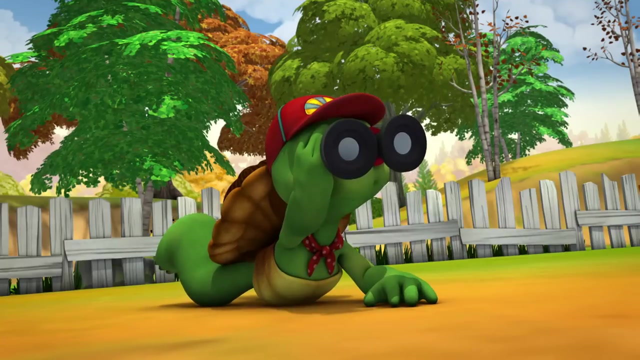 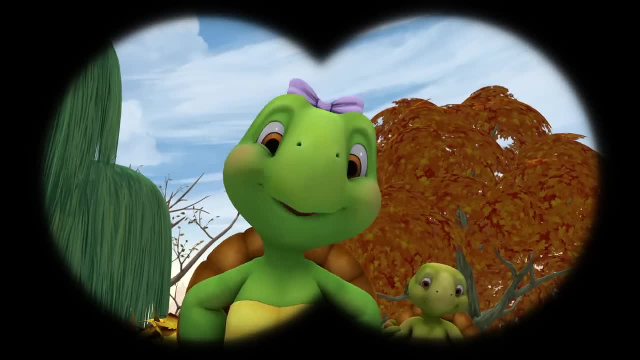 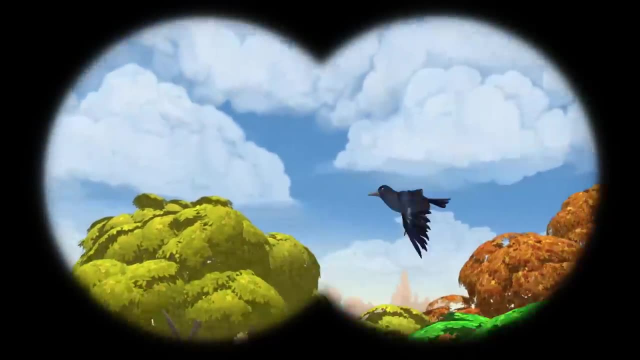 What will he find next? What are you doing, Franklin? I'm an explorer. I'm looking for adventure and new discoveries. Is that him? Is it a plane? Nope, it's just a bird. He'll get here, sweetie. His letter said he'd arrive sometime today. 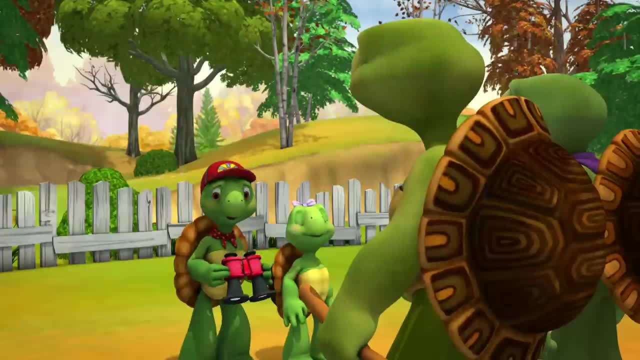 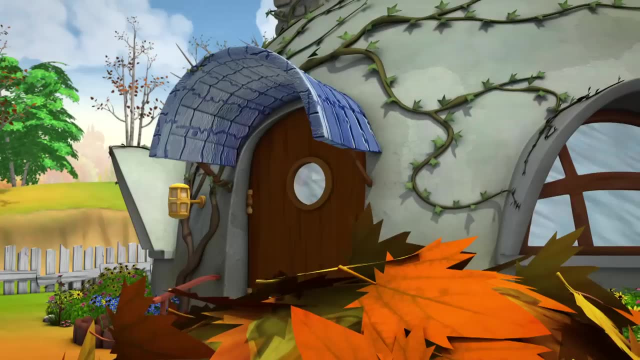 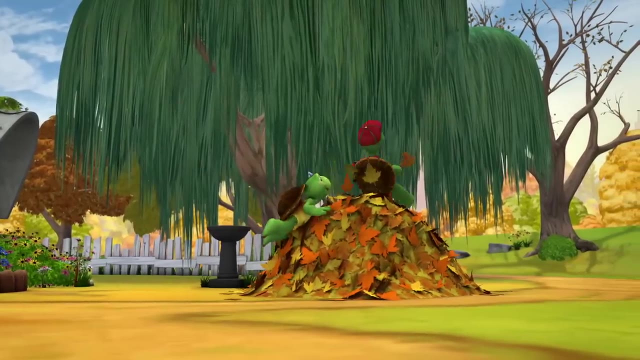 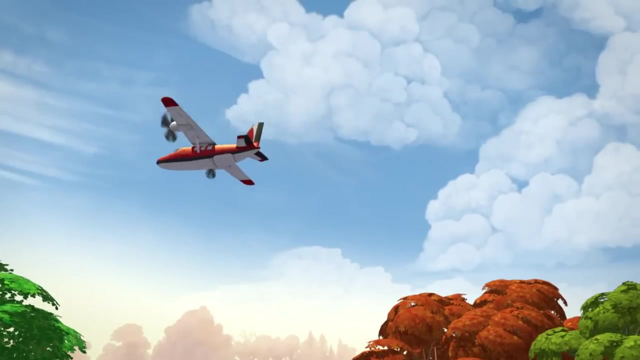 It is a big trip. He's way from the Arctic, I know. I just hope he gets here before bedtime. Hey, Franklin, watch me. Whee, Good one. Harriet, Wait for me. Whoa, Hey Dad, do you think that's him? 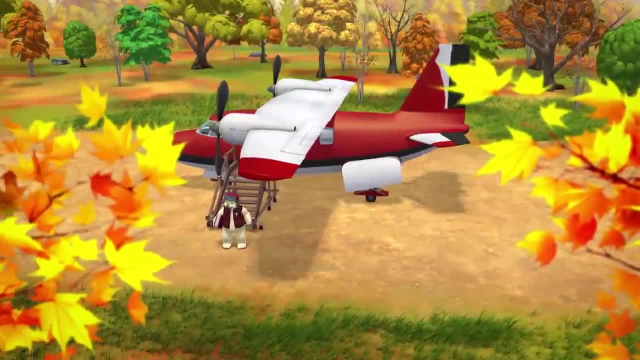 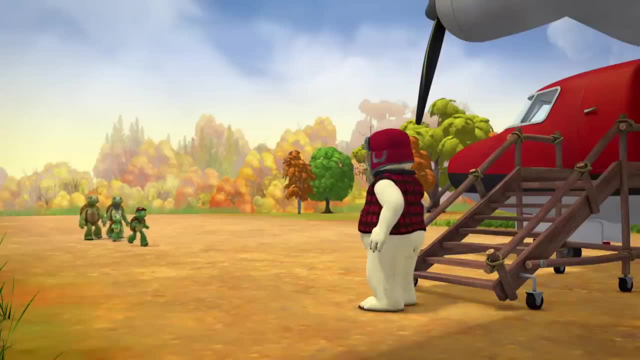 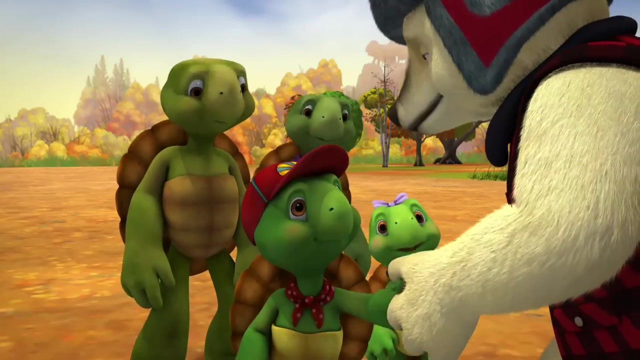 It just might be. Ah, look at these colors. It sure has been a while. Ranger Bear, I can't believe you found the explorer box. Well, hello there. You must be Franklin, Pleased to meet you, Hi, Ranger Bear. 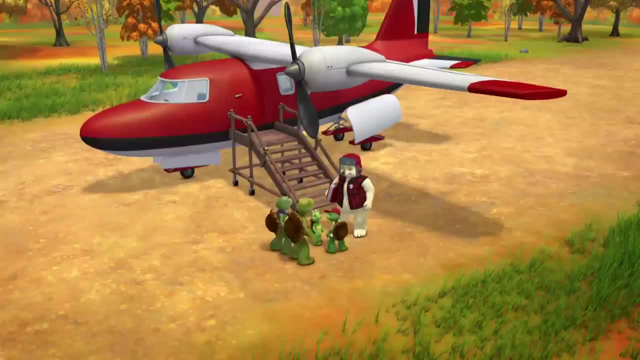 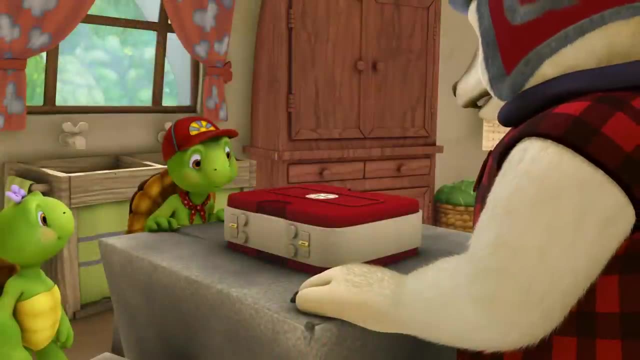 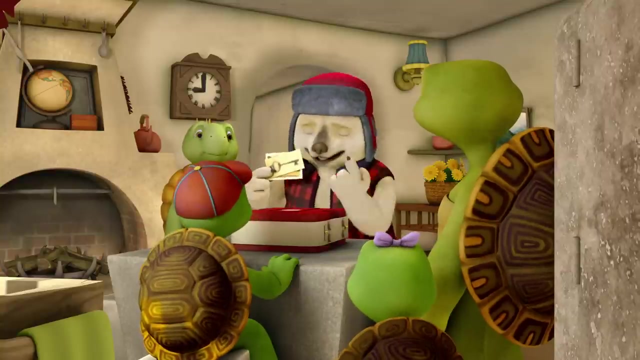 And hello to you. Welcome to Woodland Ranger Bear. You must have had a long flight. Please come relax at our house. Thank you, Mrs Turtle. Now, as I was saying, when I saw this explorer box, I remembered getting this young fellow's letter and his drawing of the key. 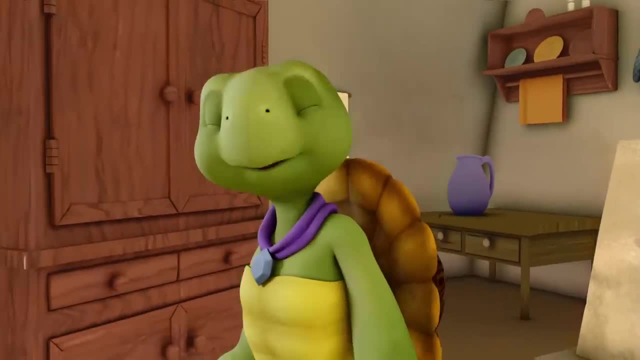 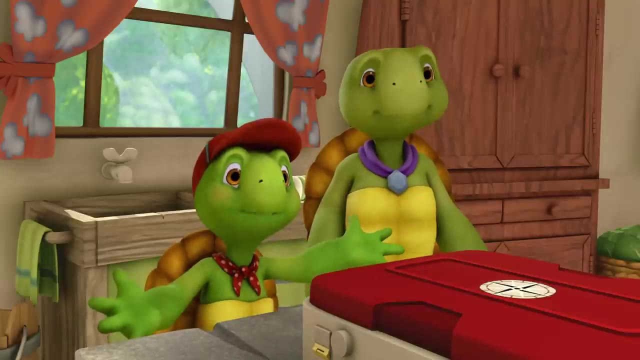 Franklin's Great Aunt Harriet, gave him a key and told him it opened a special box but that the box got lost on a northern expedition. She said if I ever found the box it would lead me on a great adventure. So I sent letters to all the ranges in the north hoping someone would find it. 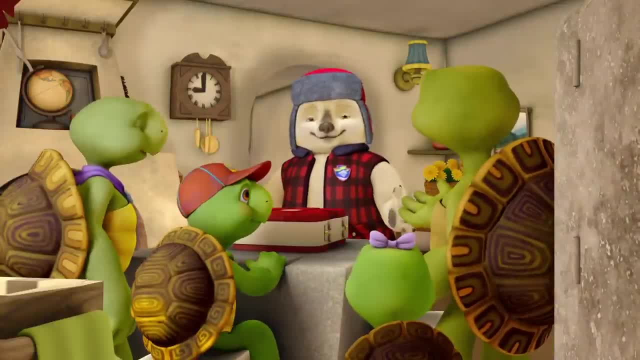 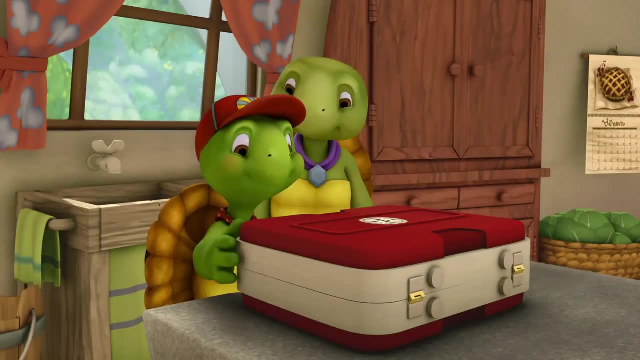 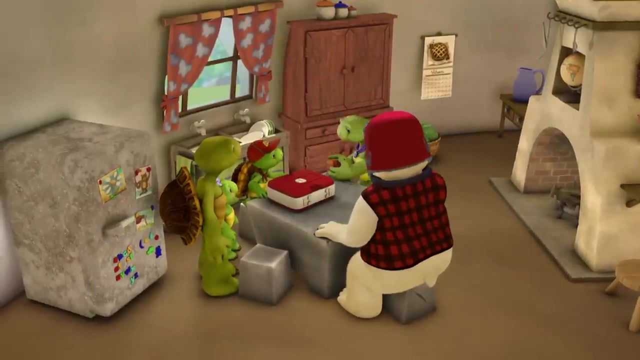 Well, here I am. Thanks for hand-delivering it. My pleasure. It gave me a chance to see your beautiful woodland. Whoa, I'll get the key. Great Aunt Harriet wanted to be here for a while, But she's exploring in the rainforest right now. 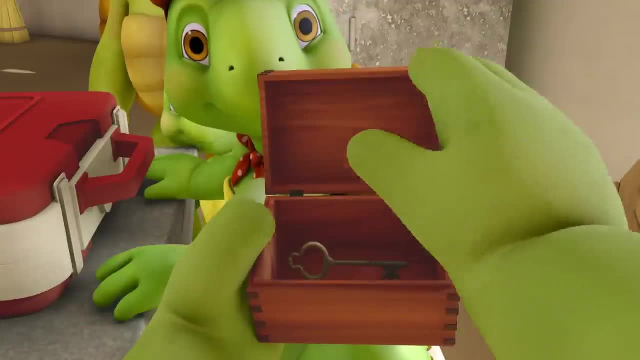 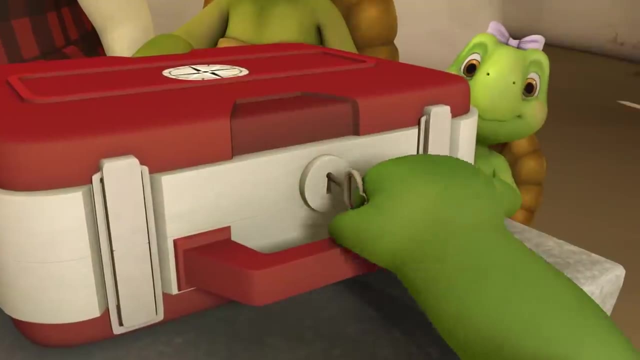 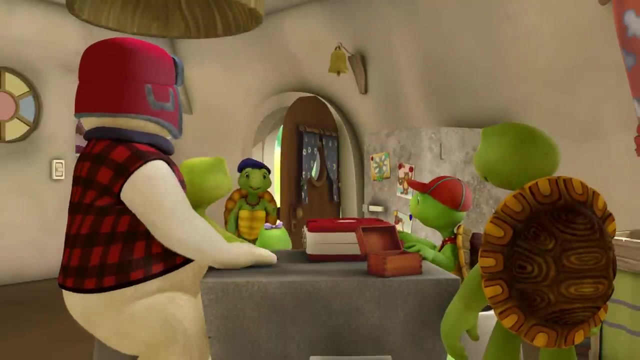 It's hard to believe she still goes exploring after all these years. Go ahead, Open the box, sweetie. Here it goes, It fits. Whoa Sis, Am I late? Did I miss anything, Auntie? Oh hey, sweet pea. 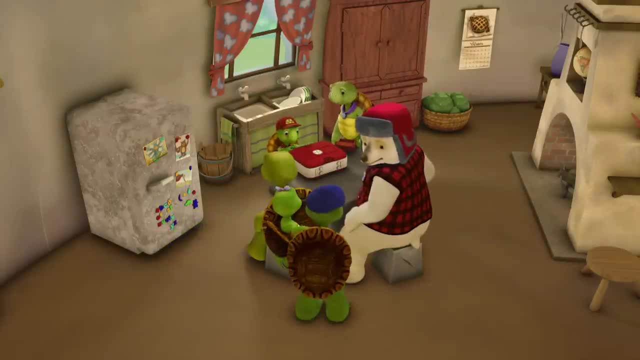 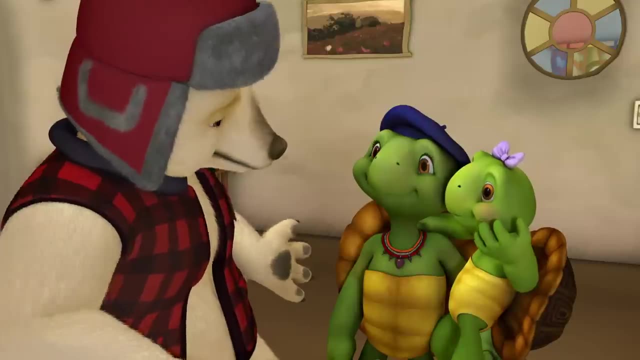 Franklin's about to open Great Aunt Harriet's box. Go ahead, Franklin. I'm Auntie Hi. Ah, Ranger Bear Pleased to meet you, Okay. okay, Here I go. Whoa, Look at all this cool little stuff. 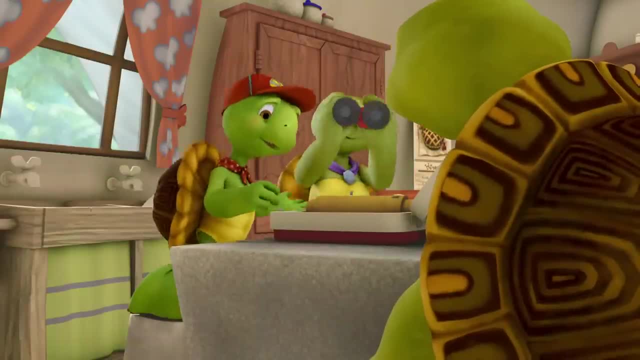 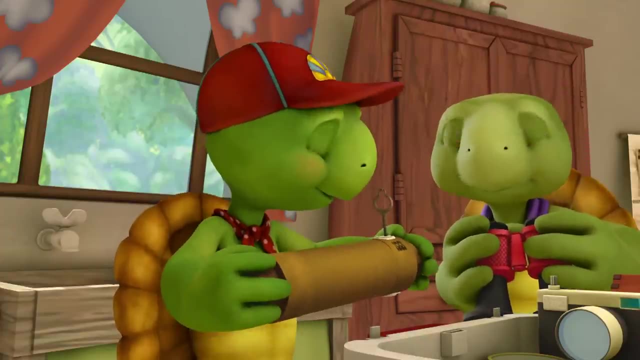 Binoculars, a camera, a compass, a? Oh, What is this, I wonder. What is it? There's a key in the first keyhole. It kind of looks like some sort of code bar. You know, I've heard of explorers using gizmos like this to keep their secrets. 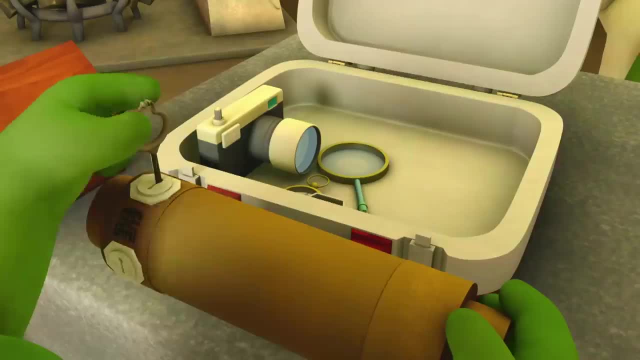 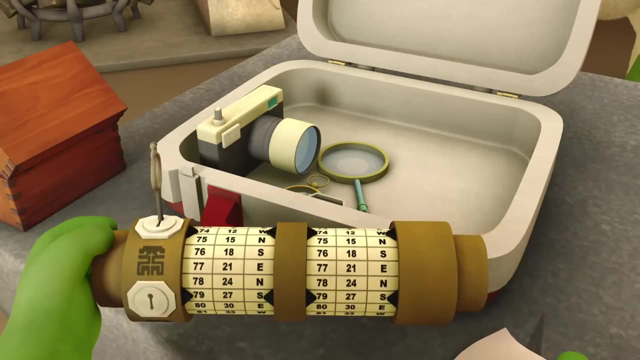 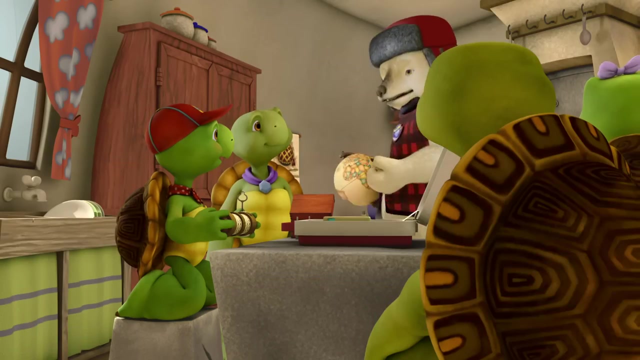 I'm going to try it. Let the adventure begin Interesting. But what do these numbers mean? Ah, allow me. Those are longitude and latitude numbers. Explorers use them to find spots on the globe. As it happens, where these numbers meet is at a spot right near my ranger's station. 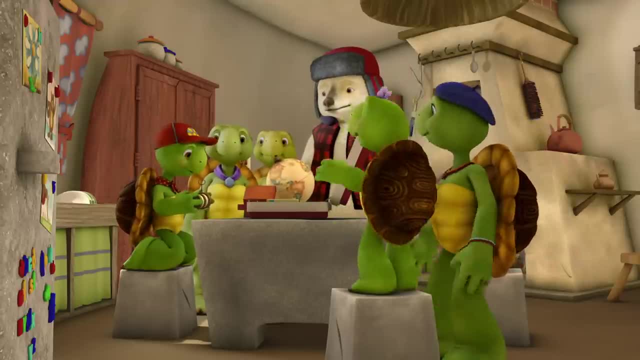 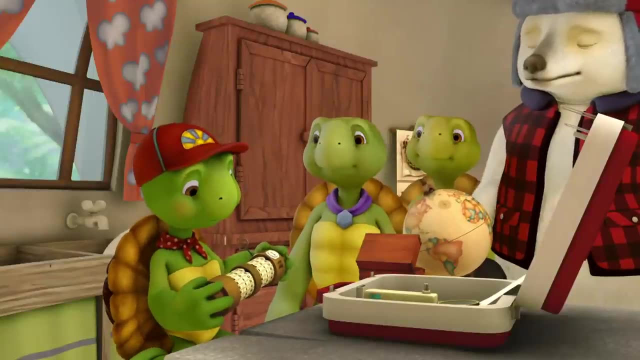 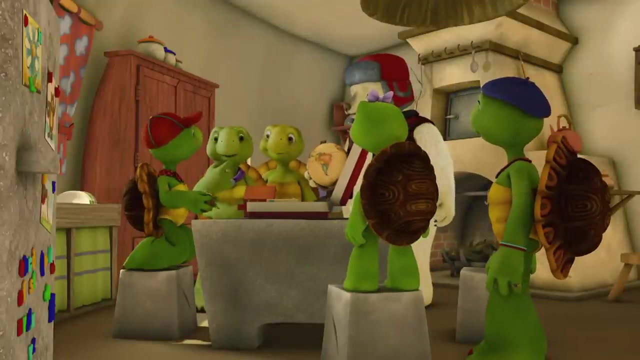 Wow, I wish we could go there. Try the next one, Franklin. Okay, Here it goes. Oh, Doesn't work. Maybe those numbers are just the first clue to the adventure Great Aunt Harriet wants you to have. Something tells me that if we go to that first location, we'll find a way to unlock the next clue. 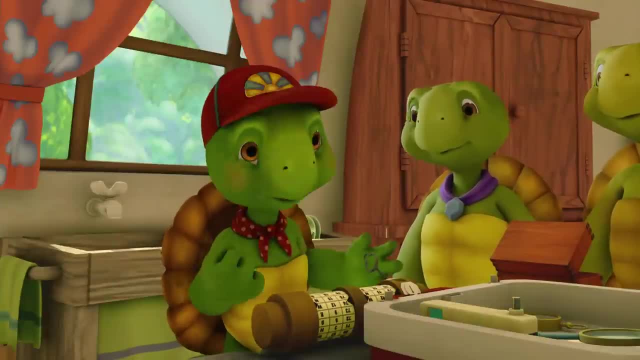 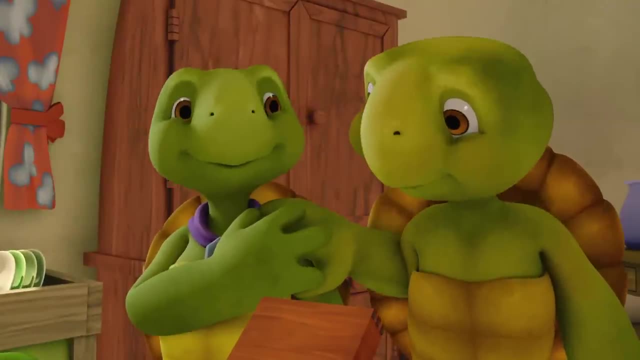 Well, when I grow up and become a real explorer, I'm definitely going to go there and find out. Wait, Did you say, if we go Mom? Yes, she did. What do you say, Franklin? Are you ready to go on an adventure? 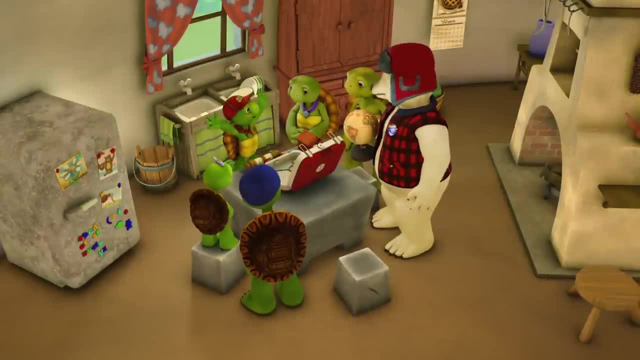 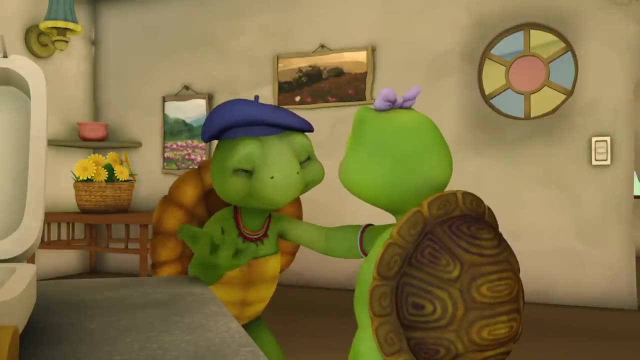 You mean it, Mom? Yes, I really am Woo-hoo. Yay, Explorer Franklin, And guess what, Harriet, We'll get to have our own woodland adventure Together, Just you and me. Yay, Explorer Harriet and Explorer Aunt T. 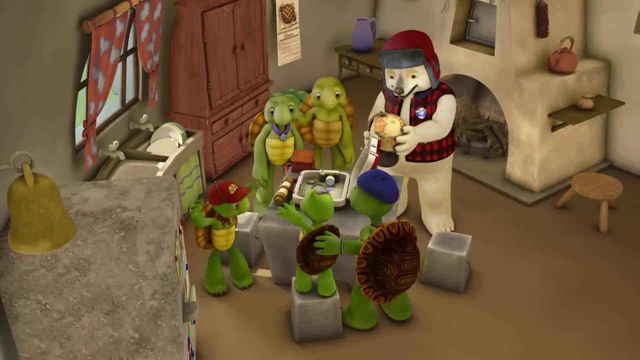 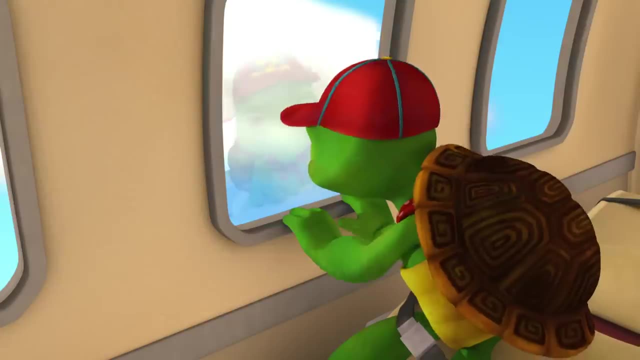 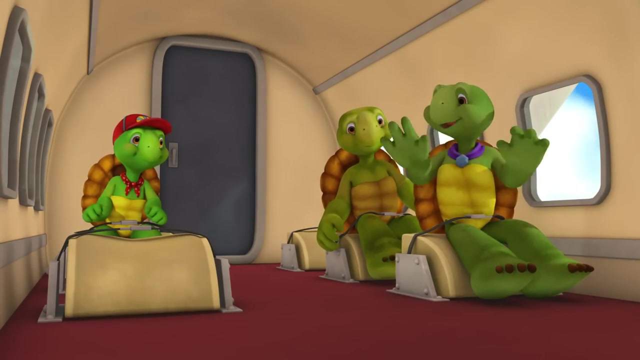 We're going on an adventure, Woo-hoo, Yeah, I've always dreamed of seeing the world, And now we're on our way. We're on our way. We're on a grand adventure. We're on our way To the ice and snow. 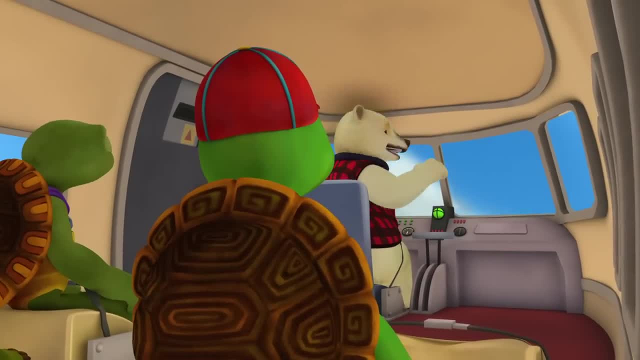 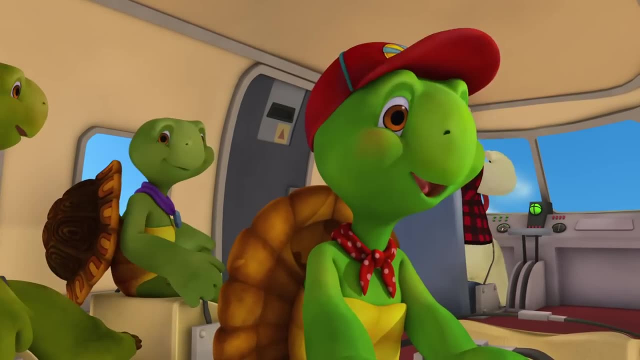 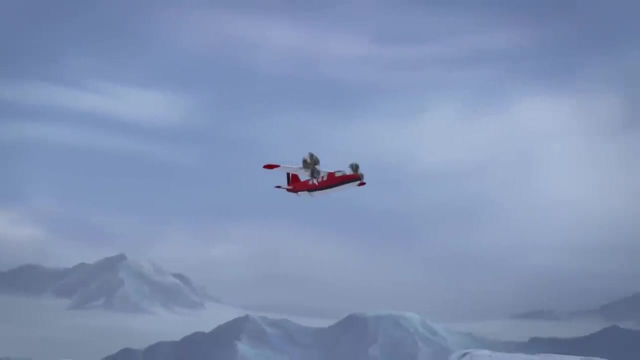 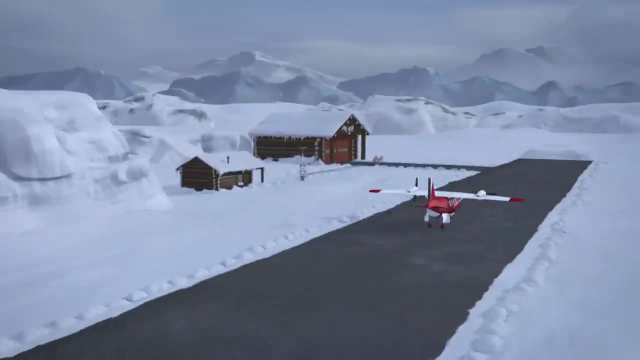 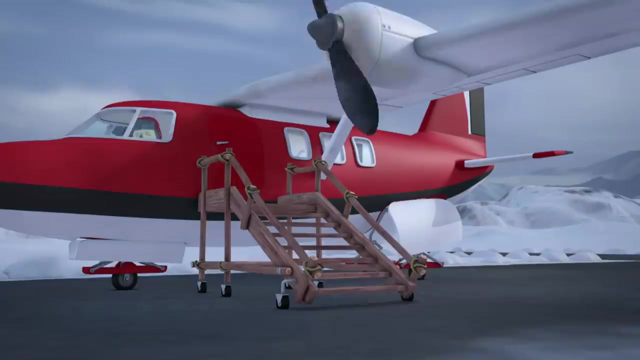 Ice and snow. I'll get you there, Just like the brave explorers. We're on our way Off, we go Off, we go, Ahh, Ahh. Welcome to my arctic home. Smell that air, Oh my God. 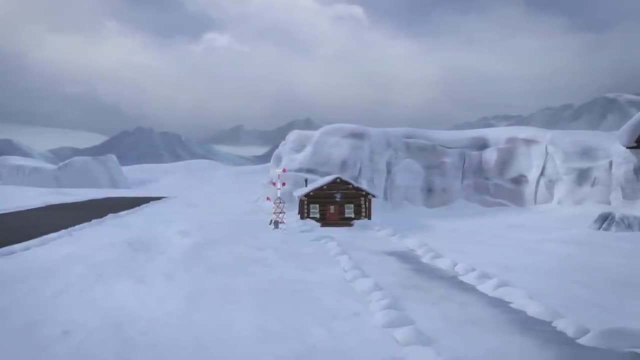 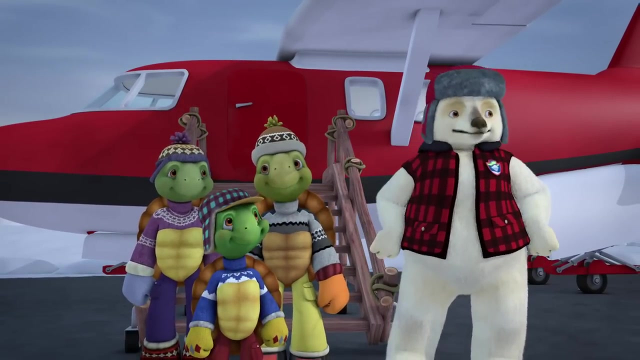 I never thought I would ever be so far away from woodland. I didn't imagine it would be so…. Harriet trekking across these ice fields, and now it'll be us. Yep, This view never gets boring. Ranger Bear, when will we see a penguin? 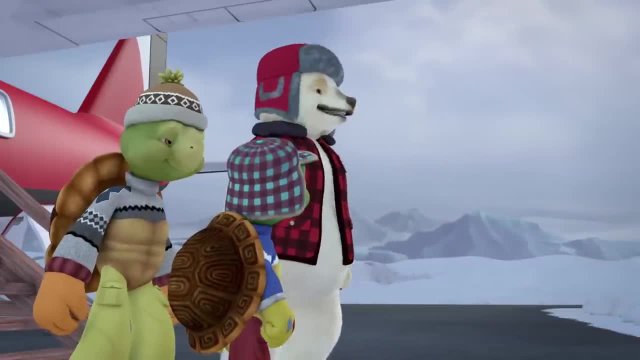 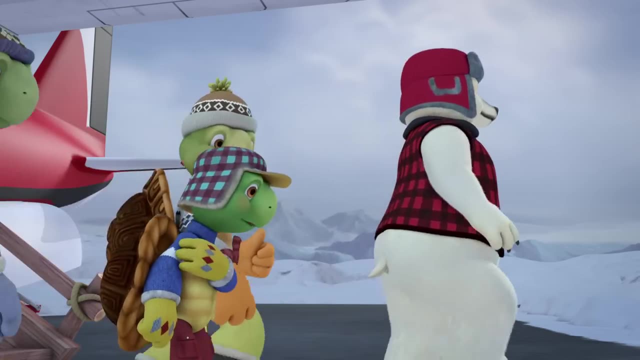 There are no penguins in the Arctic, Franklin. I'm afraid they live a very long way from here at the other end of the world. Oh, I thought there'd be penguins. Hey, are your sweaters as itchy as mine? 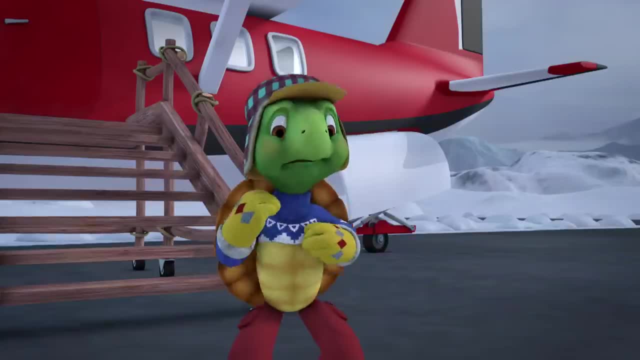 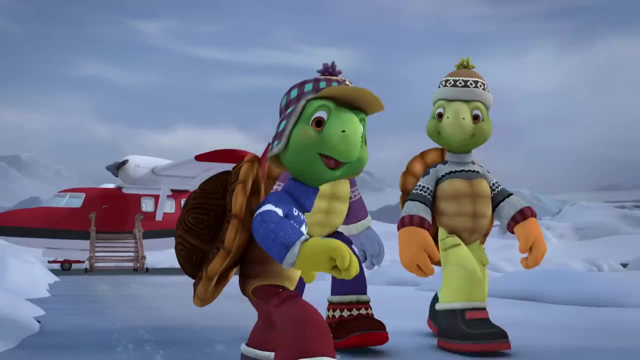 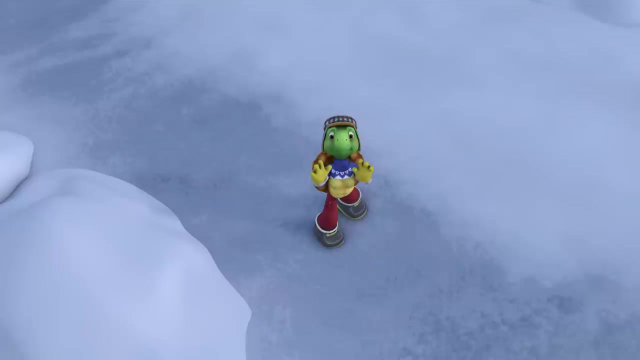 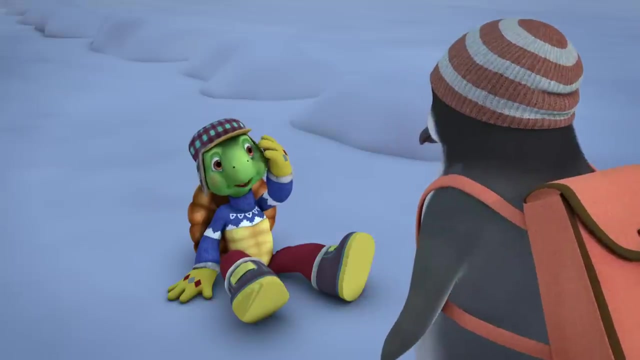 Don't worry, Franklin, You'll get used to it. Whoa Woo-hoo, Hey, coolio. Whoa Wahoo, Woo-hoo, Uh-oh, Hey, Hey, you're a penguin, Yep. 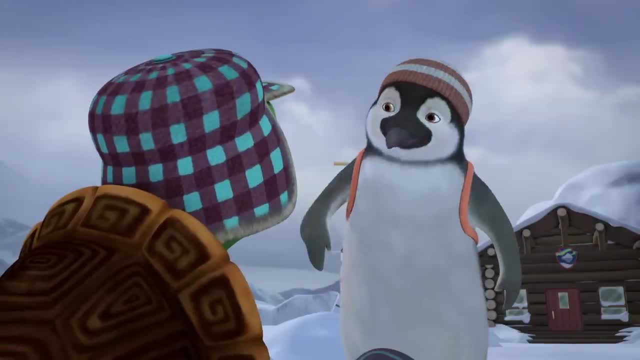 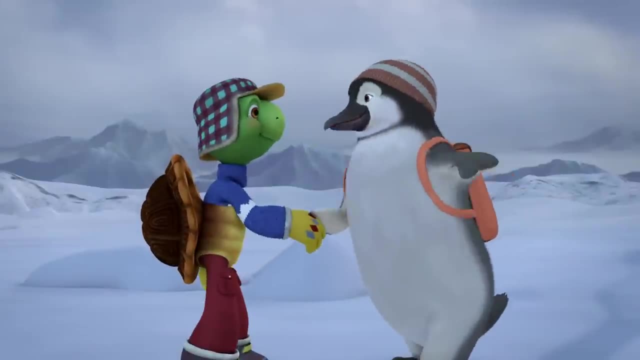 I thought there weren't any penguins in the Arctic. That's right, mate, There aren't normally. But I could say the same thing about turtles. Yeah, Yeah, you're right. Hi, I'm Franklin. Hey, name's Pip. 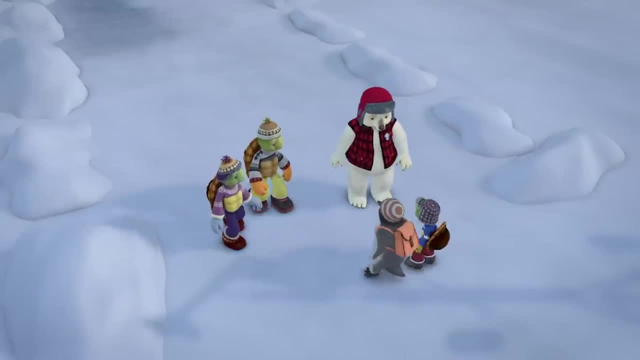 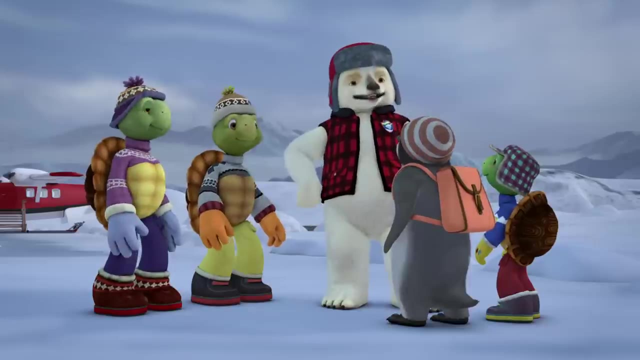 Mom, Dad, look who I met. Hello there. Well, hello, This is Pip. Hey, just passing through but thought I might hang out here for a while. Welcome, I'm Ranger Bear. Let's go inside and you can tell us how a penguin ends up on the other side of the world. 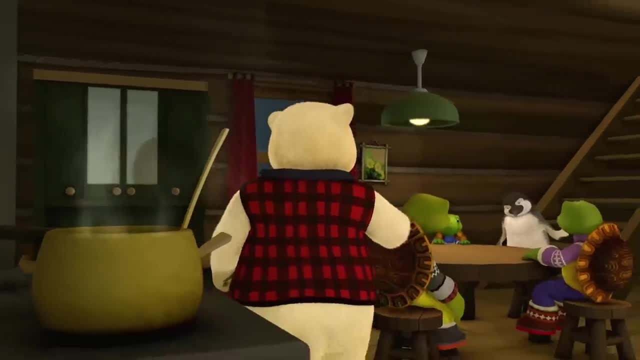 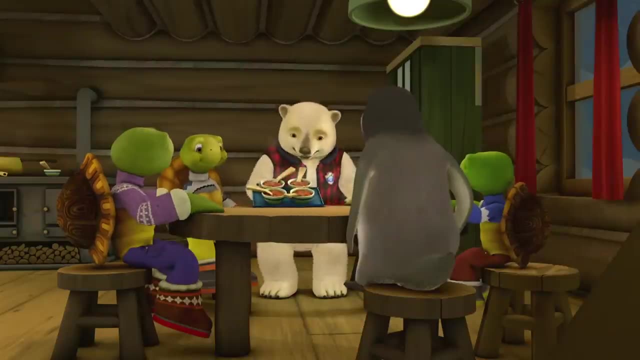 So I'm on what my family calls a penguin walkabout. We all do one when we're growing up so we can see the world and have new experiences. Sorry to interrupt, but Sorry to interrupt. but the sweet potato chili's hot. 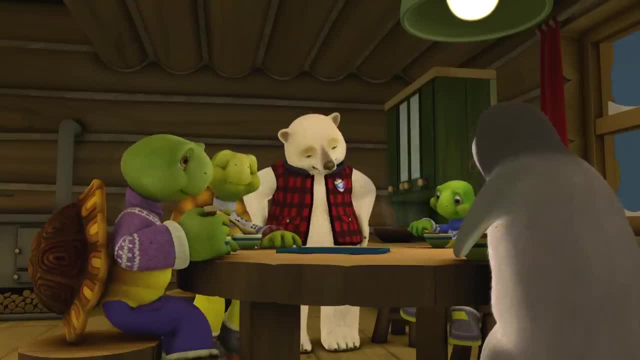 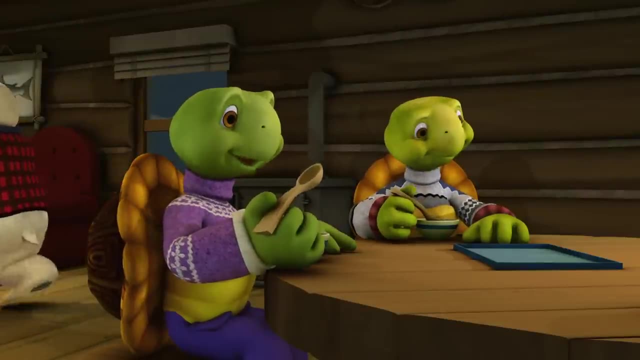 Dig in. Thank you, Thanks, Awesome, Mmm. Lovely, Very tasty. I love cooking A walkabout. you say: Uh-huh, That's quite impressive, Pip. Yep, My folks are back home in Antarctica. I've always wanted to come explore the north, so I got a lift on a passing boat. 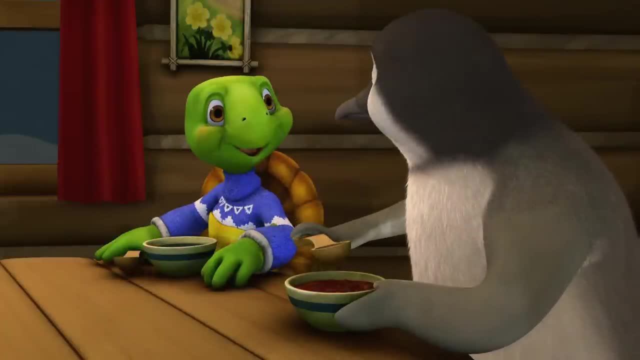 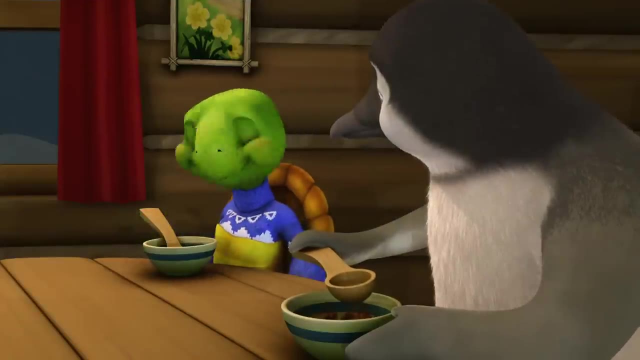 So you came here all on your own. Coolio, I want to be a real explorer too. What's it like? Pretty fun, I guess We're here on an exploration trip. I'm here on an exploration too. My great Aunt, Harriet, gave me an adventure to follow. 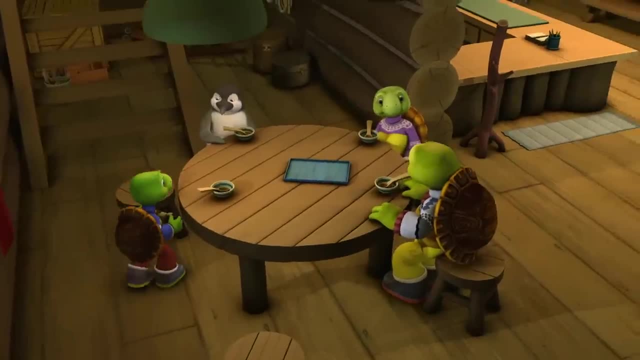 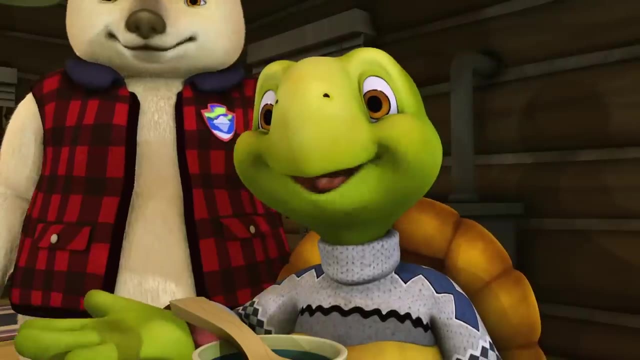 It's a real mystery. We don't even know what we're looking for. Huh, Sounds like a cool adventure. You should join us, Pip, Definitely. It'd be great to have a fellow explorer on the team. Yeah, Come with us. 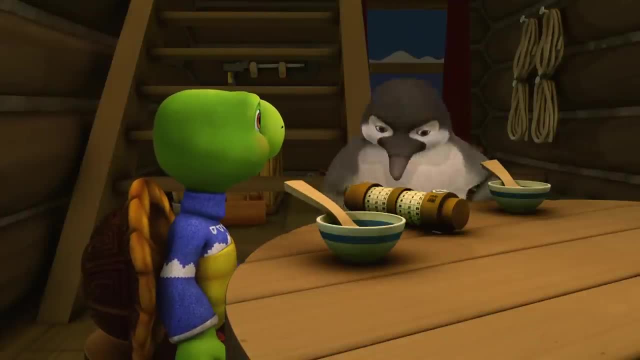 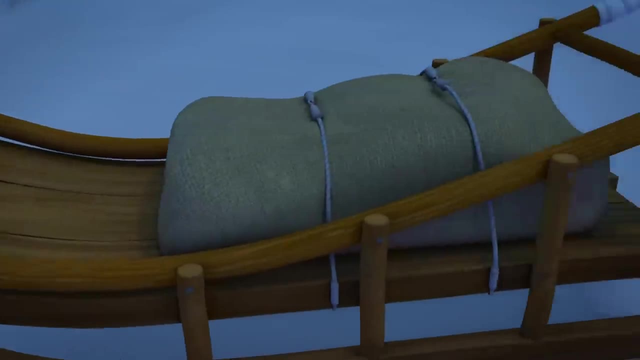 I am on a walkabout And I'm always up for an adventure. Count me in. Yay, All right. Woohoo, Franklin's right. These sweaters are itchy. Don't worry, Dad, You'll get used to it. 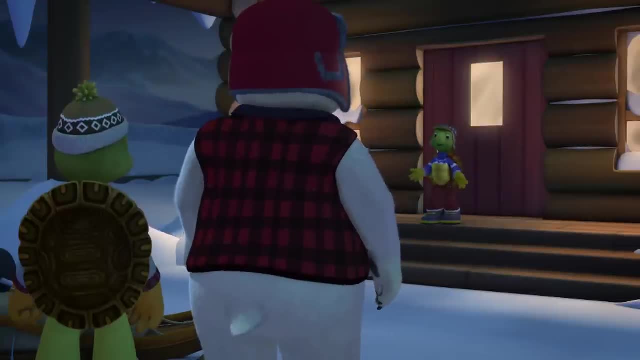 Hey, I thought we were going to leave in the morning. It's still dark out. It is morning At this time of year in the Arctic. the sun is so far away that we get only a few hours of sunlight a day, Really. 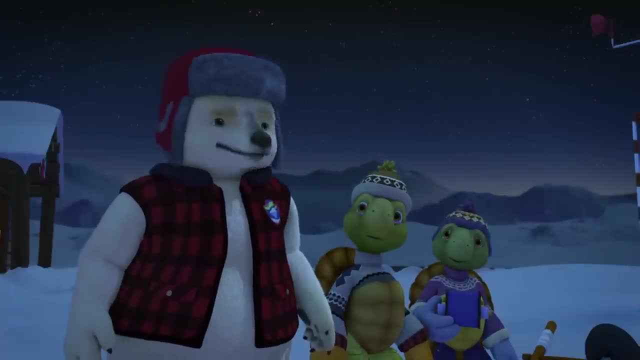 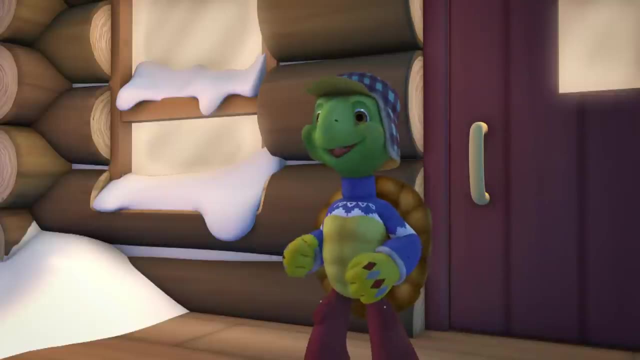 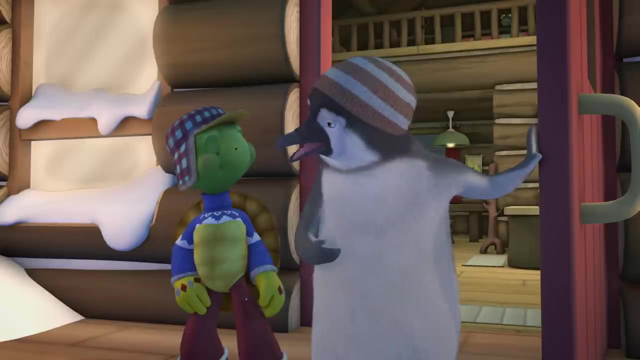 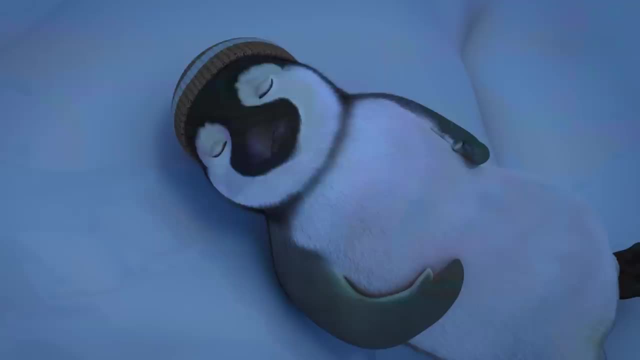 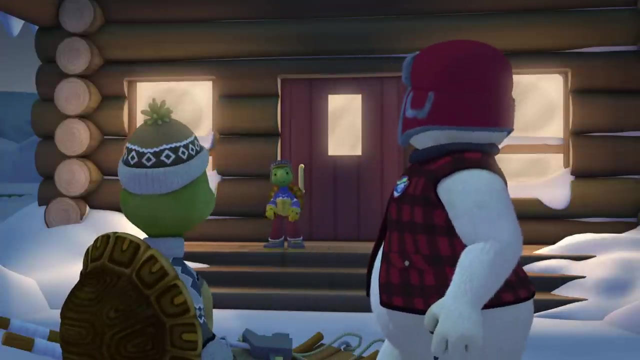 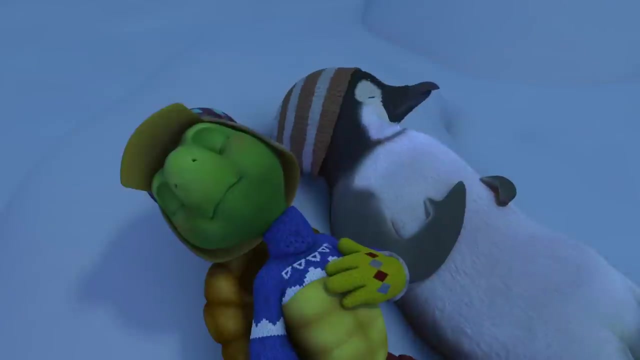 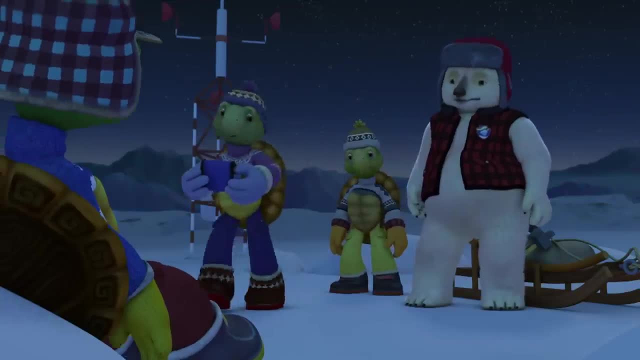 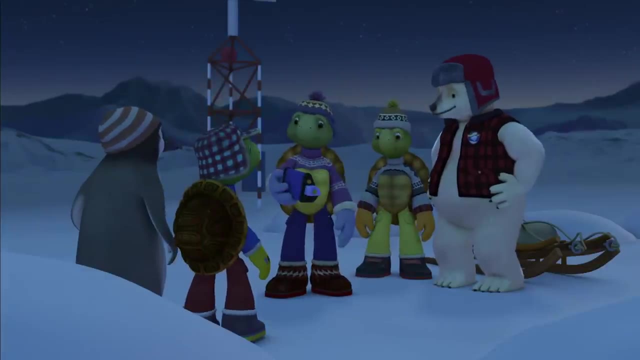 Yeah, I'm tired too. Well, you two sleepy heads, I hope you're not too tired, because we're ready to head out. Nope, No, Mr Bear lent us his GPS. All we have to do is enter the coordinates. 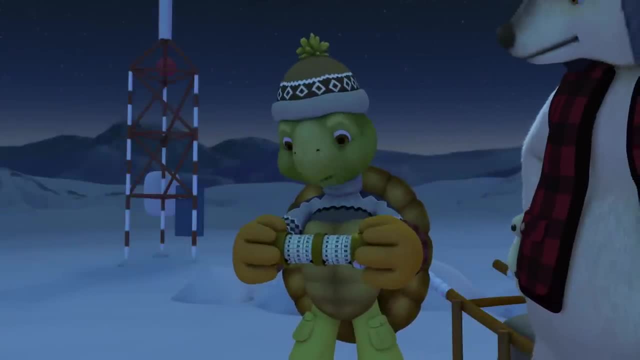 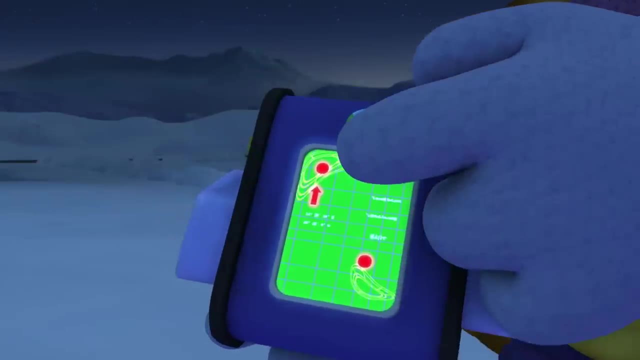 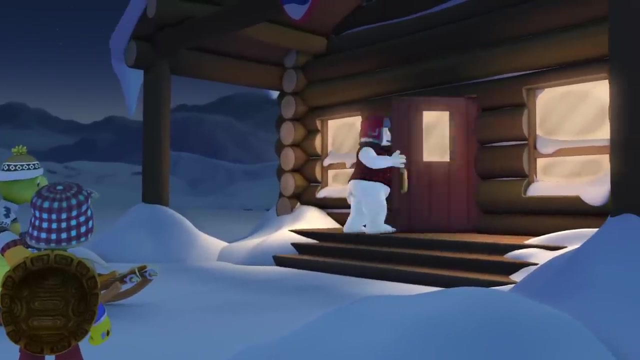 76.3 degrees north and 83.3 degrees west, And it points us in the right direction. Looks like we're headed for that cluster of ice ridges. Wow, I'll catch up with you folks later. First, I need to check the radio tower. 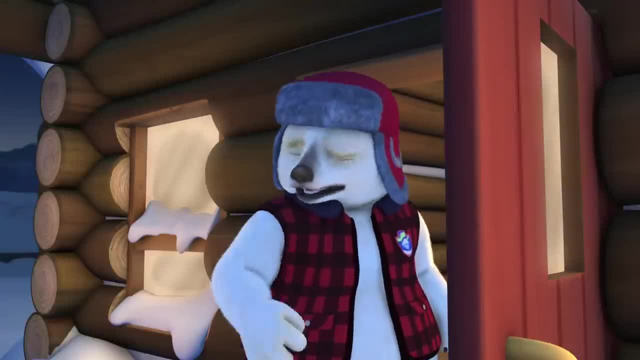 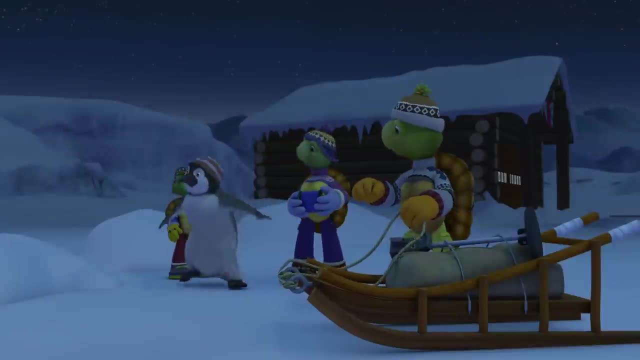 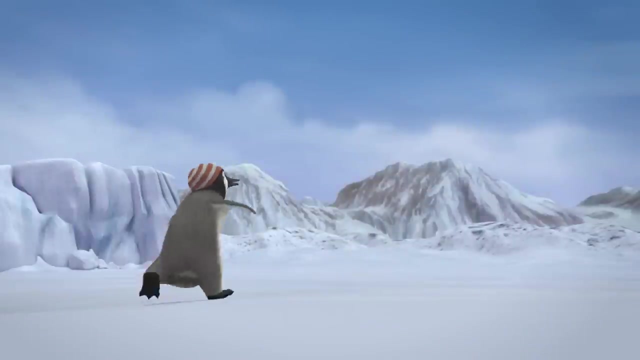 and collect a few ice samples. Have fun out there And keep me posted on the CB radio Over. They work Over. Come on, Let's do it. Woo-hoo After you, dear Woo-hoo, Let's go. 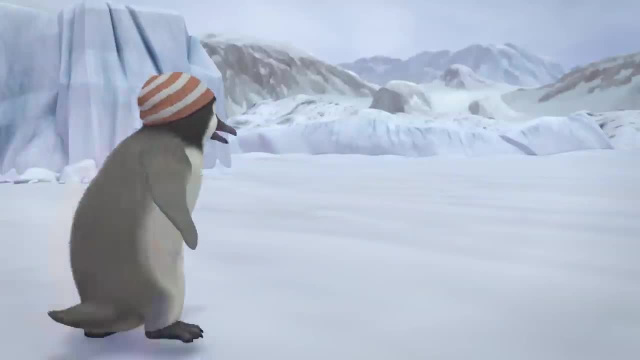 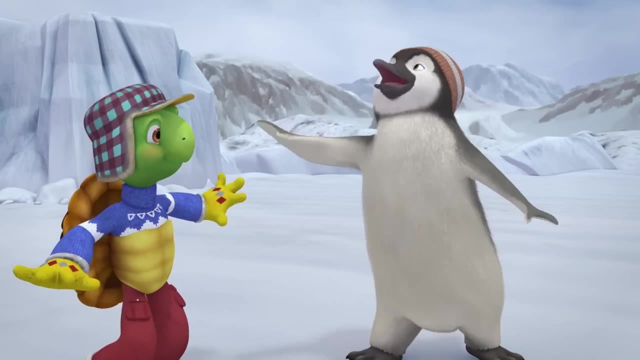 Wow, Pip, Are you always this fast? Well, actually I'm Pip the penguin, and I'm practically prone to wander the world out on my own. I seek adventure on the northern side, though the south is where we penguins reside. 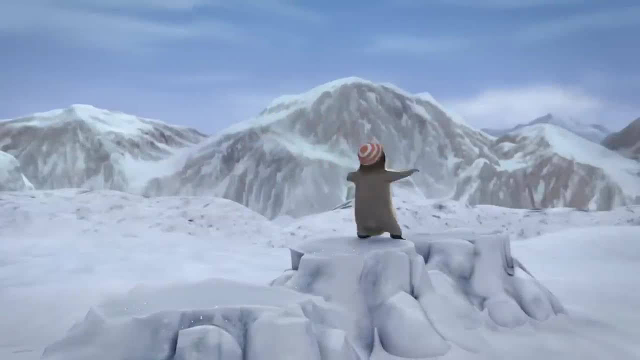 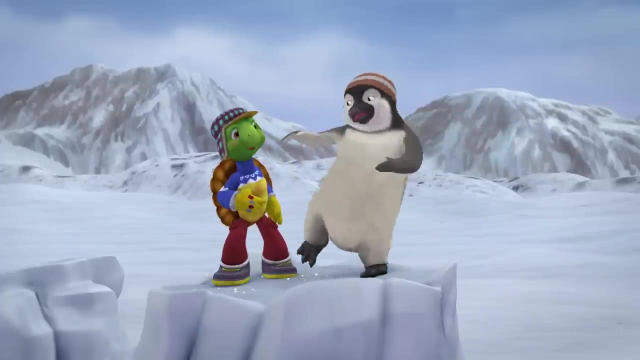 I'm on the move, You're moving, all right On the move. Hey, watch this. I'm Pip the penguin just passing through, but I love to pause and pal around with you. I love to jump and glide and slide around. 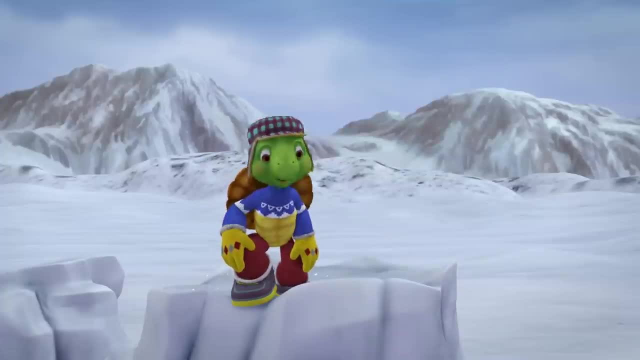 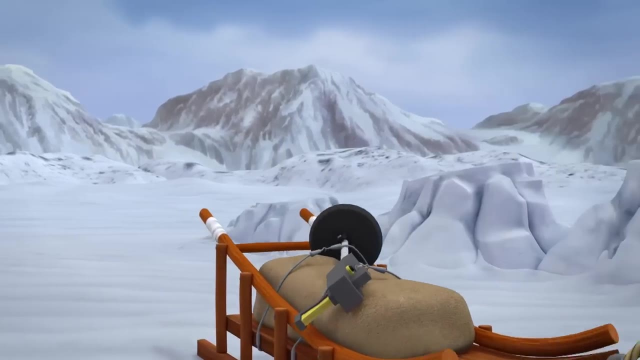 See, I'm right side up and now I'm upside down. I'm on the move. I can hardly keep up On the move, Coolio. I'm from far away from the windy pole. I go with the flow and what moves my soul. 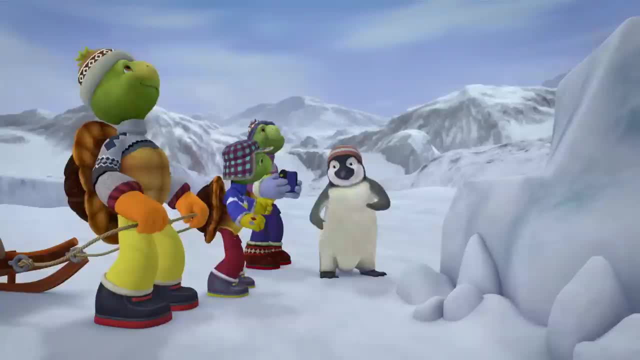 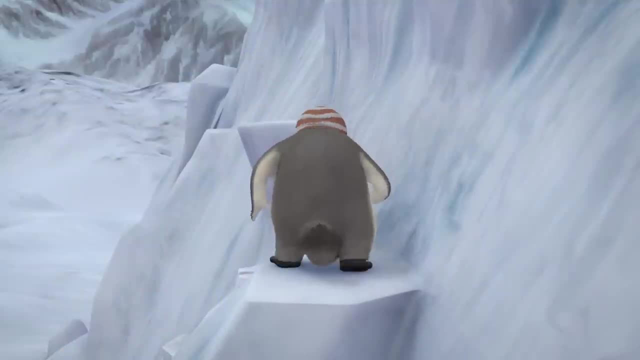 But I can see there's this thing we share, We love to explore, and it doesn't matter where. Yeah, I'm on the move, Yeah, yeah, yeah On the move, Go Pip, I'm upside down And now I'm right side up. 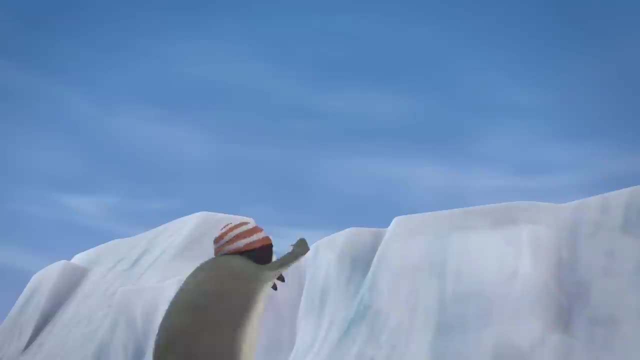 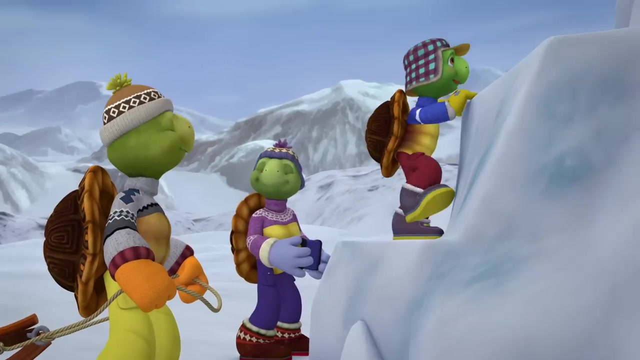 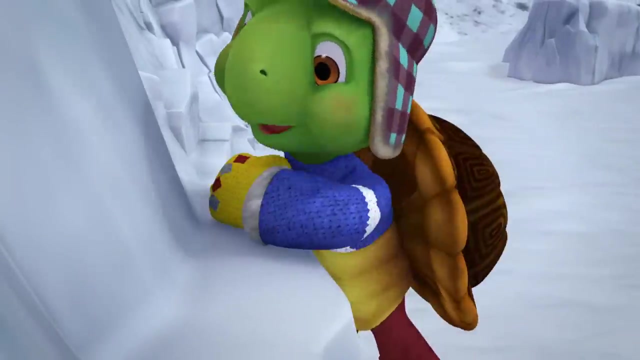 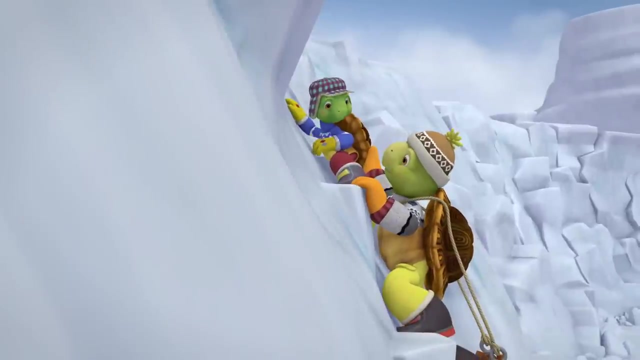 Upside down. Yeah, yeah, yeah, Yeah, Come on, let's go. Coolio, wait for me. Parkour, Careful now. Oh, take your time. Franklin Pip's made for the ice and snow. Okay, Dad. 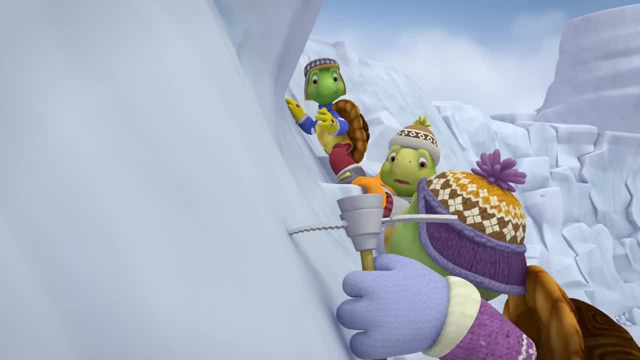 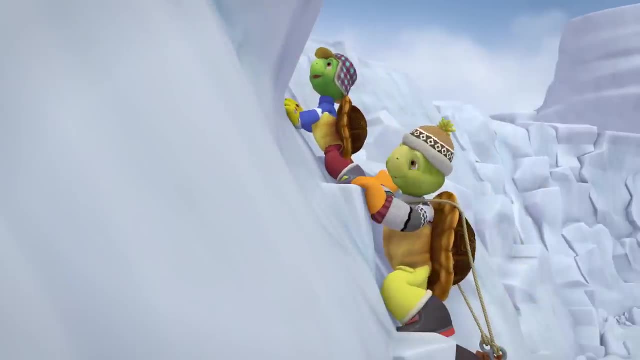 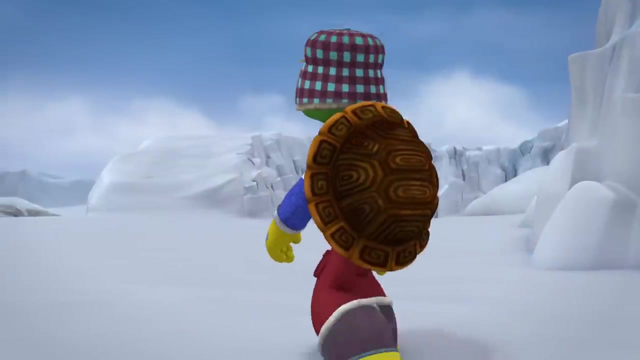 I'm just trying to keep up with him. We're getting closer. Hey Pip, see anything? Not yet Just snow. Let's look over here, Hmm, hmm, hmm, hmm. Hmm, I found something. It looks like a turtle. 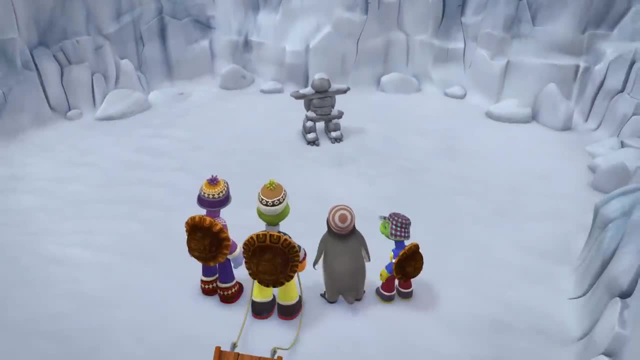 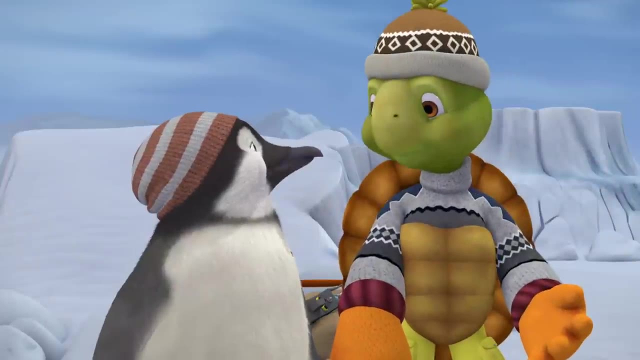 It sure is. It's made of rocks. Only Great Aunt Harriet would leave rocks in the shape of a turtle. Rocks in a pile like this are called inukshuk- Inukshuk. Well, they're used here in the north to mark important spots. 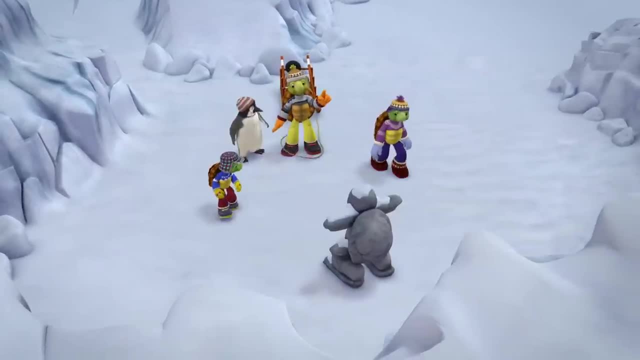 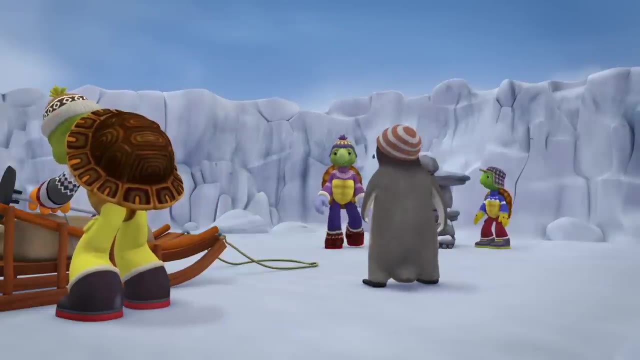 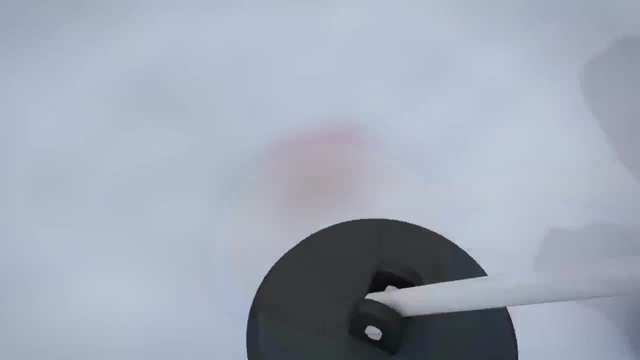 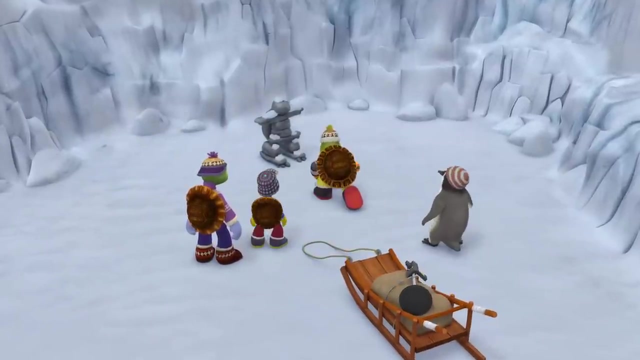 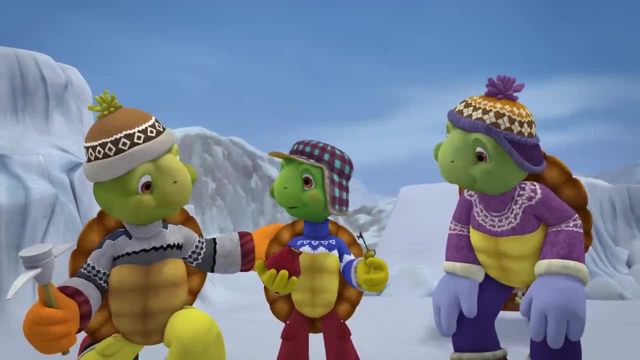 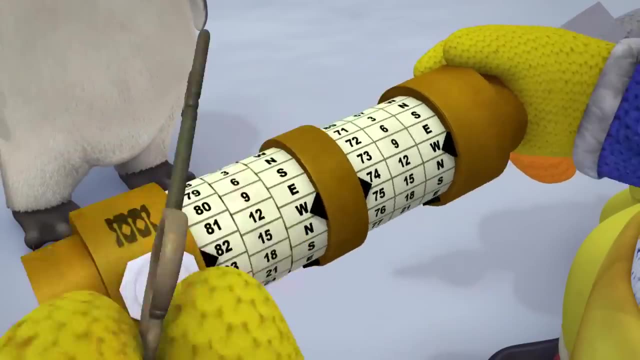 I see something. Wait, Dad, let me get it. What is it Franklin? Another key, I saw it. She did leave you a clue. Wonderful, Go for it, Franklin. Thanks, Okay, here it goes. More numbers. 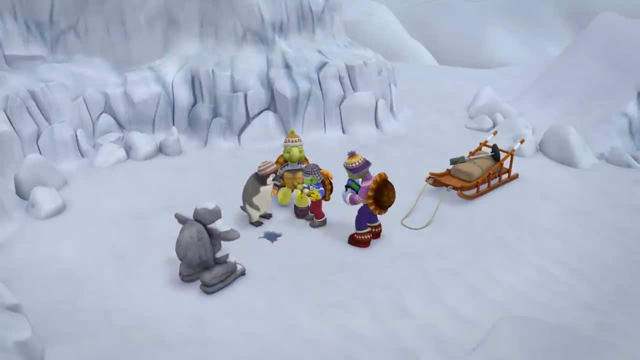 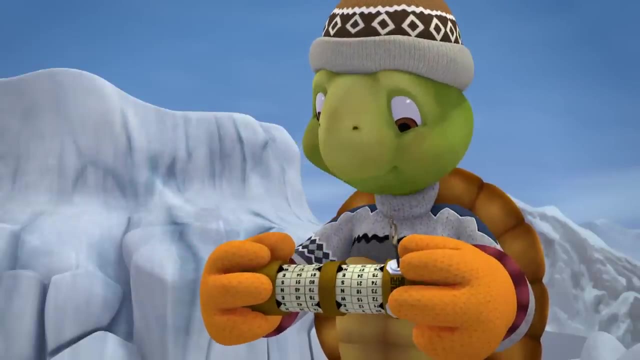 Wow, Yay, Wow, Sweet Grand Aunt Harriet wants us to go there next, right? Yup, Let's see. We're going to 76.27 degrees north and 82.57 degrees west. This is a way bigger adventure. 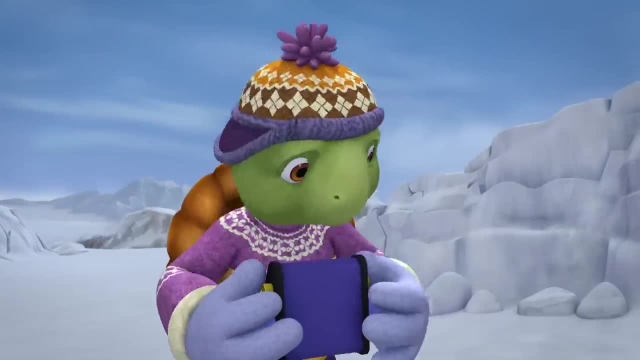 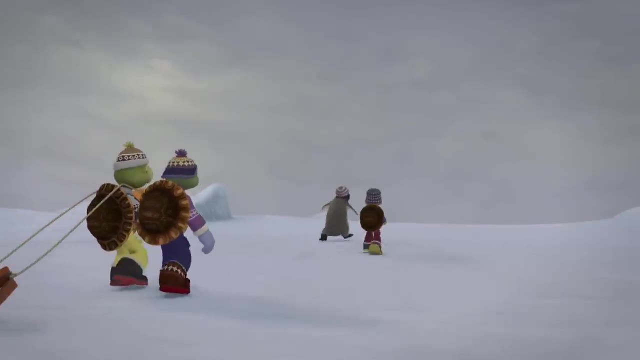 than we thought, isn't it? Okay, it's not too far We're going that way, Come on, let's go. Pip, wait up. Our next clue should be right around here somewhere. Let's go, Come on. 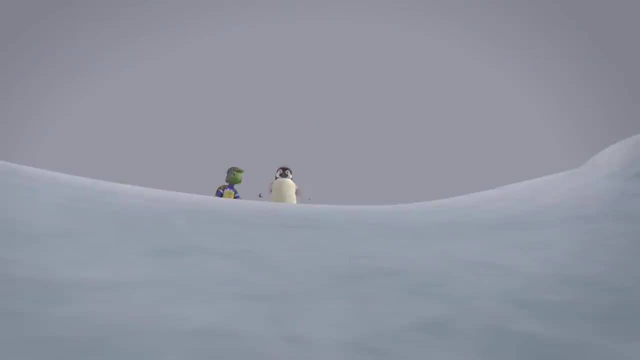 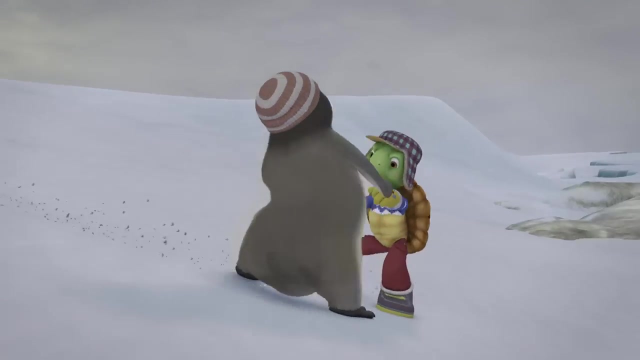 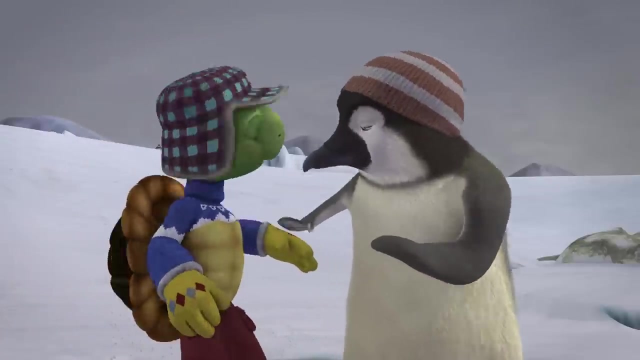 There Look. Is that it? Let's check it out. Woo-hoo, Awesome, Right behind you. Whoa, Whoa, Whoa, Whoa, Whoa. You really gotta work on your brakes. Okay, you slippery sliders. 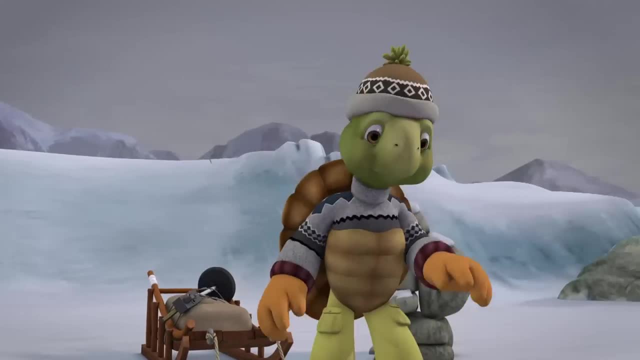 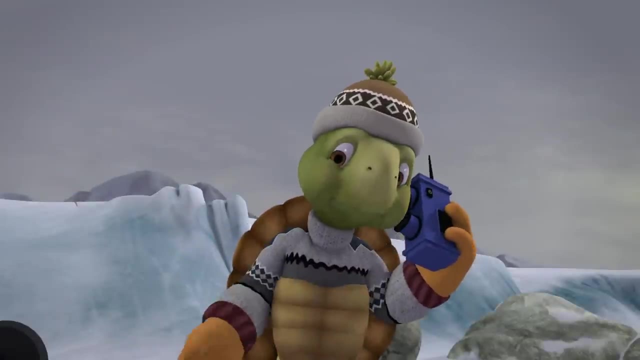 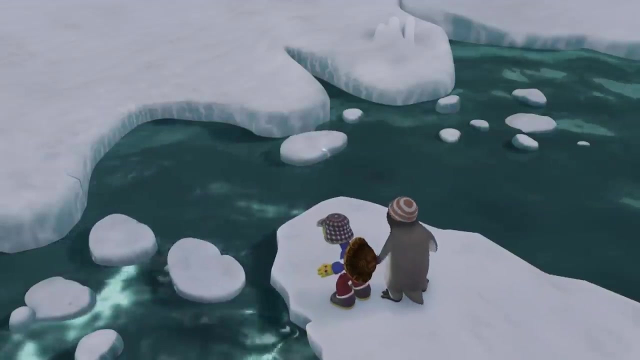 Ah, Oh, no Kids, We're floating away Everyone. I'm calling Ranger Bear. Ranger Bear, we need your help. I'm on my way. I'm tracking you with the GPS. Thanks Over, He's on his way. 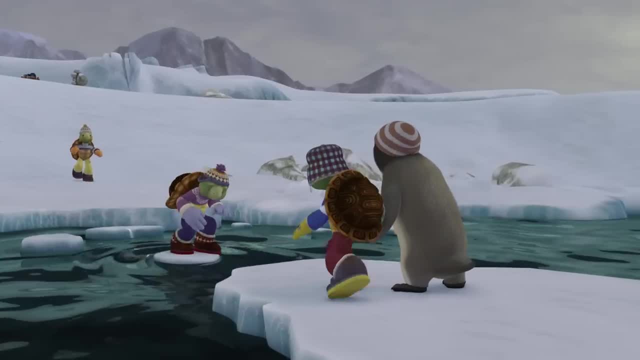 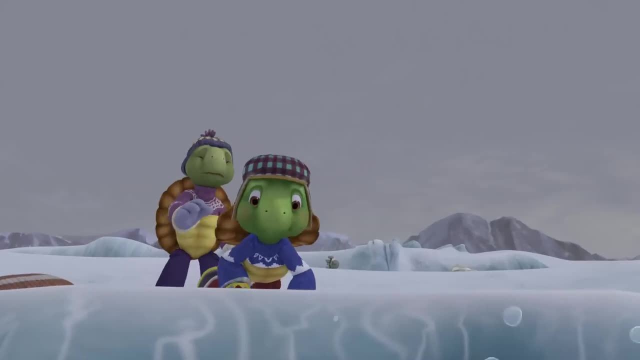 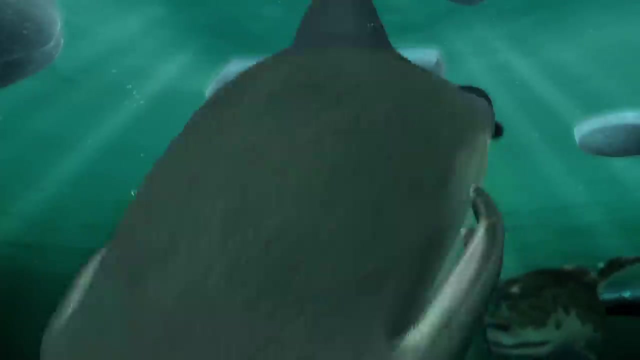 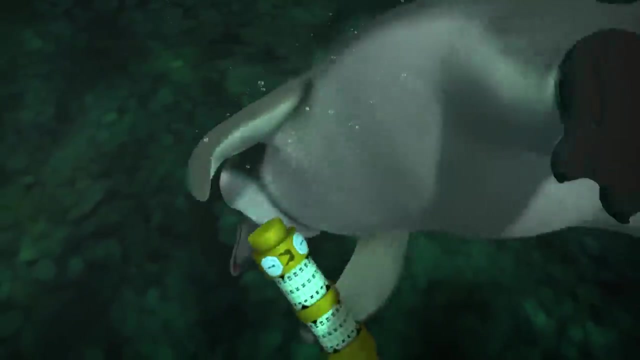 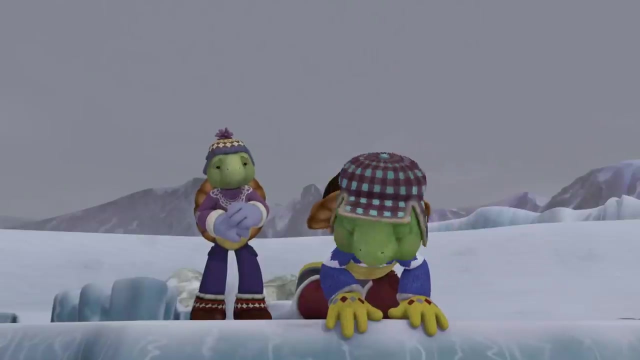 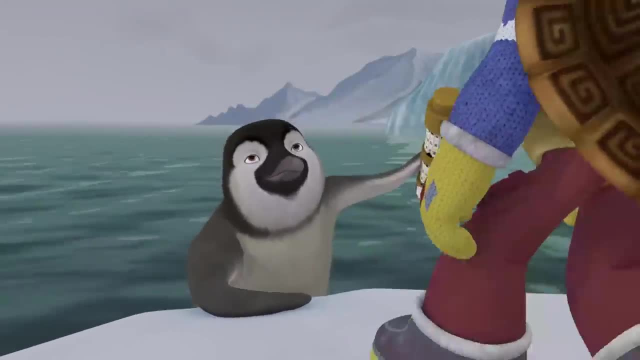 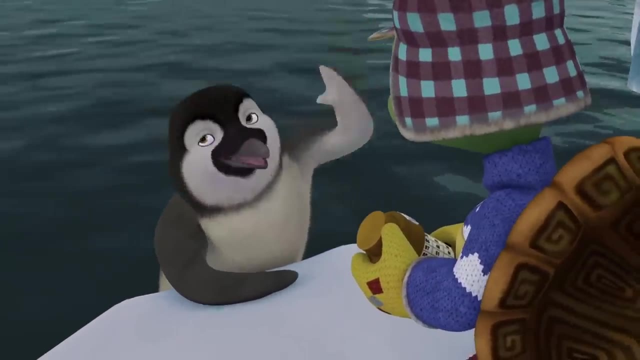 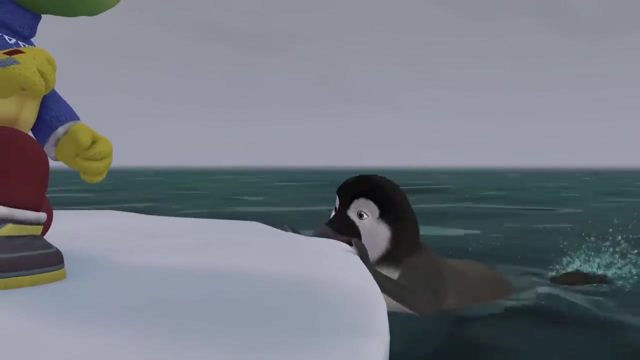 I can't see anything. Pip, Here You got it. Oh, I'm so happy you're safe. He's a huge whale with a long horn on his head- Really Everyone. okay, I'm gonna try pushing them to shore. 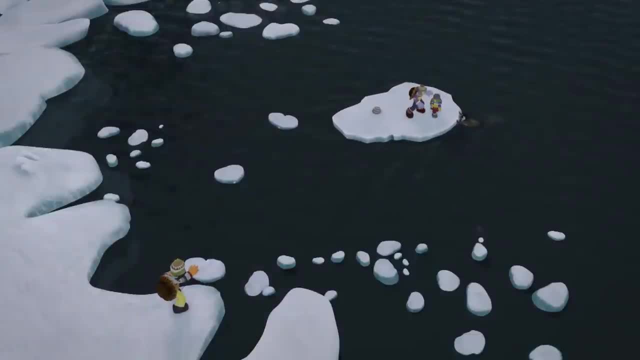 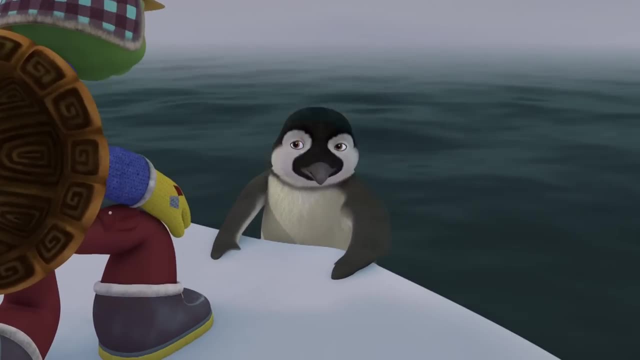 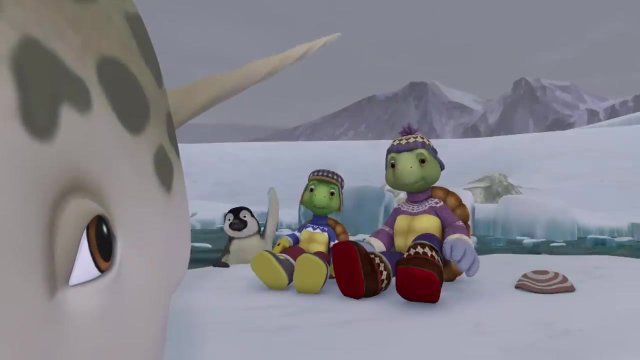 You can do it. Yeah, come on, Pip. Oh, be careful, I can't, I'm not strong enough. We'll find another way. What happened? It stopped moving, but I didn't do it. Whoa Coolio. 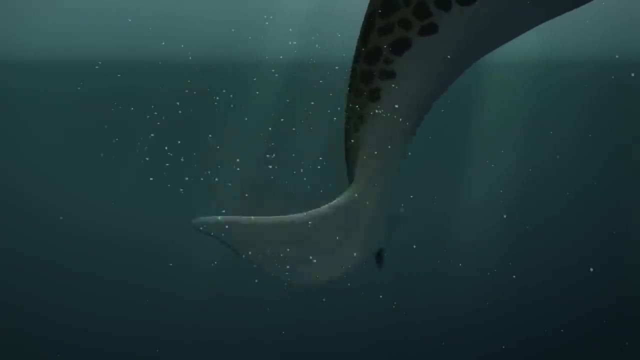 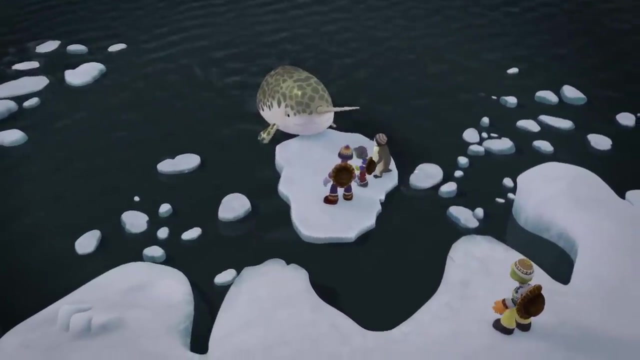 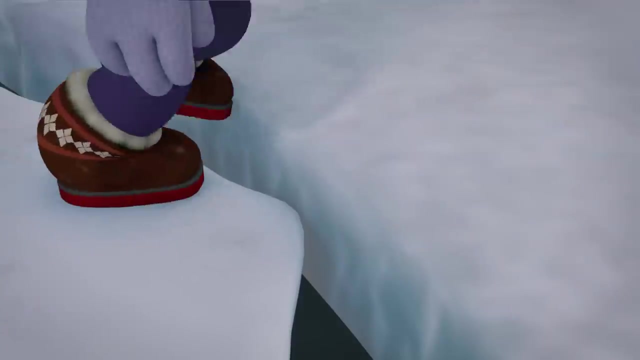 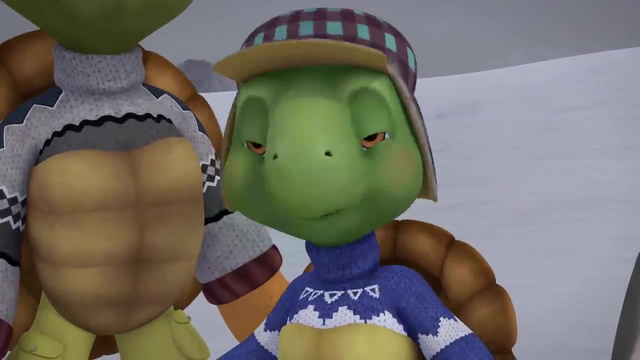 It is. What's he doing? He's pushing you back to shore. He's helping us. Come on, everybody, Careful now. Yay, Everyone, okay, You all right, boys? Yeah, Yeah, Thank you so much, Narwhal. 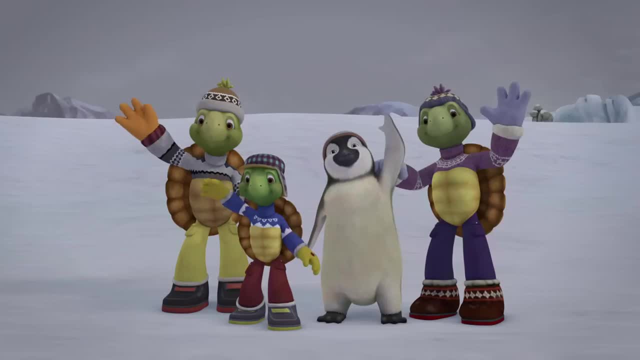 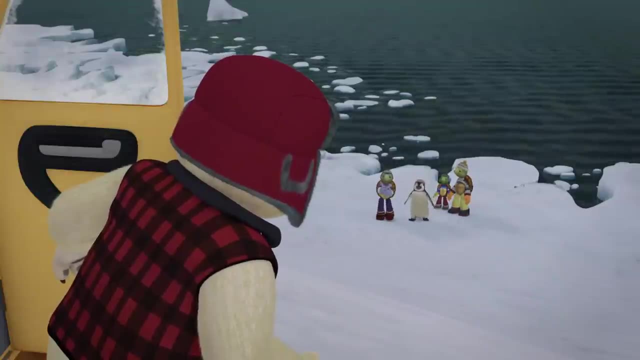 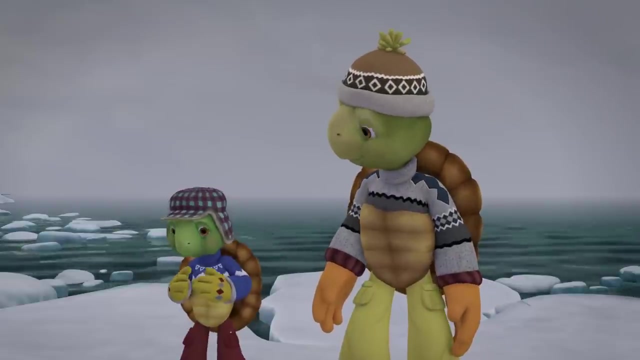 We'll never, ever, ever forget you. Bye, Yeah, Everybody. okay, You just missed some excitement, but we're still really happy to see you. Ranger Bear Cool treads. Hmm, This is some adventure, huh, son. 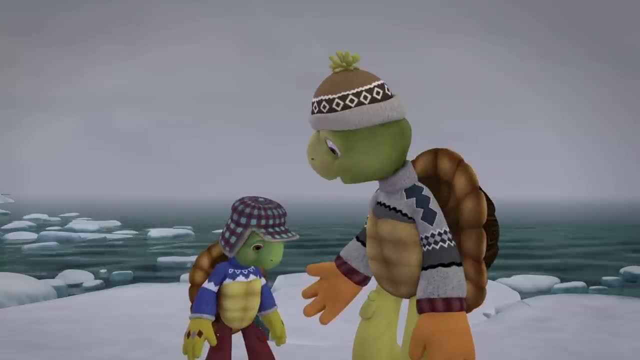 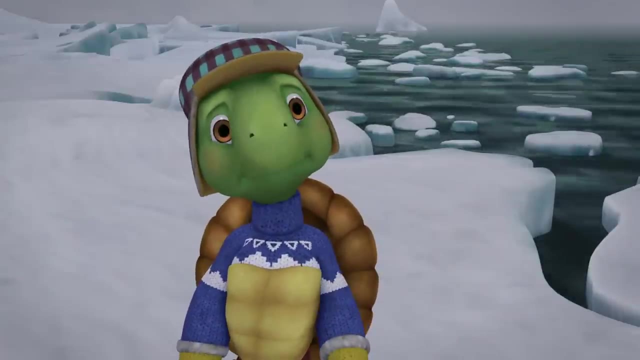 It sure is, Dad. Um, Everything all right. I guess I was just trying to keep up with Pip. Then I sort of slid further than I wanted to back there. I'll be more careful, Dad, I know you will. son. 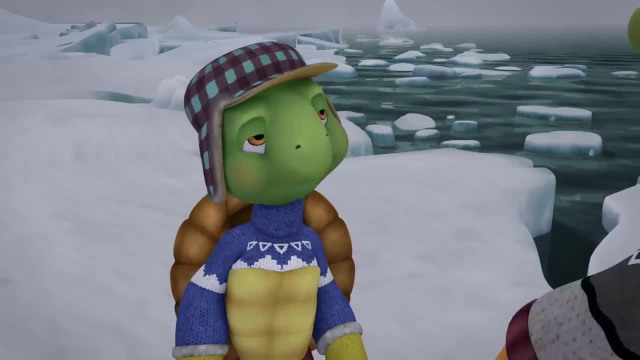 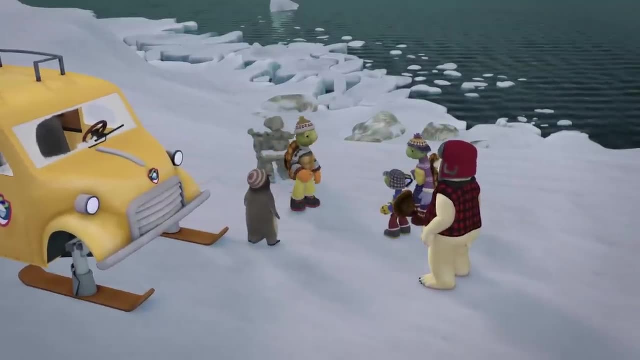 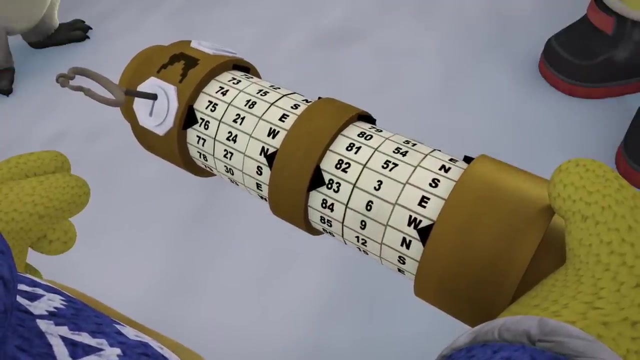 Come on, Let's go find the next clue. Okay, Here it is. Is that it, Dad Yep Franklin, The last key, Thanks. 76.24 degrees north, 83.6 degrees west. I wonder where this is. 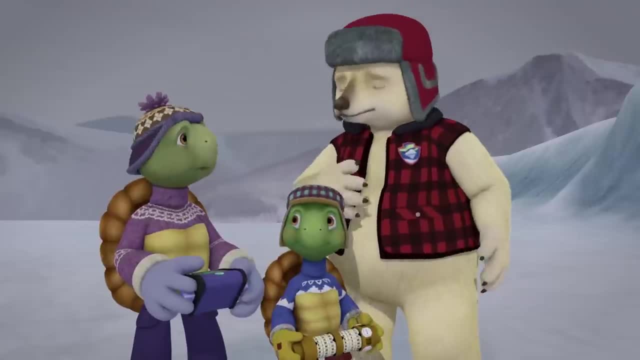 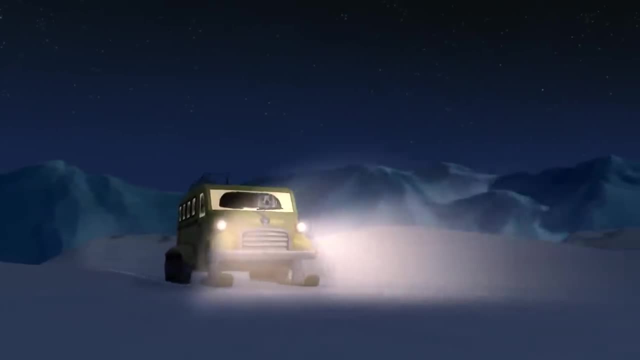 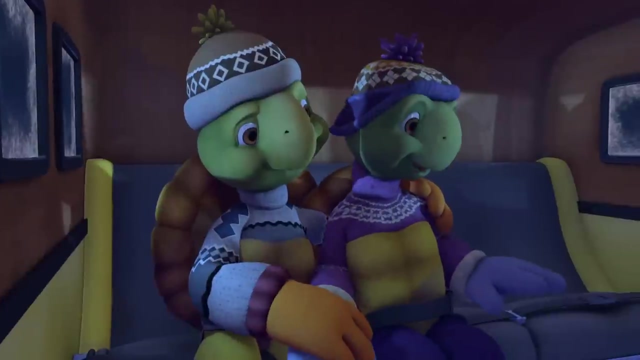 That's quite a ways away. What if I gave you all a lift? Sure, Yes, Awesome, Let's go, Let's go. I want to hold your hand dear. These sweaters are really, really itchy, That's true. 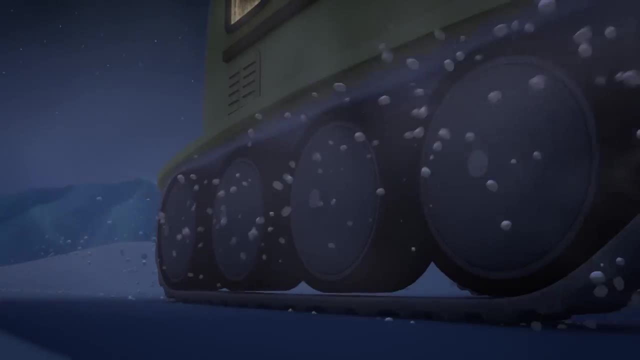 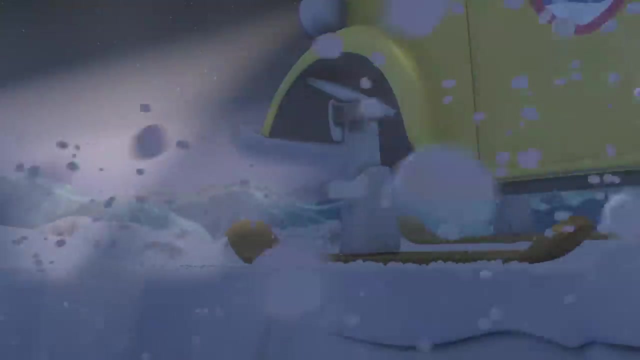 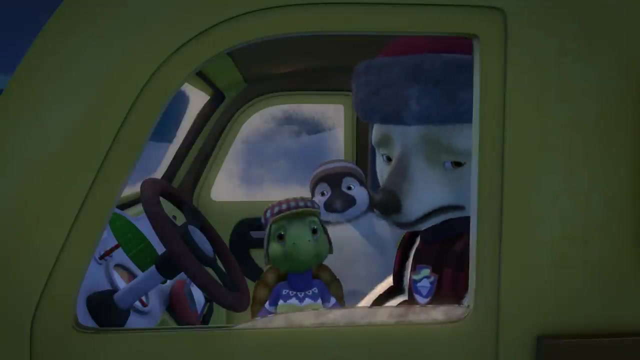 Hold on folks. Hold on folks, We gotta stop. Whoa, Everybody. okay, Yeah, That was close End of the line. That wasn't here last time I came this way I'm afraid we can't get across. 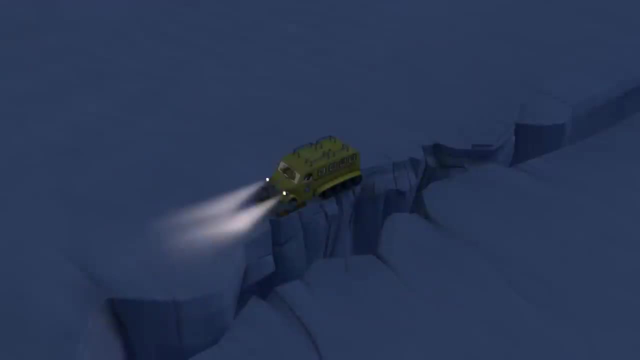 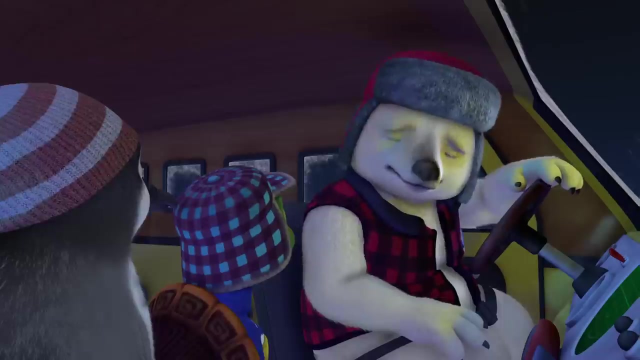 But we can't give up. now We've come so far. Maybe we could fly your plane across. I'm sorry, son, There's nowhere to land a plane on the other side, But by gosh flying is a great idea, Franklin. 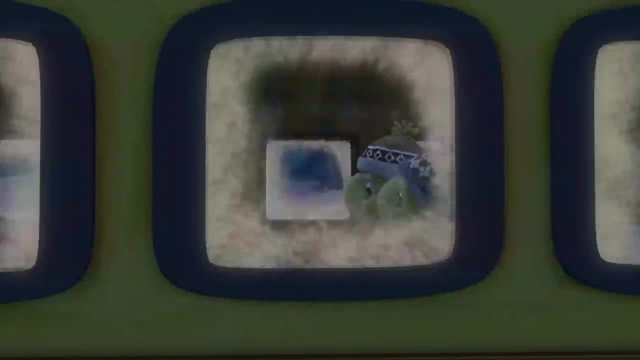 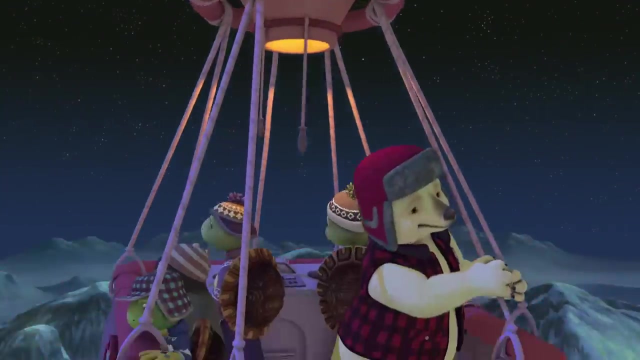 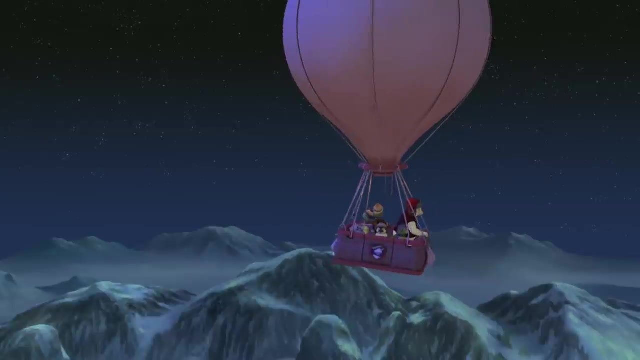 It is. Come on, let's buckle up And up we go Going up above Fantastic And we're off. Here we go. Yeah, I use this as a weather balloon to track changes in the temperature high above us Epic. 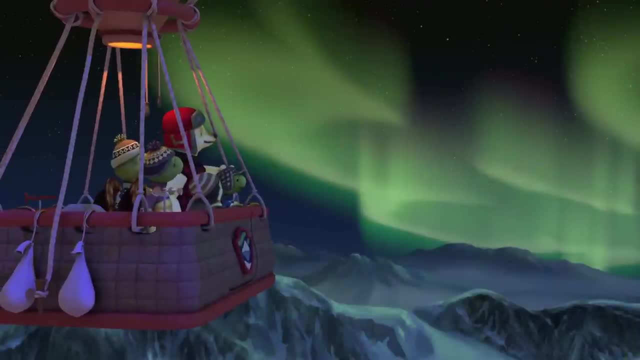 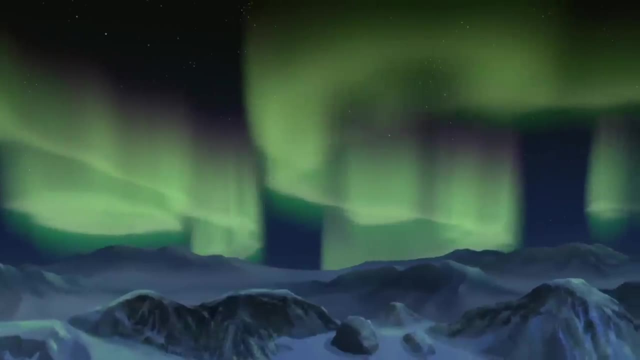 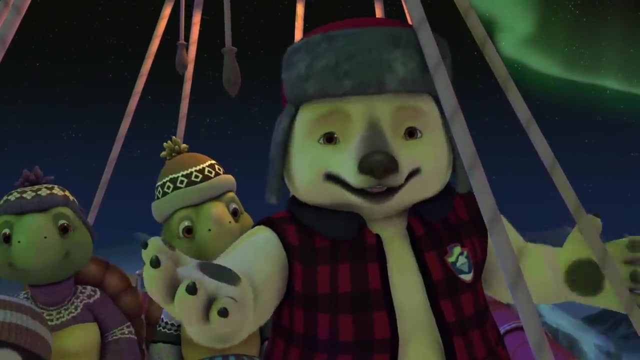 Terrific, Whoa, Everyone. look What is that? The aurora borealis. Wow, Sometimes called the northern lights. How beautiful, Amazing, Yep, it's quite a sight. What makes all the colors? Well, when the solar wind meets the air way up high, sometimes the air starts to glow. 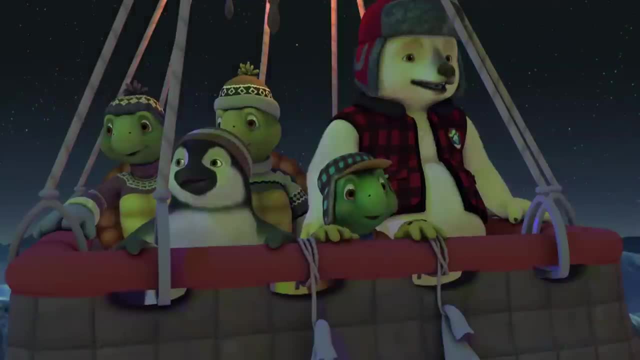 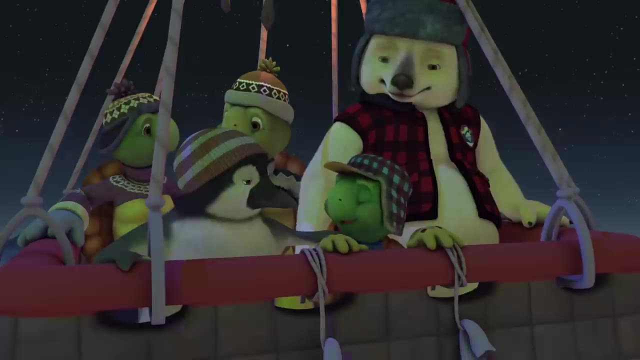 It's amazing. It's like curtains of light. It reminds me of home. Franklin, remember when we met and you asked me what it's like to be an explorer. Uh-huh, Well, I think this is what it's like. 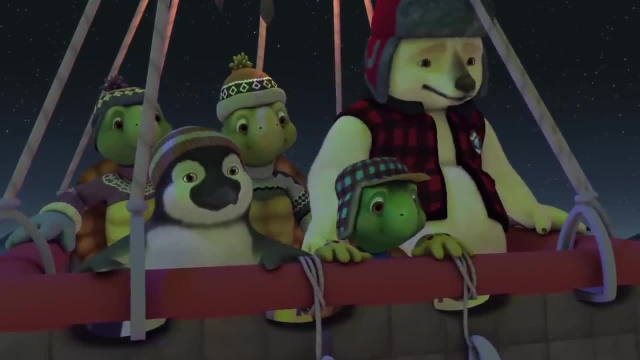 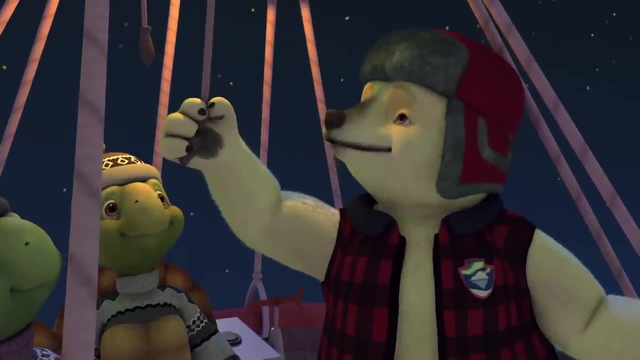 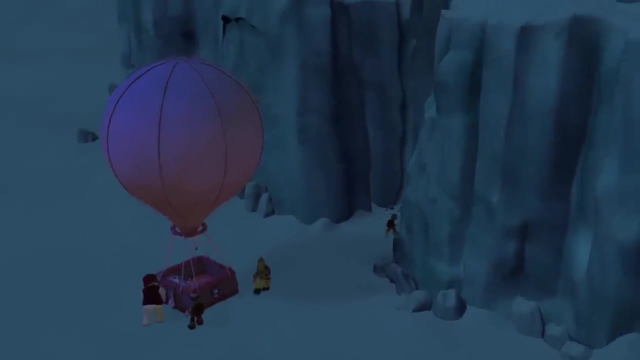 Yeah, I think you're right. Oh, It must be down in that canyon. Prepare to land folks. Go ahead, son, we'll catch up, But be careful, Let's go, Franklin. Hold on Pip, Come on. it's this way. 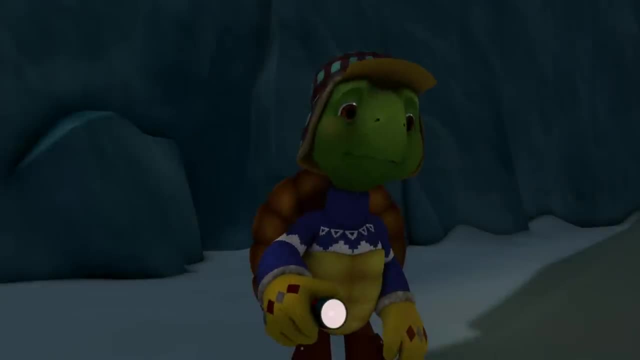 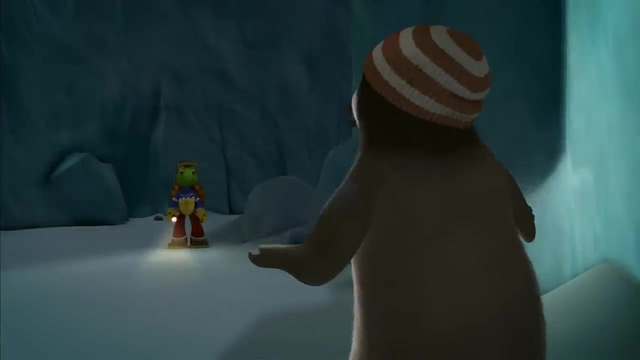 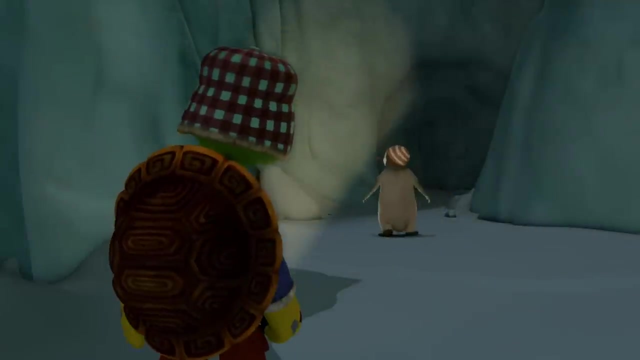 Um, Okay, Franklin, I can't wait to see what your great-aunt Harriet has waiting for you. Um, Maybe we should wait for the others. Nah, they'll catch up. You can go ahead. I want to follow you. 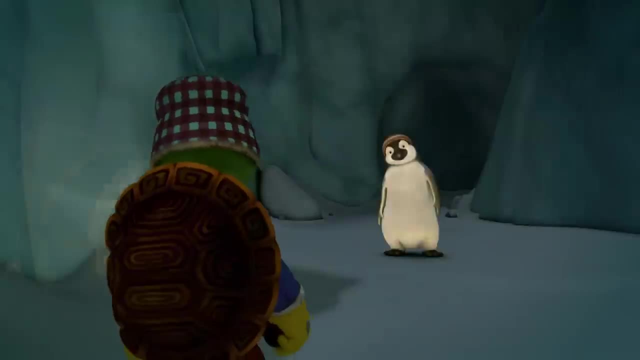 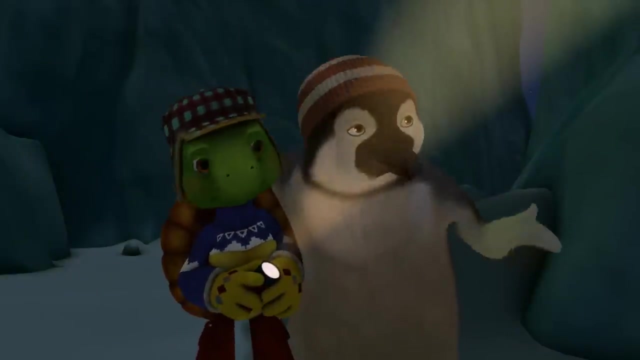 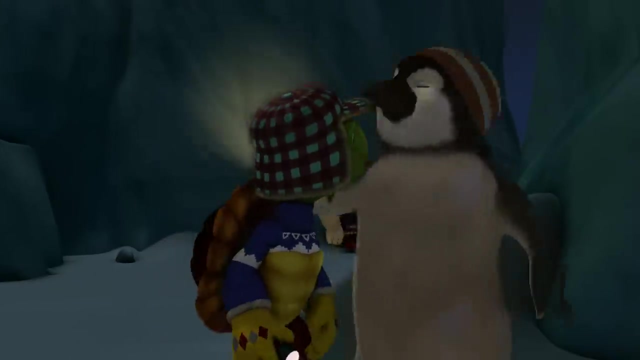 but I'm a little scared. I'm going to wait for my parents. Well then, Let's wait. We're doing this together. Franklin, That's just the wind. We can handle that. Right mate, Right Franklin. there you are. 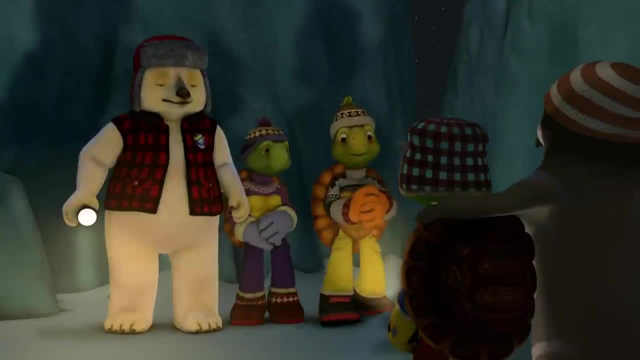 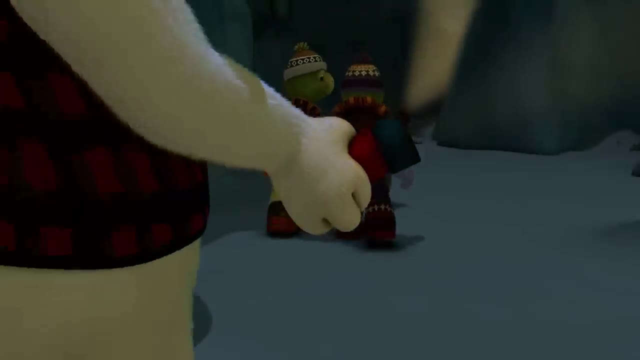 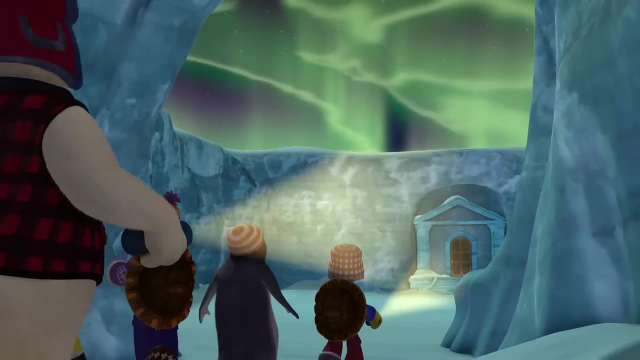 Did you find anything yet? Not yet. We wanted to wait for you. Great, Why don't you lead the way, son? Okay, This way, everyone, But be careful, It's dark in here. Whoa Awesome, Isn't this something? 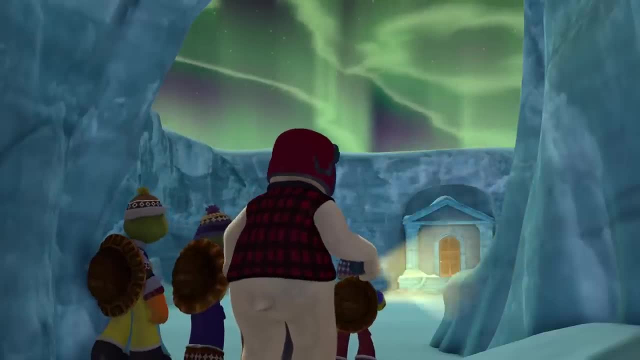 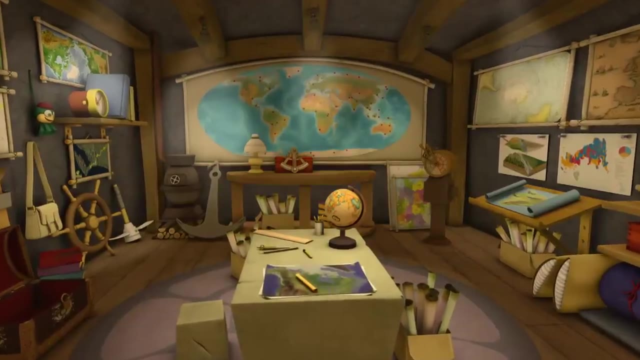 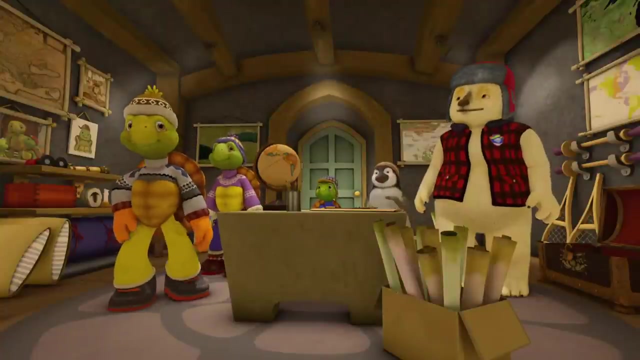 Look, There's a door. Wow, Maybe I can shed a little light on this situation. Great-aunt Harriet's map room- Wow, Look at all these maps. Amazing, Isn't that something? She sure has been to a lot of places. 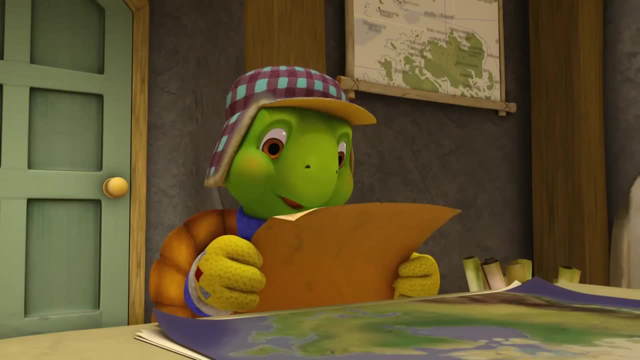 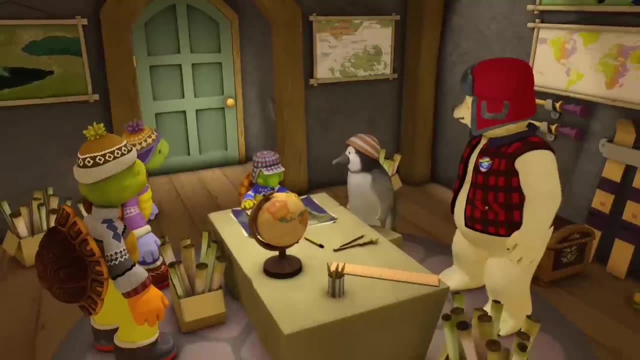 Maybe this is where she kept the record of all the places she traveled. We're going to the end of Great-aunt Harriet's adventure. That's it. We did it. This is what she wanted me to find: More adventures, You're right. 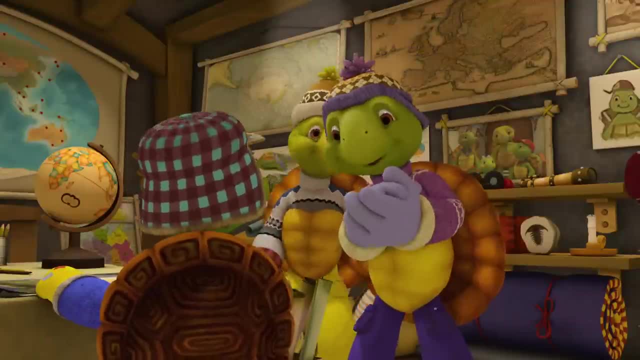 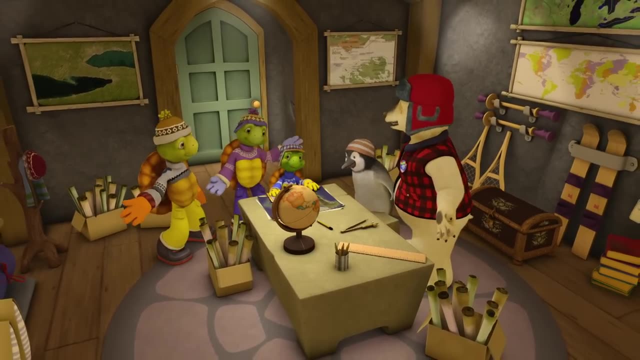 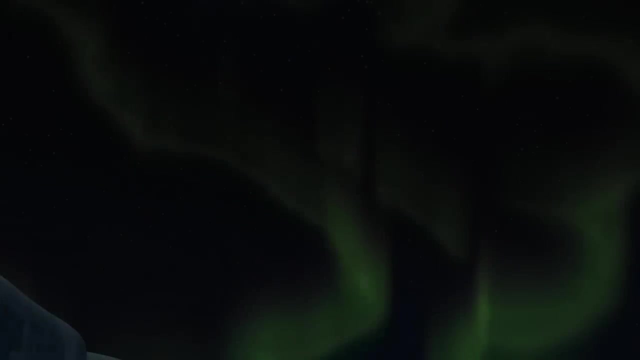 Nice job, son Coolio. Well done. Congratulations, son, We did it. We found our way, Just like the brave explorers, We found our way through ice and snow. Whoo Yeah, Hey, Pip, check it out. 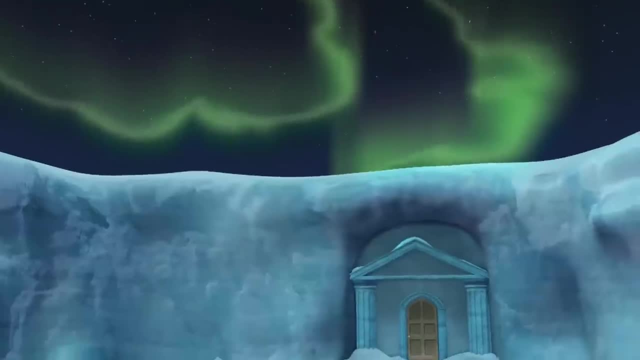 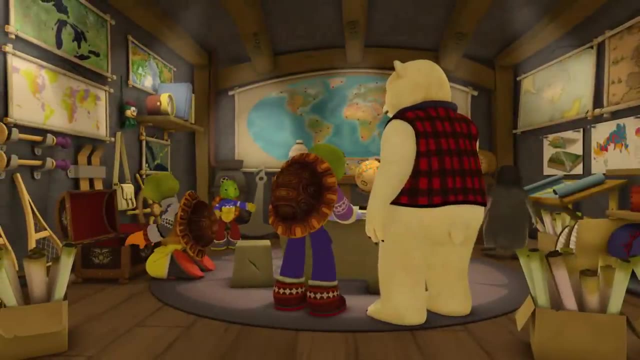 It's over here. I've never seen so many maps. This one looks super old. I can't believe we found Great-aunt Harriet's map room. The key she gave me really did lead us on a great adventure. We had the best time. 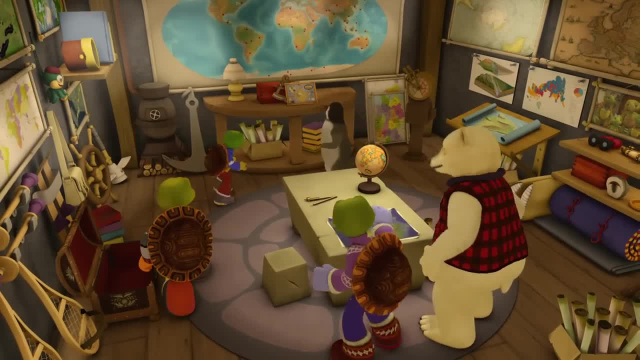 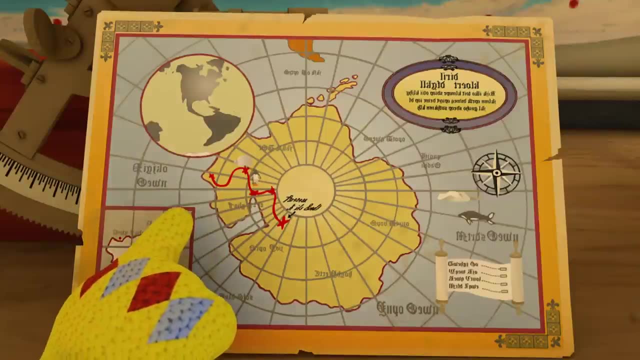 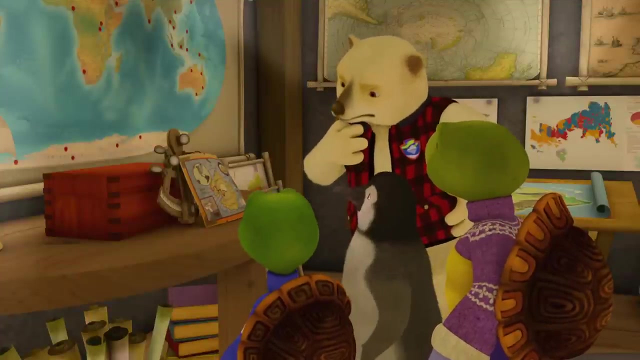 Hey, I found a map of where I live in Antarctica. Let me see. Here's where I grew up, Really. Let's have a look. I wonder what the big red X is for. There's some writing there, but I can't make it out. 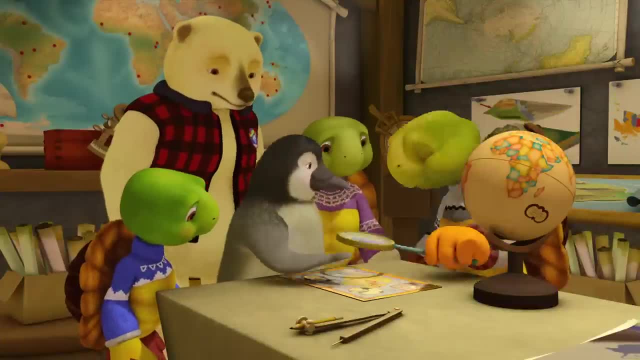 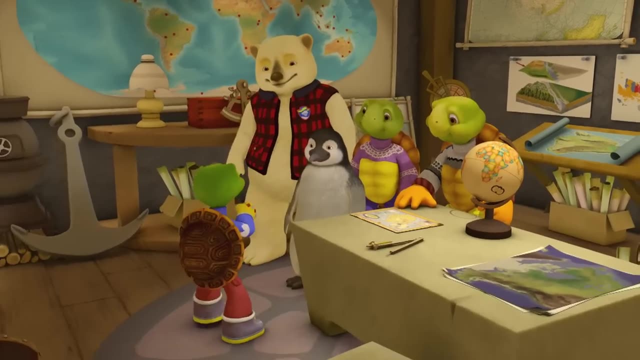 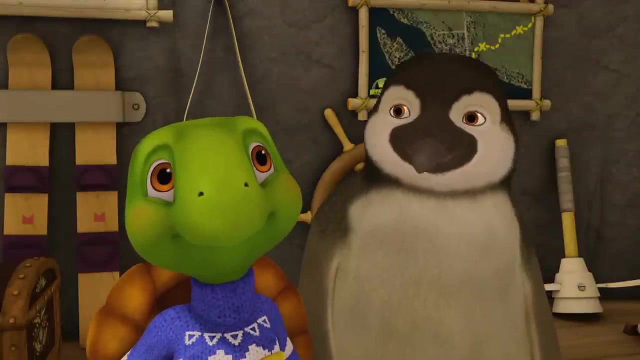 Let's take a closer look. Hmm, It says Treasure of the South Treasure. Maybe it's old dinosaur bones Or pirate treasure. Well, it could be anything. Remember Franklin? Great-aunt Harriet sometimes calls you her Treasure of Woodland. 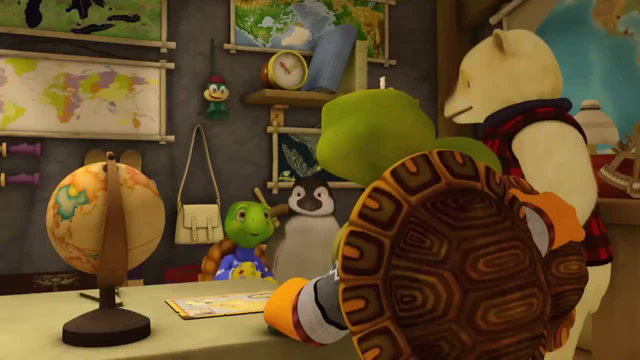 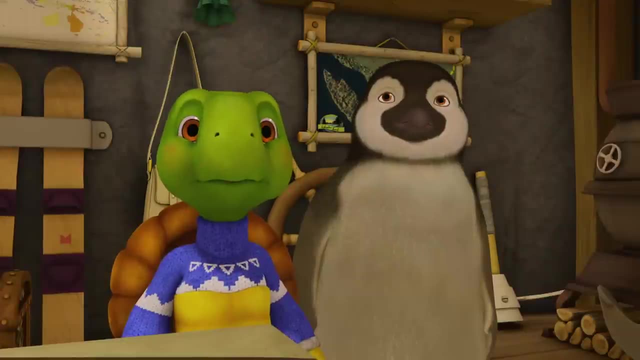 So all we can really be sure of is that she's a real treasure. Maybe we could follow this map and find out what it is. That would be incredible, Franklin, but Antarctica is very far away. It's the other side of the world. 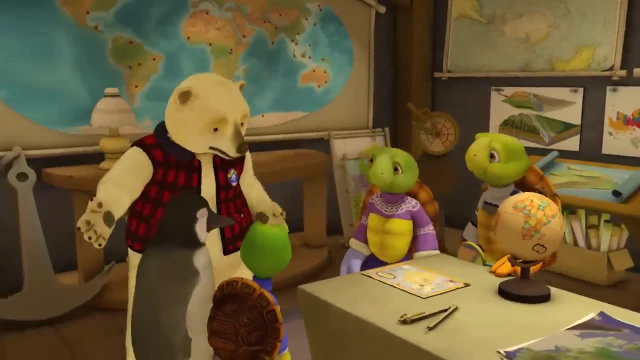 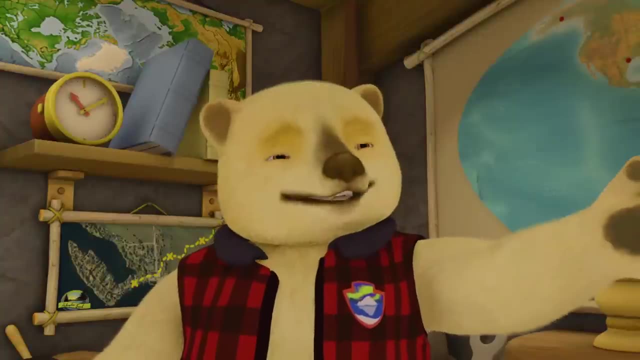 Oh, Not to sway you one way or the other. family decisions are important, But if Pip thinks he's ready to go home, I was going to offer him a ride in my plane. Wow, I wouldn't mind seeing Antarctica myself, Really. Thanks, Ranger. 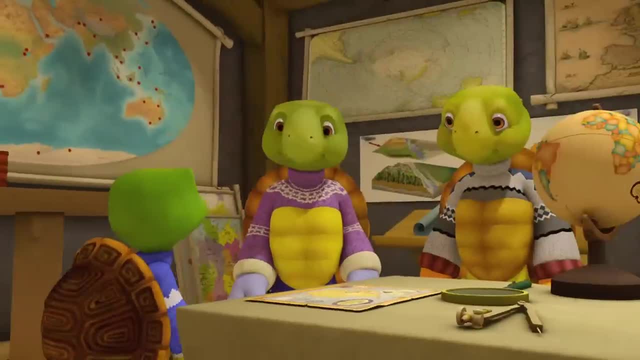 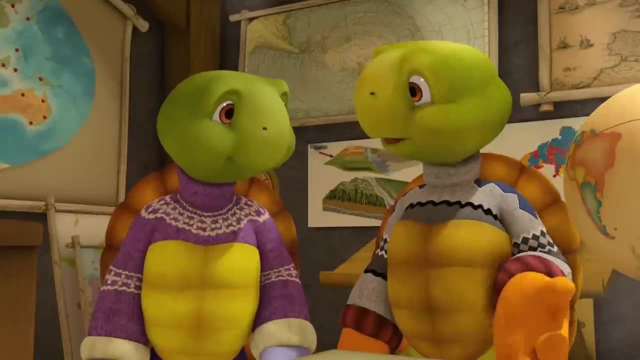 Come on, Pip, Mom, Dad, Ranger Bear and Pip are going. What do you think Should we? It'd be amazing And we probably won't get the chance again. We would need to call Aunt T and see if she can look after Harriet. 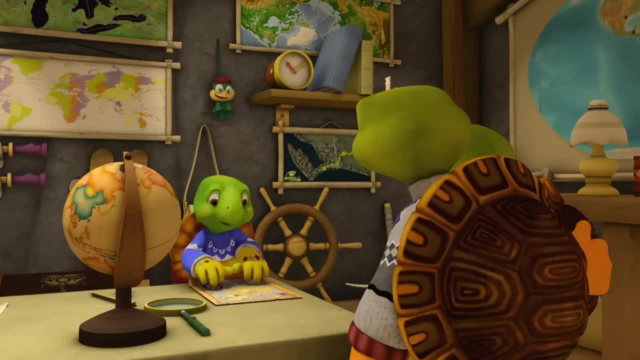 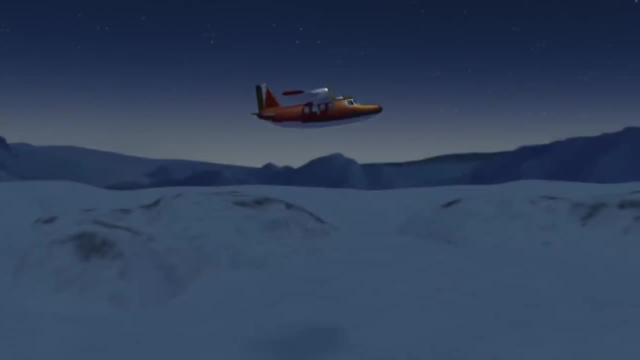 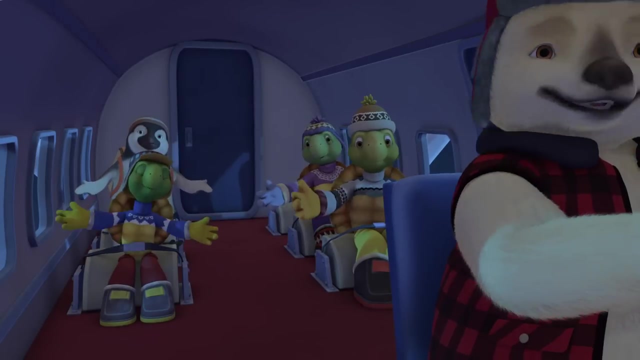 for a few more days. What do you say, Franklin? Yes, The turtles are going to Antarctica. Yes, We're on our way. Such a grand adventure. We're on our way To the Windy Pole. Windy Pole, I'll get you there. 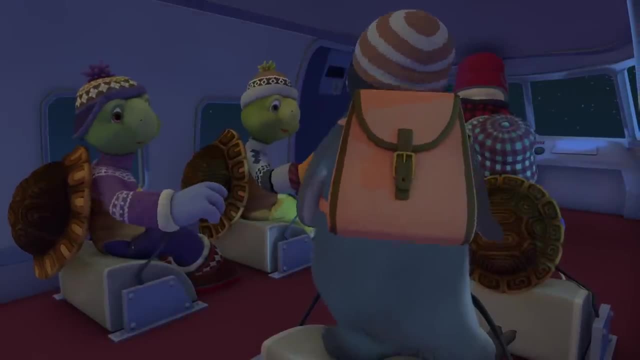 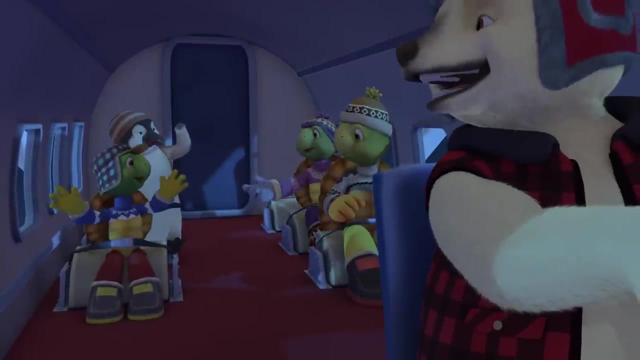 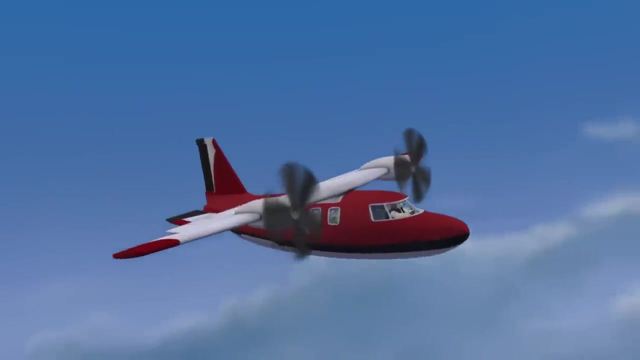 Maybe we'll find the treasure Come what may. To the South we go, South we go. We have the dream, We've got our team And we're on our way Off. we go Almost there Once we get through these clouds. Look out your windows, folks. 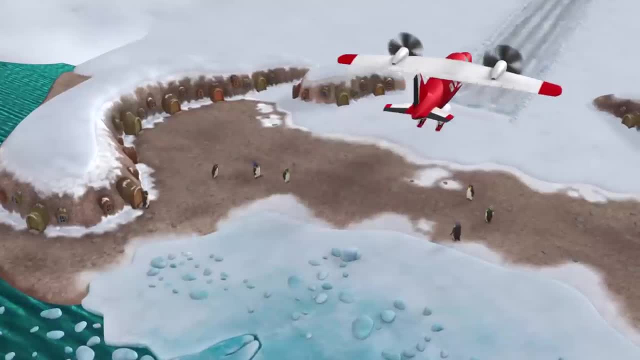 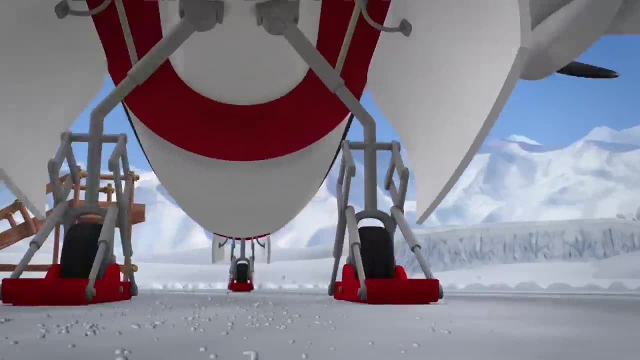 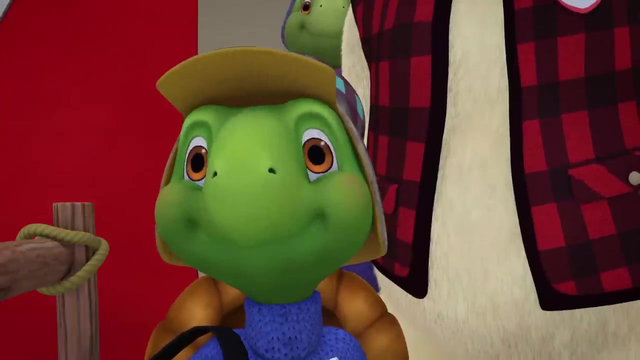 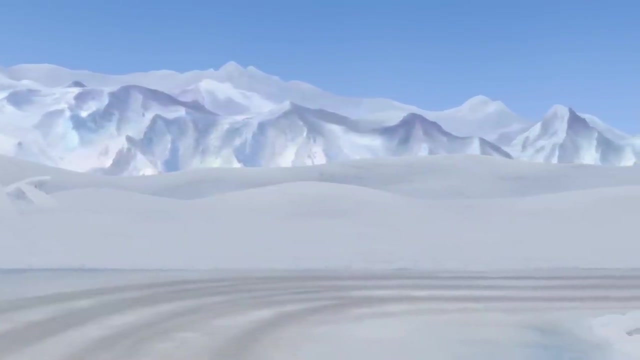 I'm home, Woo-hoo, Yeah, Yeah, Yeah. Here we are folks. Wow, it sure is bright here. Well, at this time of year, Antarctica has long sunny days and very short nights. It's just so lovely. 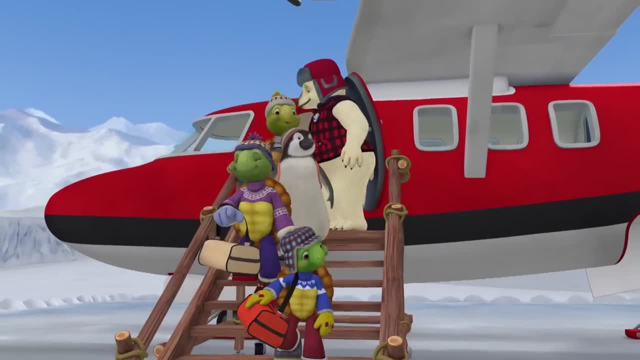 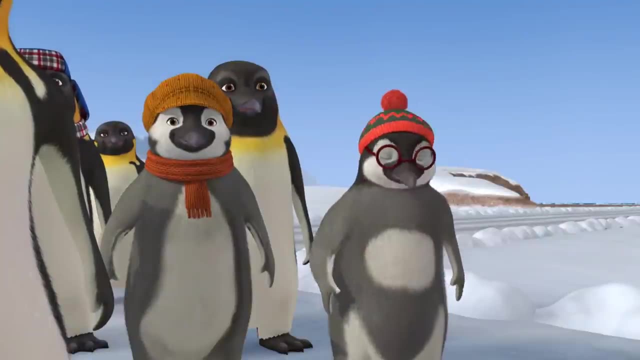 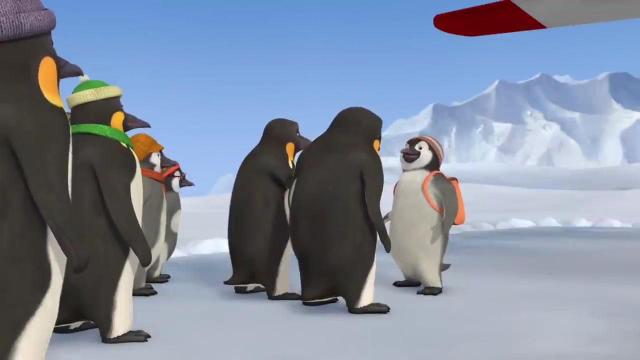 and blue And there's so much ice everywhere And penguins, Lots and lots of penguins, Hello, And I know all of them. There's cousin Fred and my friend Ava. Hey, everybody, I'm back And I brought new friends. 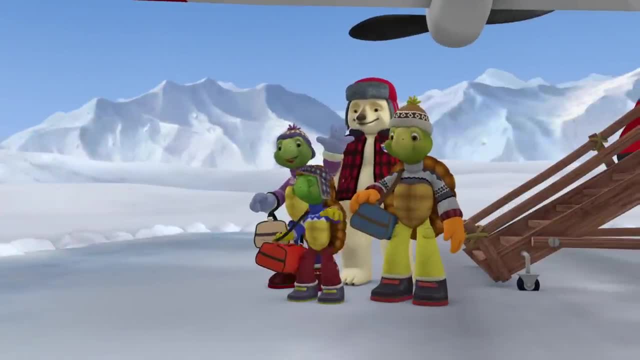 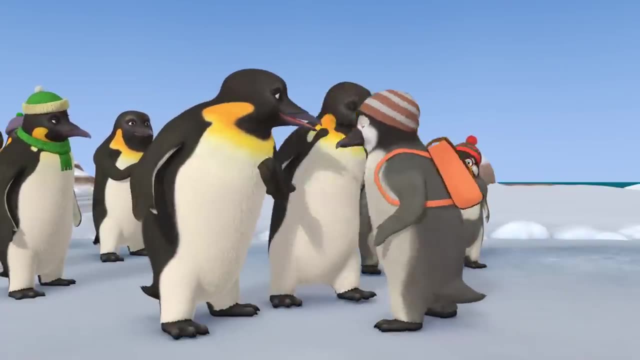 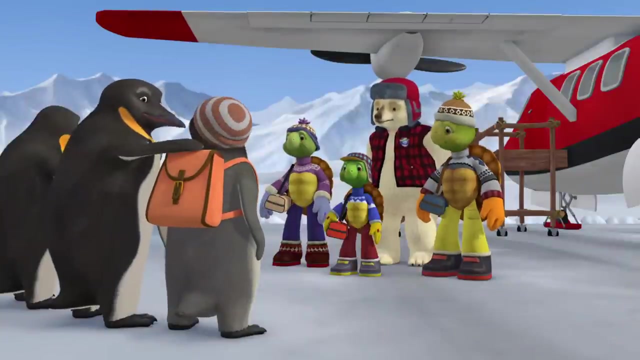 Mom, Dad, Ava, This is well everybody. Hello everyone. Hi, penguins, Pip, We're so happy you're home. Look at you. Hello everyone, Welcome. Thank you so much for bringing Pip home. 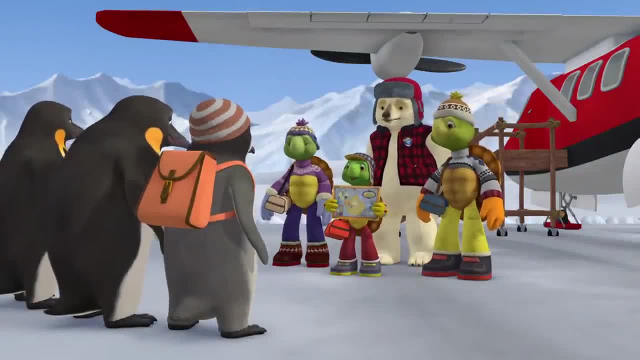 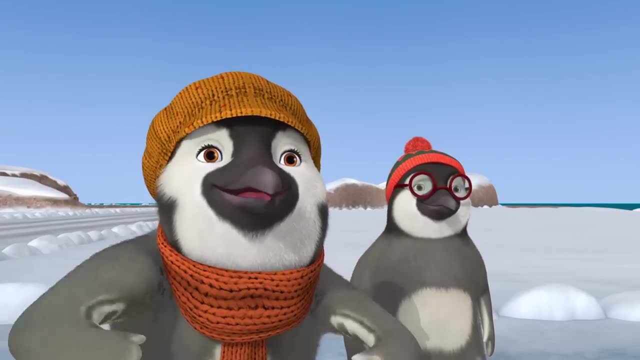 We didn't just bring him home, We found a map together, and now we're going on an adventure. How exciting. We'd love to hear all about it. Yes, I bet you guys are the first turtles ever in Antarctica. Well, Ava, that's not exactly accurate. 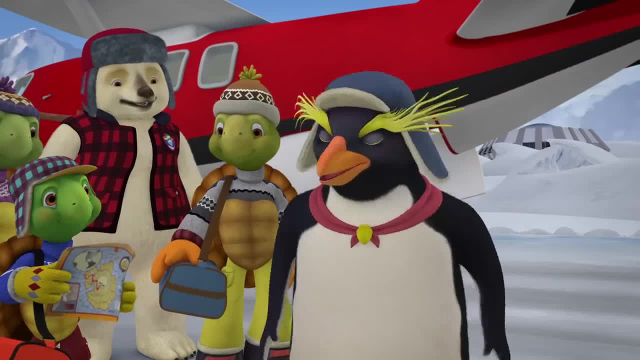 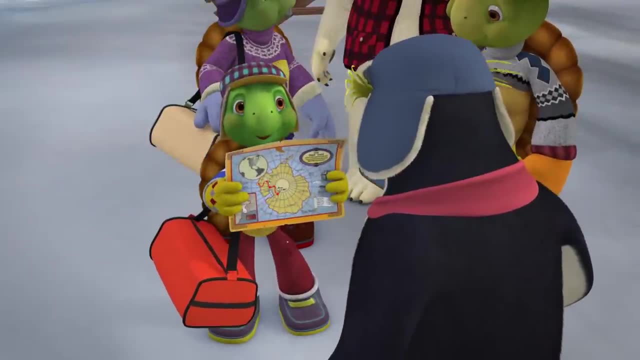 as I recall, Some time ago another turtle came here, A great explorer who goes by the name of Harriet. I believe That's my great aunt. We're gonna retrace her steps and find the treasure of the South. Whoa, Blow me down. 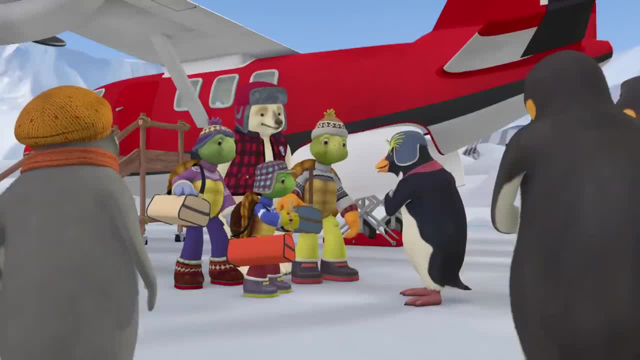 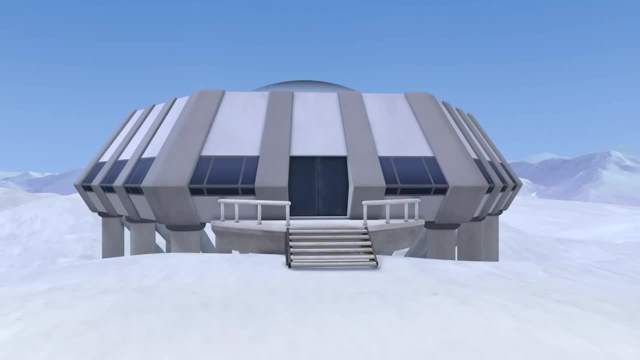 I'm Ranger Penguin. Kia ora folks- That's how we say- hello back in New Zealand. Kia ora Ranger Penguin. Well, come on over to the Ranger Station and you can tell me all about this adventure. That's some Ranger Station. 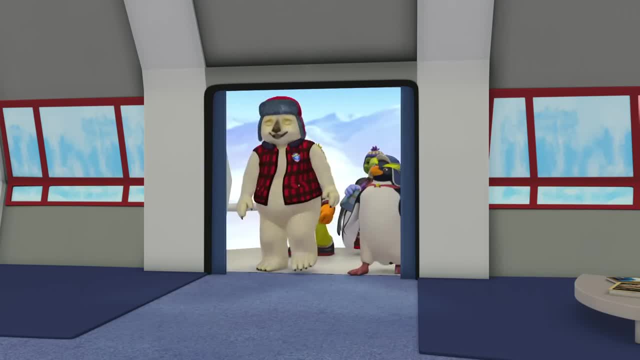 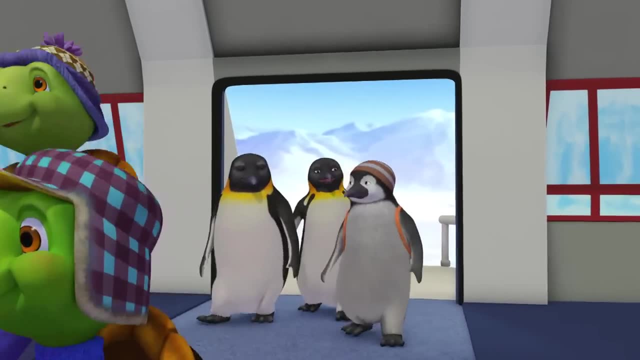 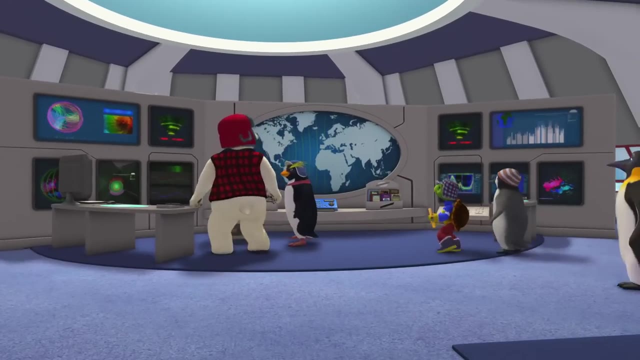 Wow Cool. And I had to dive into the water. and then a narwhal came and pushed the ice floe back to shore. Oh my, What's this Ranger Penguin? It's a 3D scanner. It redraws map terrain. 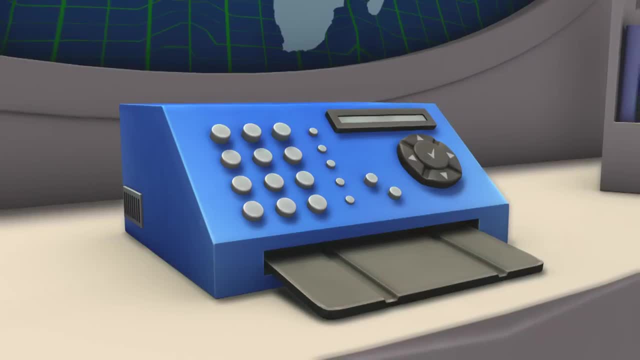 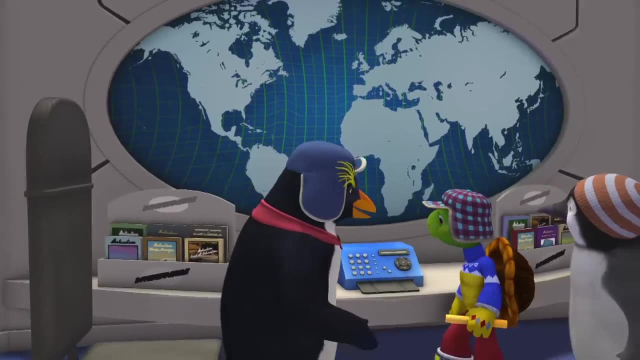 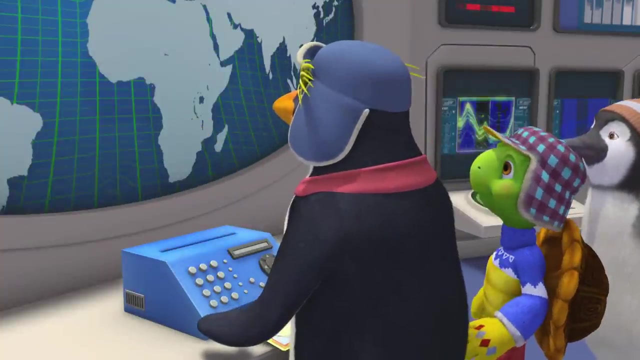 in three dimensions. Can I borrow that map of yours? Sure, Whoa, Wow, Cool, See, you're heading here towards the X. We'll look for the X and then we'll go back to the X. Cool, We're heading here towards the X. 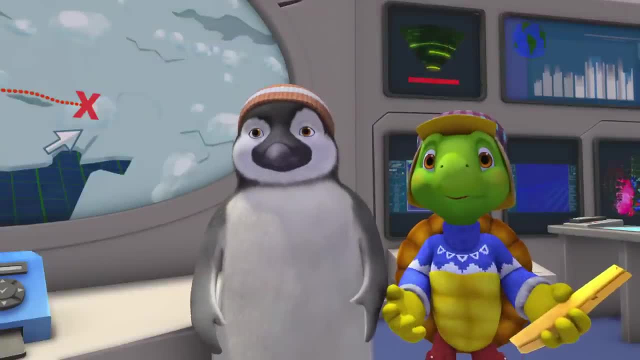 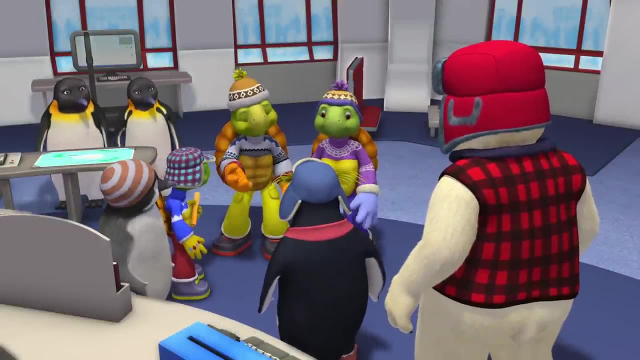 We'll go by snowmobile. Uh, we had a plan that we- I think what Franklin's trying to say is we- decided on the way that we'd retrace Great Aunt Harriet's footsteps on the map, exactly right down to traveling on skis. 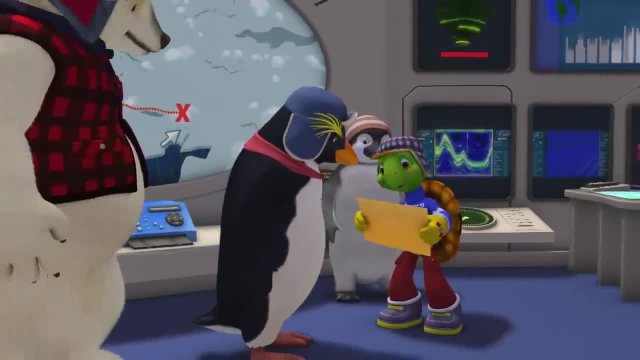 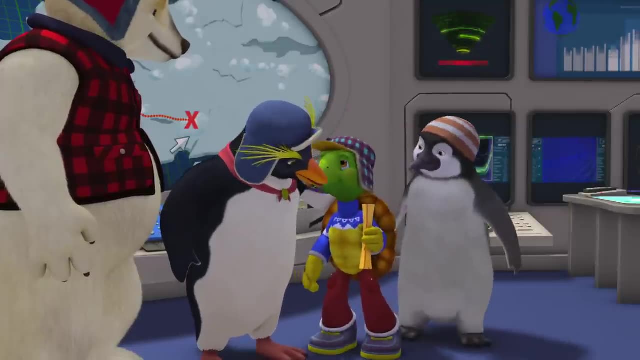 Well, that sounds like fun. Yeah, We're gonna follow her map, stop where she stopped and find the treasure of the South, whatever it is, just like she did. Well, you are a true explorer. mate Got all your supplies and the GPS. 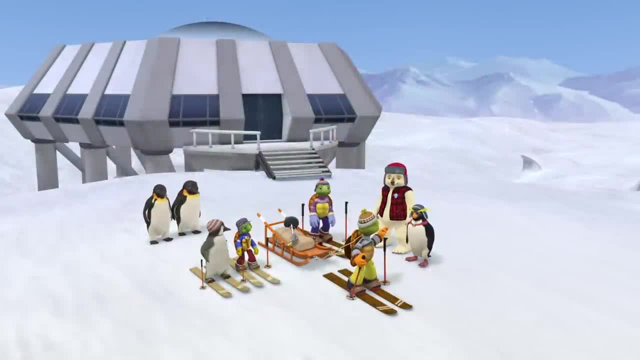 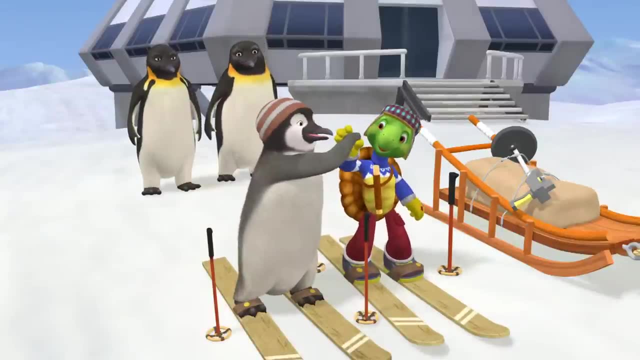 just in case you need it. All set, Have fun, honey. Ranger Penguin and I will be right here swapping Ranger Stories. if you need us Explore, Handshake High, low, wiggity, wiggity, wiggity, wow. 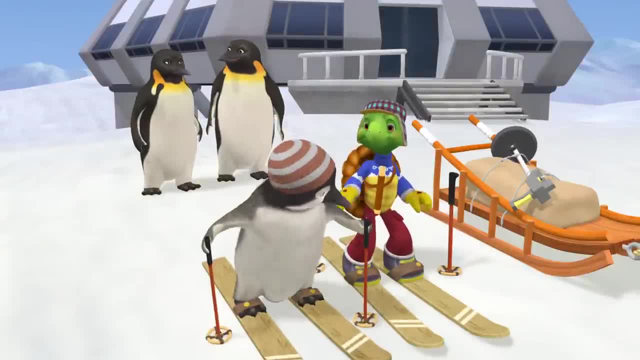 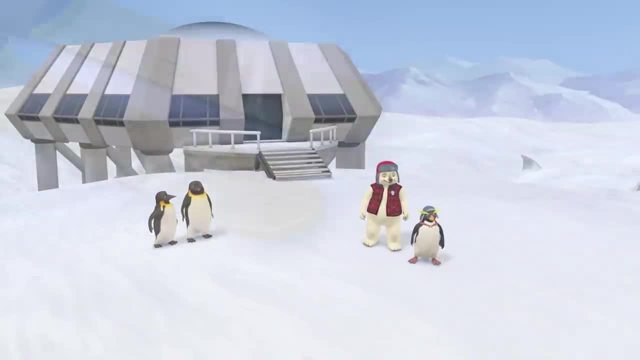 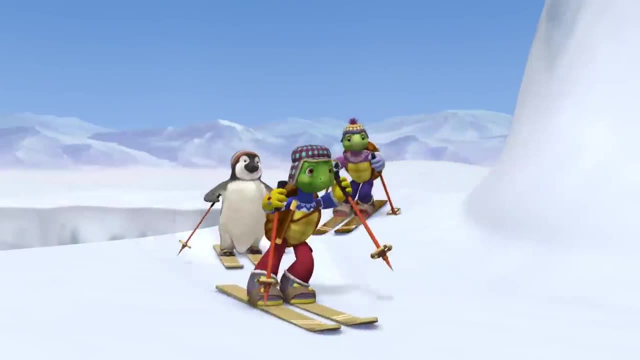 Whoa, We'll get it, Let's go. Bye Mom, Bye Dad. Safe travels, everyone Bye. now Come on guys, Let's go. Oh awesome, Look at that The sun's making a beautiful. 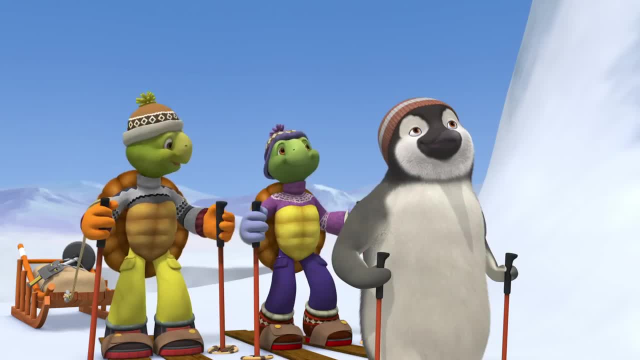 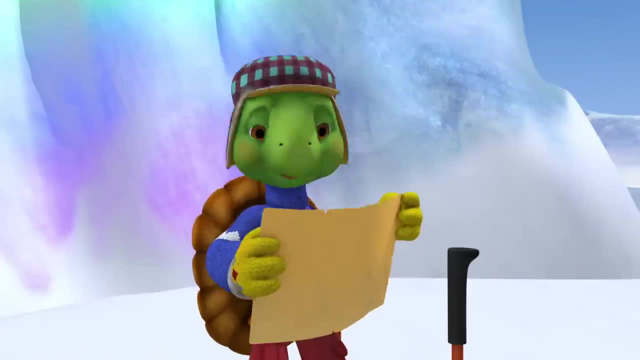 ice rainbow for us. Come on everyone, It's this way. We should take some photos to bring back home. Huh, Great idea, dear, I'll get the camera, But we should get going. Great Aunt Harriet didn't stop here for photos. 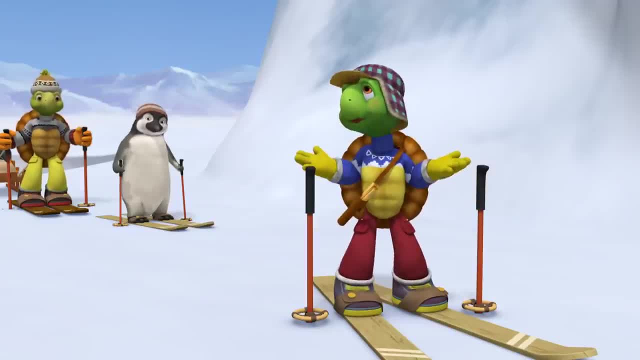 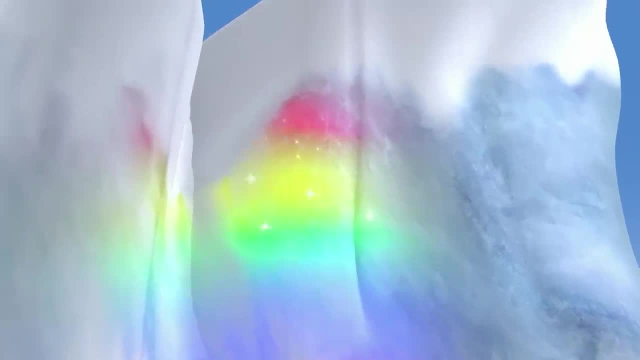 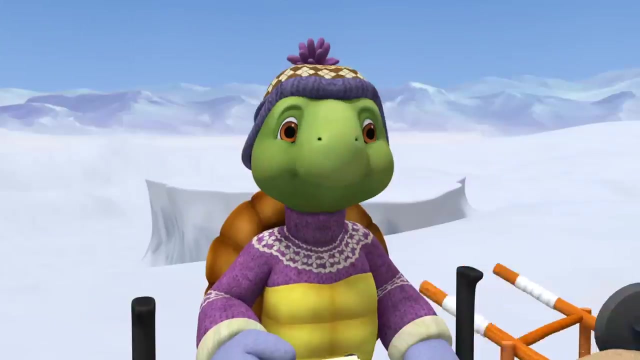 It won't take a minute, son, And just look at the view. Are you kidding mate? Look at it. Whoa, Whoa, Whoa. Okay, it's pretty great, But can we hurry up? Okay, everyone. 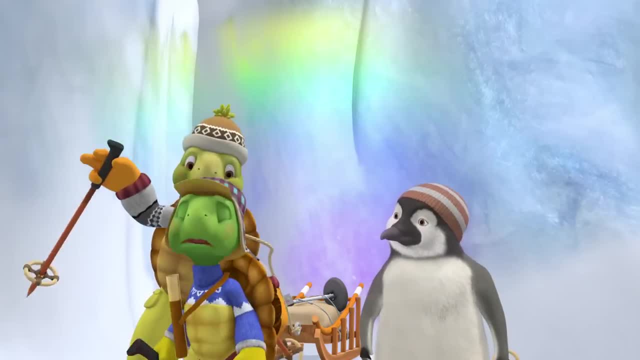 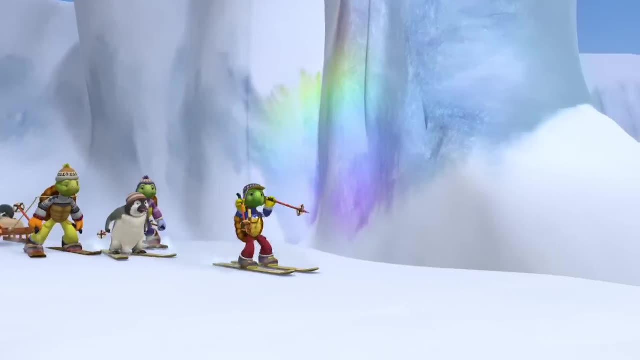 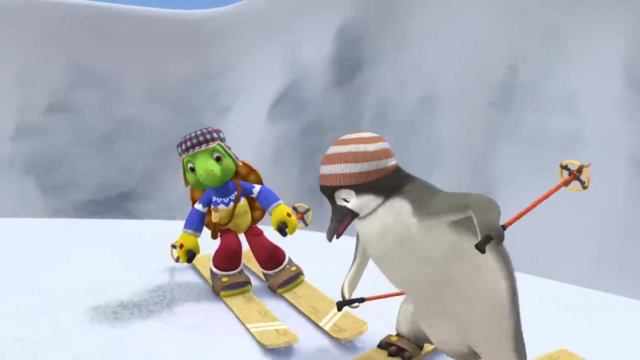 Say rainbow Rainbow. Okay, okay, Let's go. everybody, We gotta get to the spot. Great Aunt Harriet camped at This way. Whoa, Hold up, Franklin, What's your hurry? You're gonna get there. 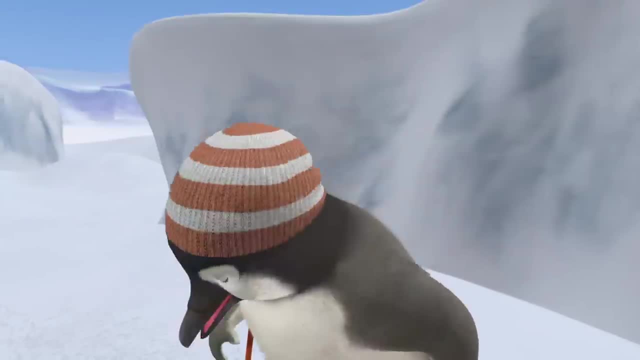 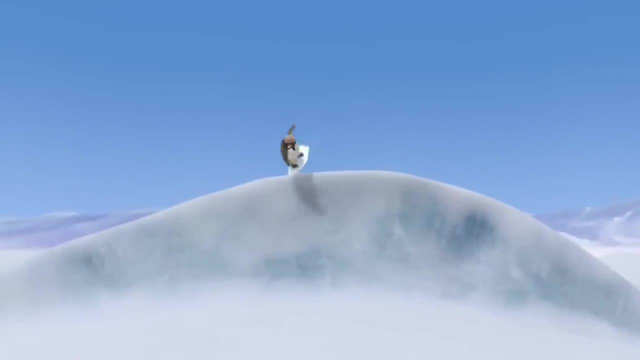 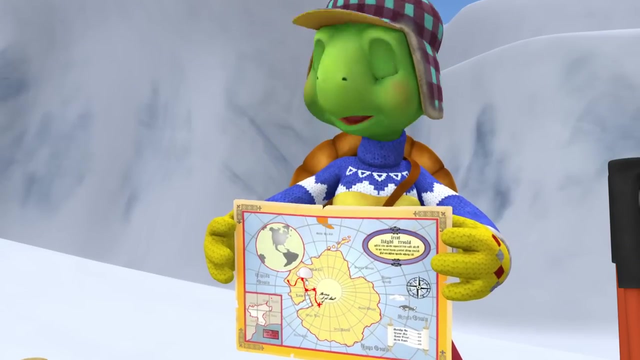 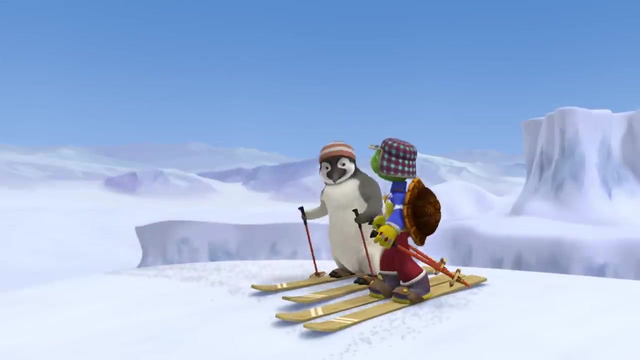 Don't you worry. Why not stop and look at the view? Ooh, Enjoy the ride Like I do If I see you hesitate. Here's the thing. I just can't wait. I like to get there when I can. Ooh. 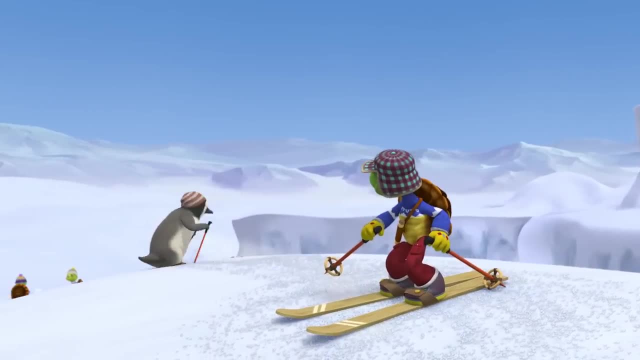 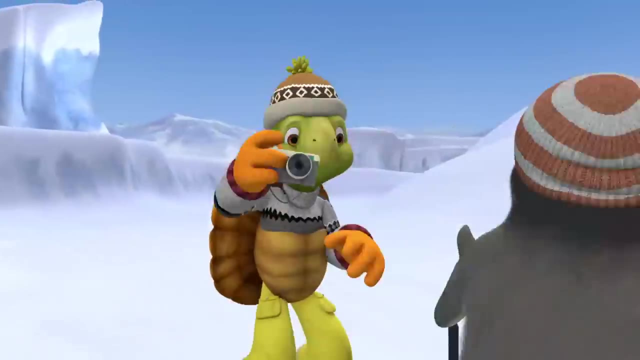 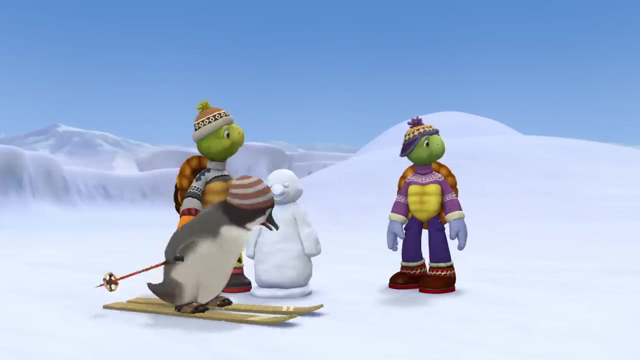 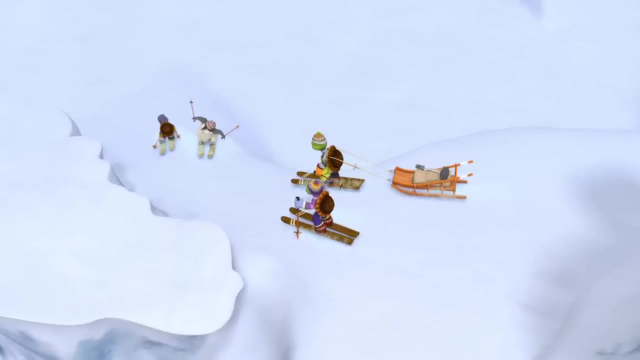 I stick to the master plan, Though you've got your eyes on the prize. sometimes, when you improvise, you might find some wonderful surprises. Hold up, Franklin. What's your worry? I can't help it. I'm in a hurry, And though I love to enjoy the views, 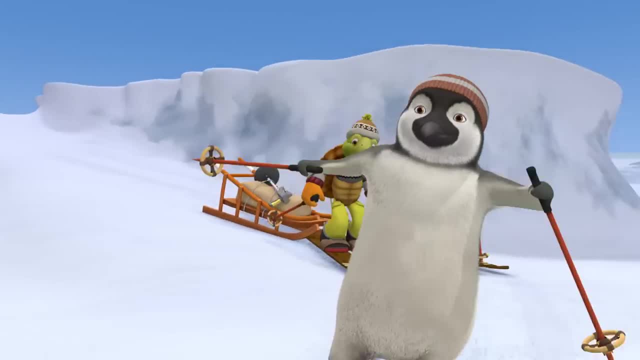 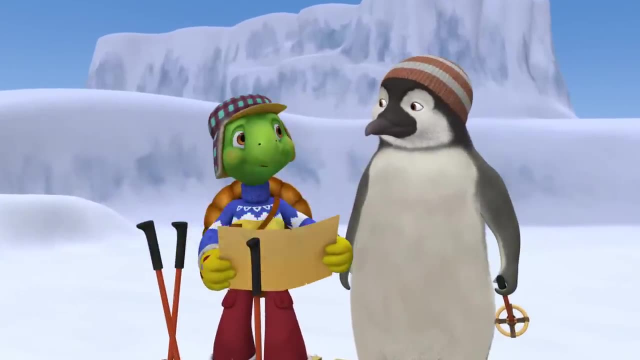 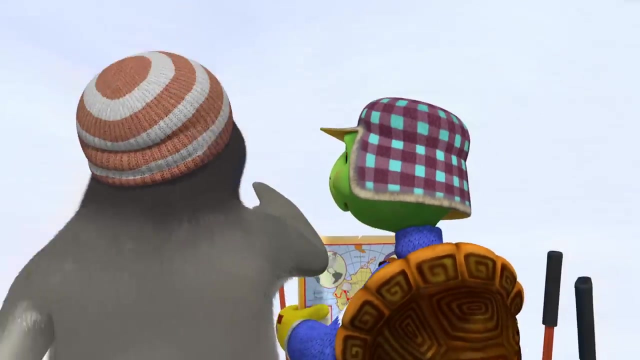 we've really got no time to lose. Whoo, Yes, I think this is it. This is where Great Aunt Harriet camped. Hey, you're right, She drew a little igloo on the map in a valley just like this one. 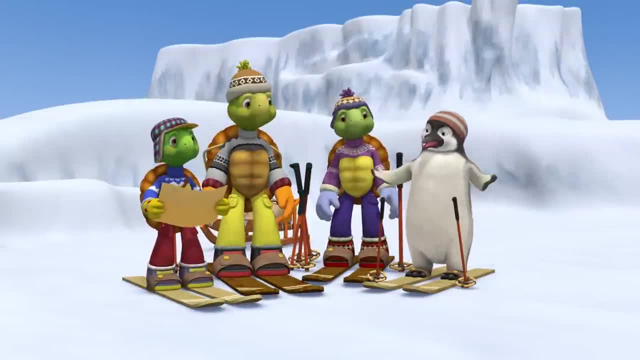 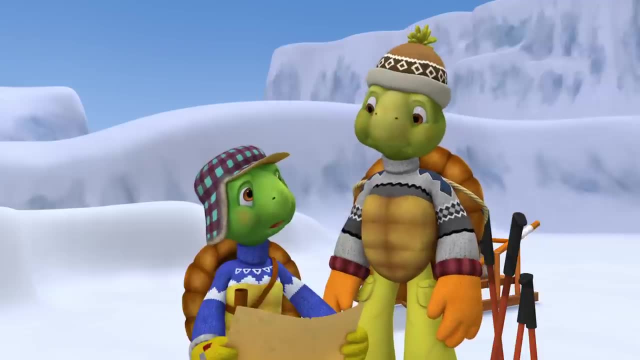 So then, this is exactly where we have to camp, But it's way too early to call it a day. Hmm, We were hoping to get a little farther before setting up camp. We wouldn't be following Great Aunt Harriet's route exactly. 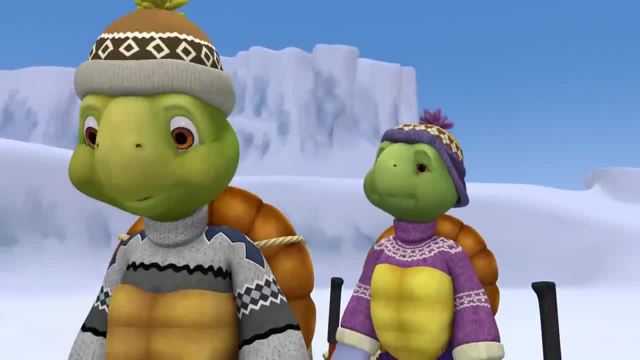 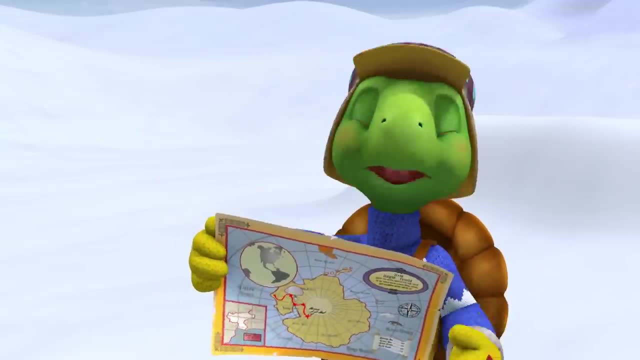 Franklin, you're not the only one on this adventure. We're all here together, son, And have to decide what to do as a team. I'm sorry, I just really want to follow the map, the exact same way Great Aunt Harriet did. 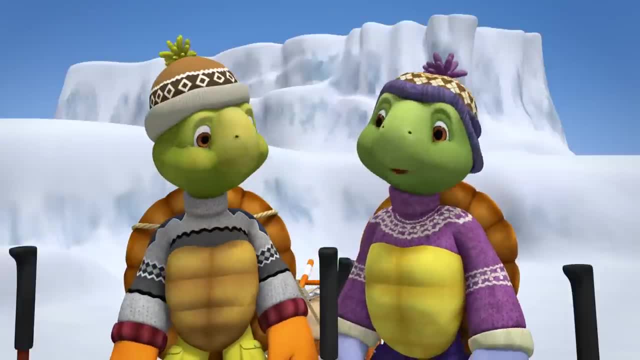 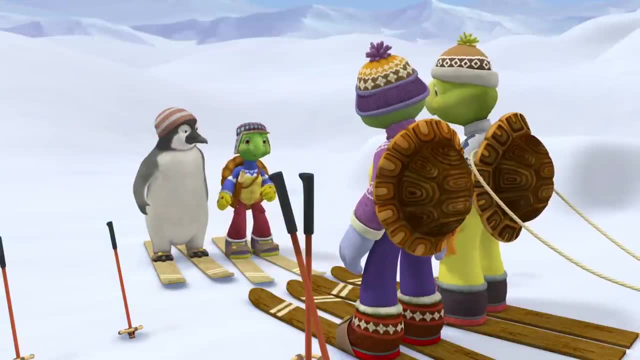 I get it. You've got your mind super set on sticking with the plan. It's cool with me. Well, okay, As long as we're all agreed, I'm fine with setting up camp now. That's great. But what if we end up in the exact same spot? 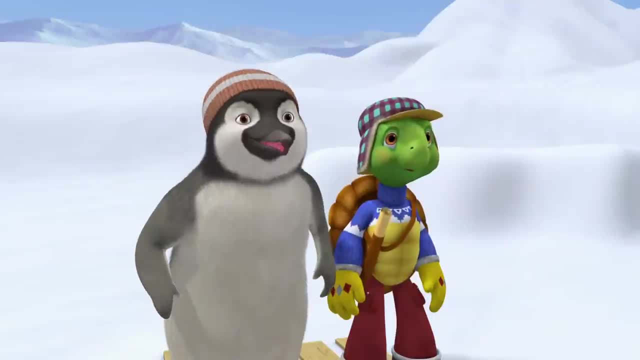 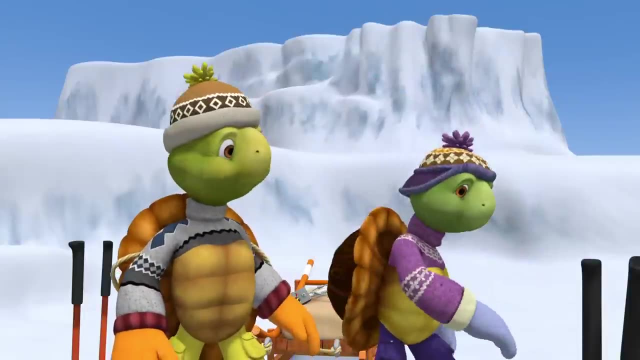 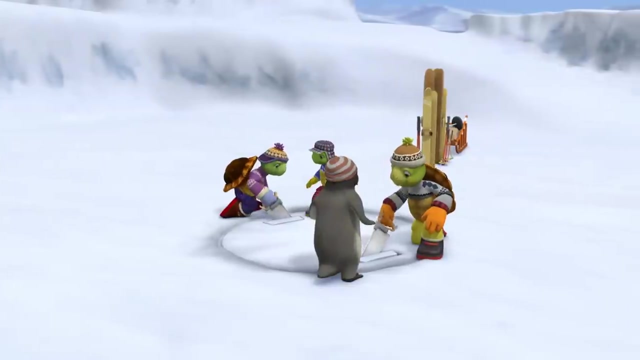 she did, Oh, and that we slept in an igloo just like she did. An igloo. Really Awesome How Mom Aunt Harriet showed me how to build one when we went winter camping together. Come on, I'll show you. 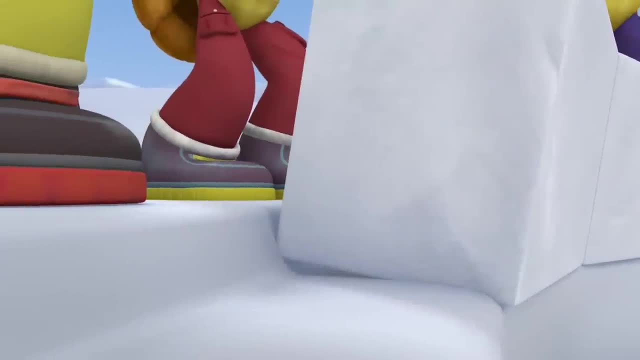 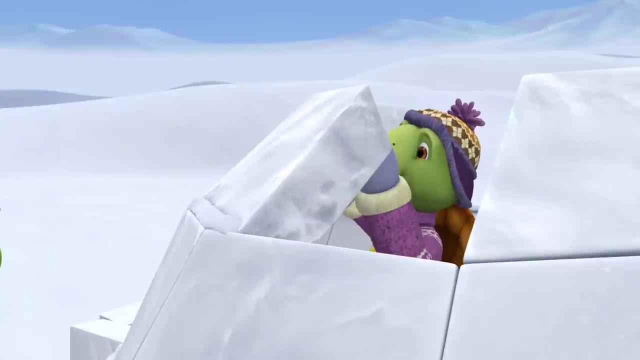 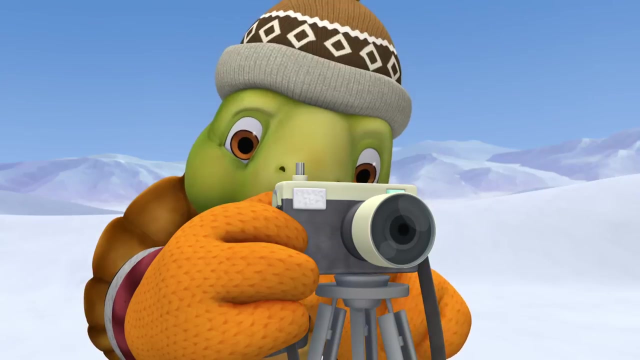 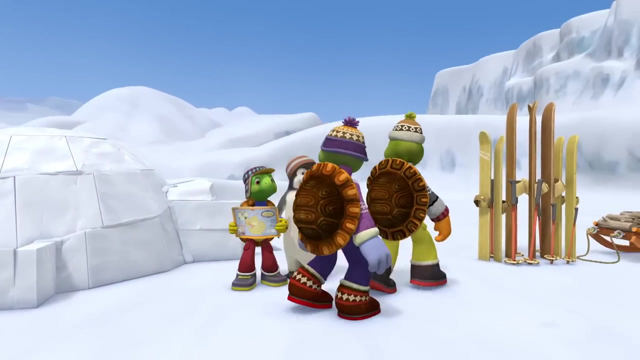 All right, Mrs T, This is so cool, Let's go Perfect. Yay, Okay, you boys can go play while your mom and I make supper, But stay close. Come on, let's go practice our explorer handshake. 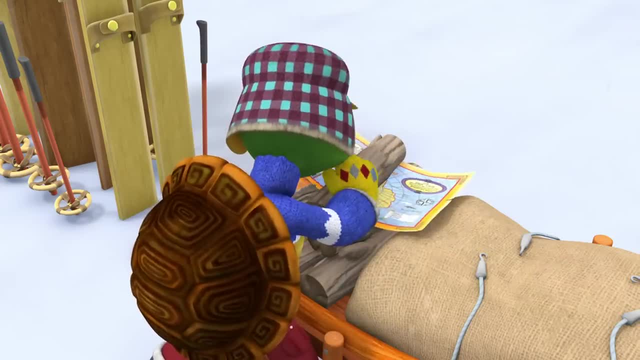 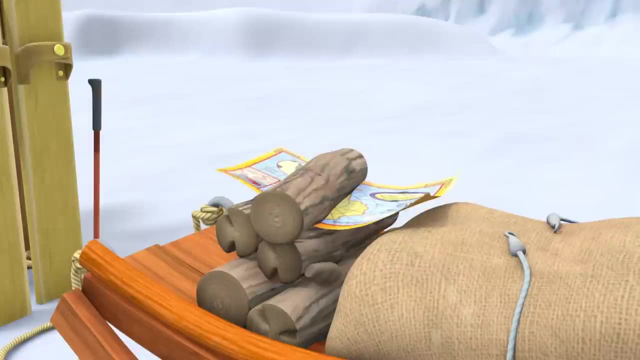 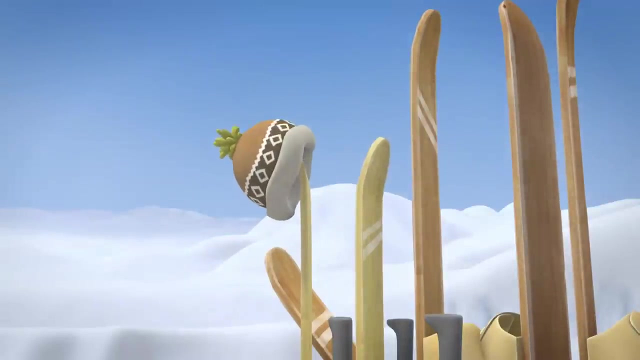 Okay, I'll just put the map down here. Whoa, It sure is windy. Yup, we've got lots of wind in Antarctica: Super high, Super low. Wiggity, wiggity, wiggity, Wow, Oh no. 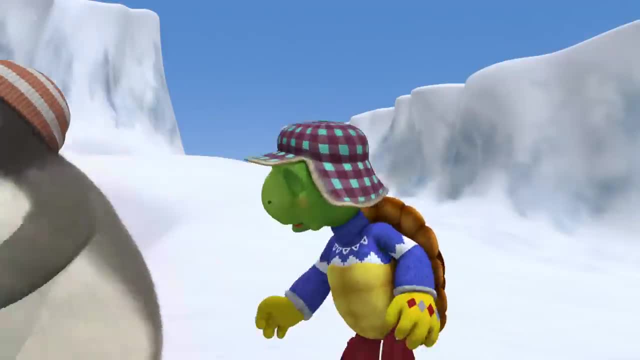 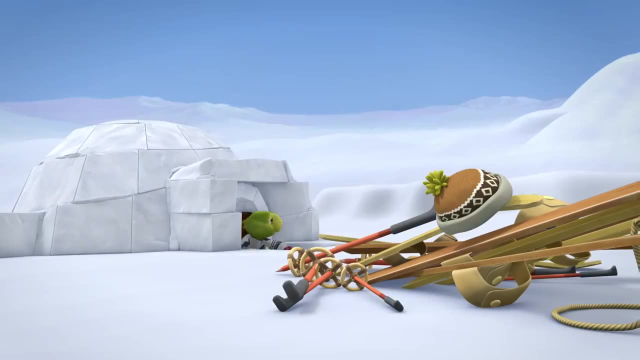 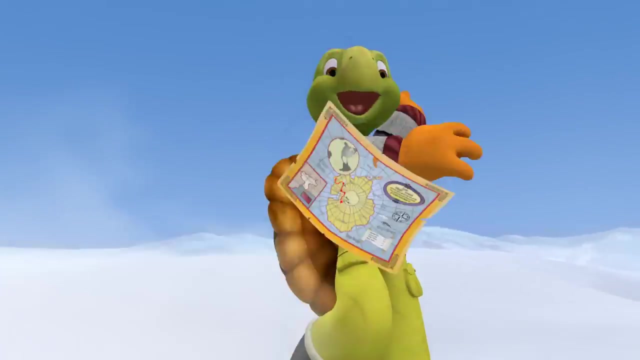 There go our skis, The map, Get it. Pip, Do you have a break? I got it. Everything okay out here. Whoa After that map. Oh no, Let's go, Got it, Don't got it. 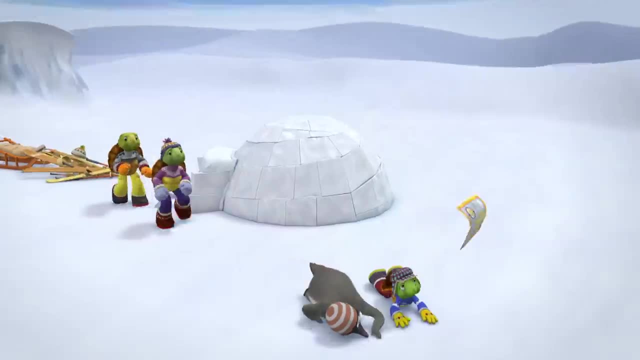 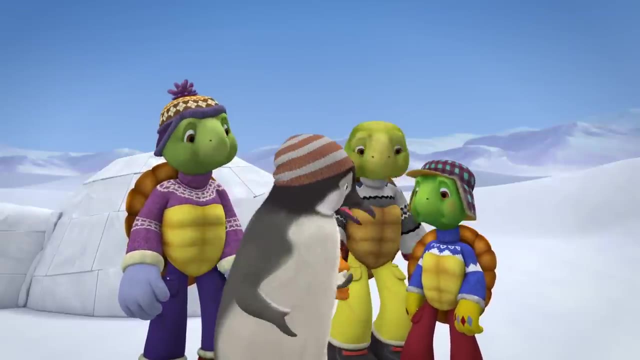 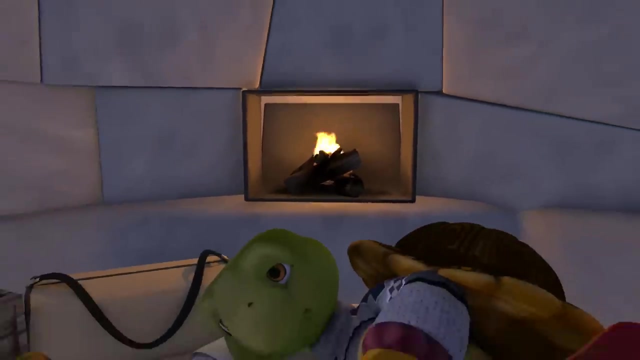 Come here. Oh no, There it goes, Yes, No, Oh, dear. Well, that's it. We've lost the map. Sorry, Franklin, It took us to get back to the ranger station, right, But how are we going to follow? 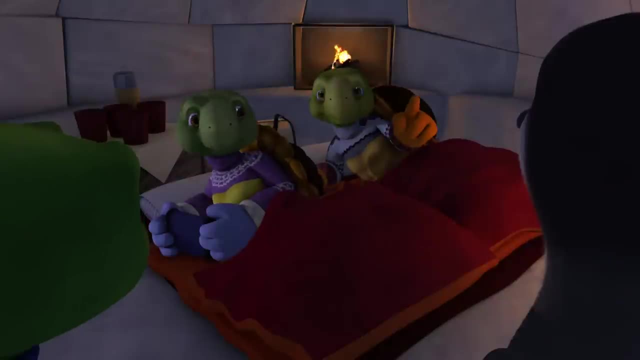 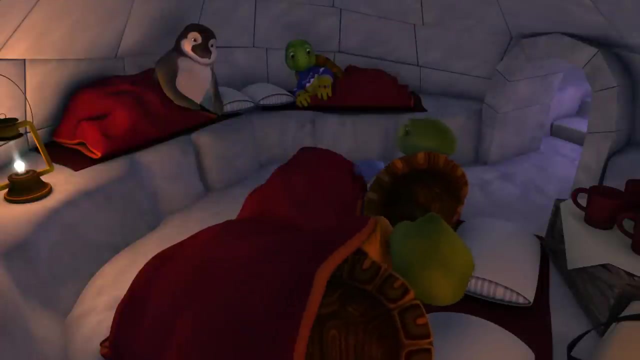 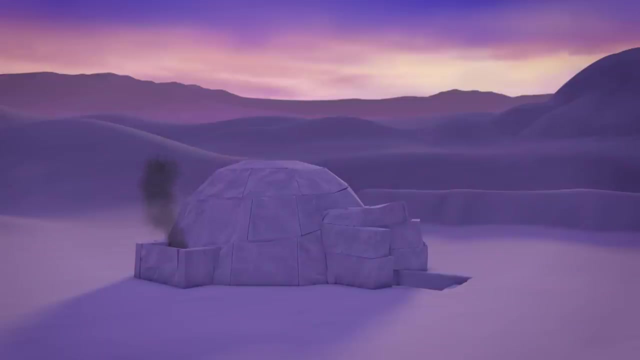 Great Aunt Harriet's footsteps, without the map. Tomorrow's a new day. We'll put our heads together and come up with a great new plan. Until then, it's bedtime, explorers. Good night, Good night. Good night, Don't worry, mate. 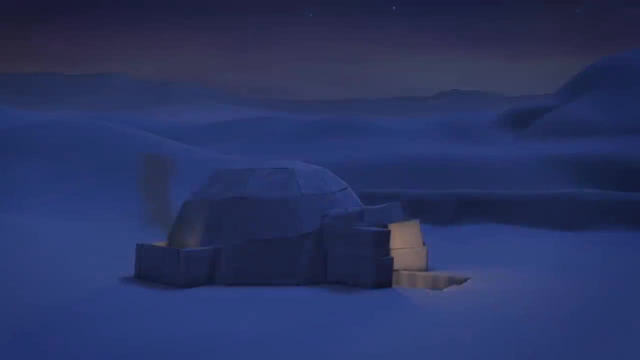 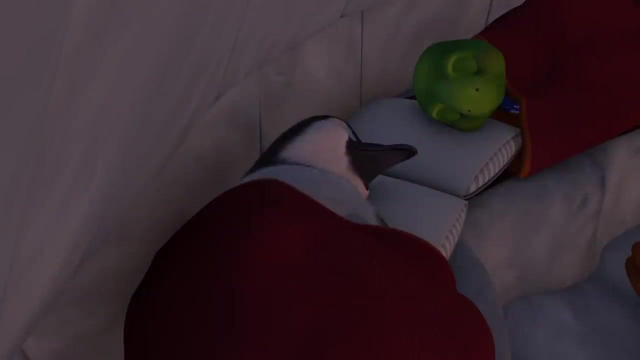 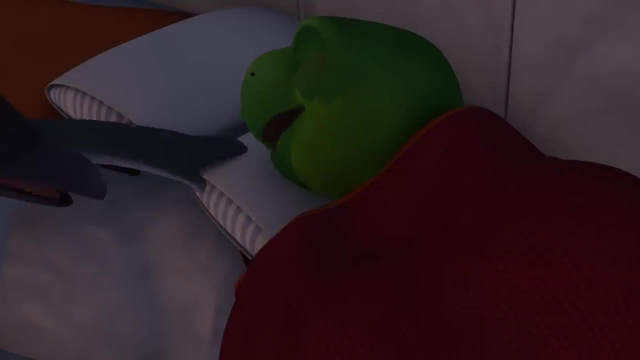 We'll figure out how to keep going. I know we will. Yeah, I hope so. That's it, Franklin. I know how to get the map. Wake up, little buddy. Okay, I'll get it and bring it back. 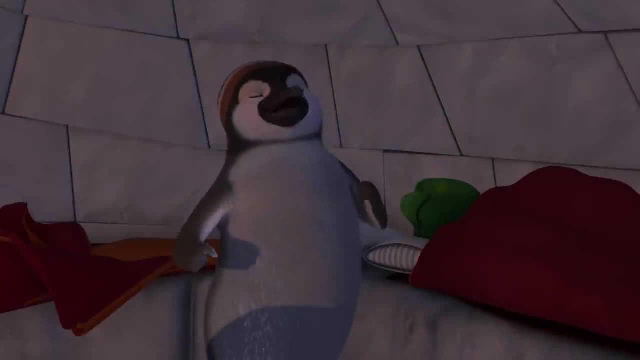 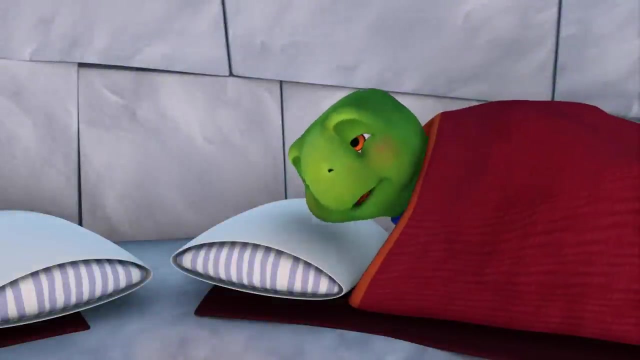 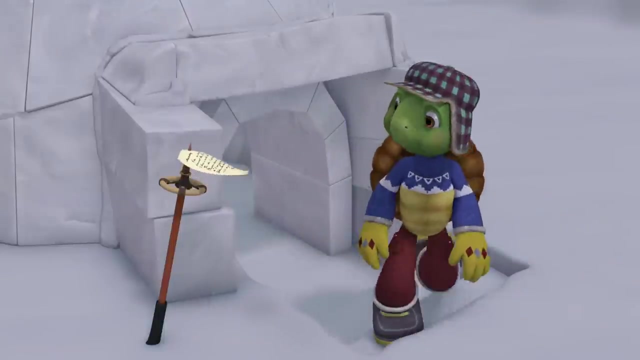 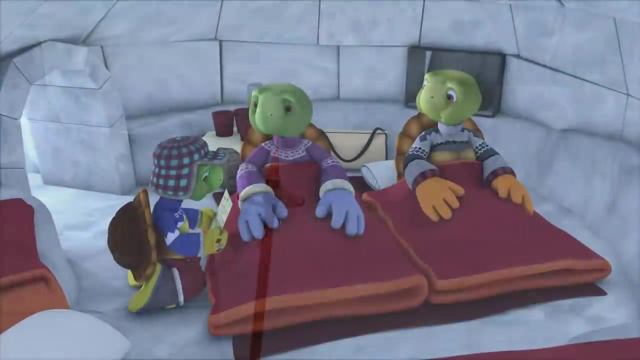 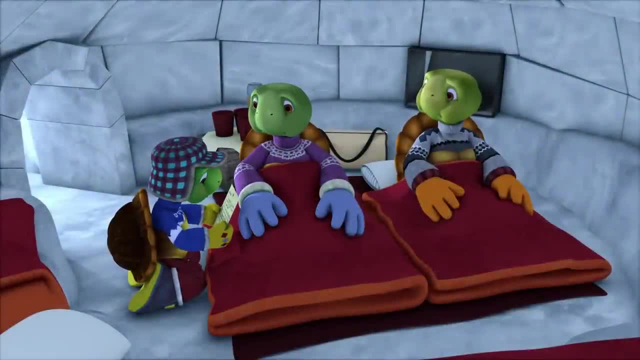 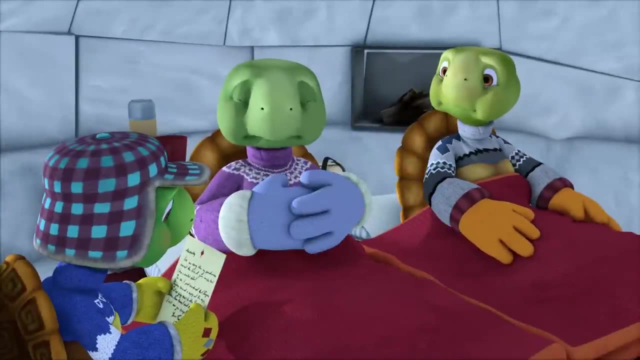 Pip's going back to the station to get a copy of the map from Ranger Penguin. He says we should stay put and he'll bring it here. We have to go find him. He may be an experienced explorer, but I am a mother and I can't let him go all the way back on his own. 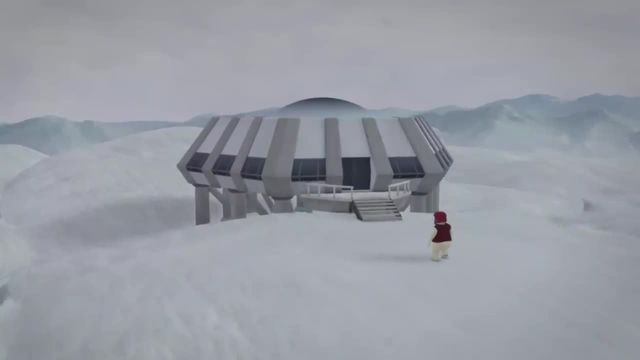 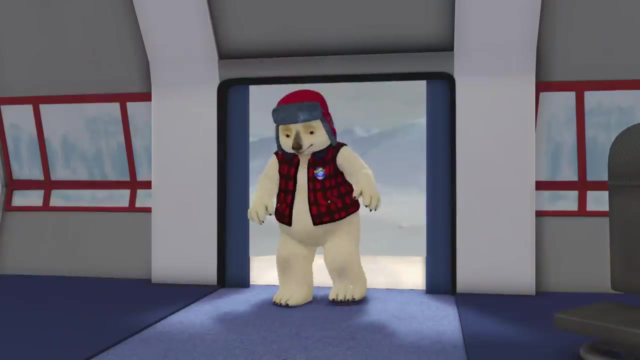 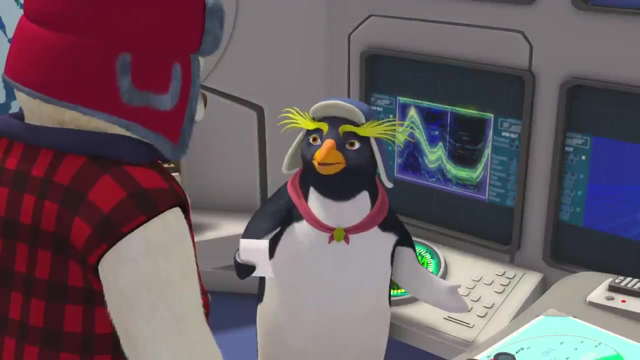 Let's pack up, Let's hurry. We have to find him, Nook. Not good, Not good at all. Good morning, Gwynny. What's going on? Something wrong? It's a bit of a worry, Barry. 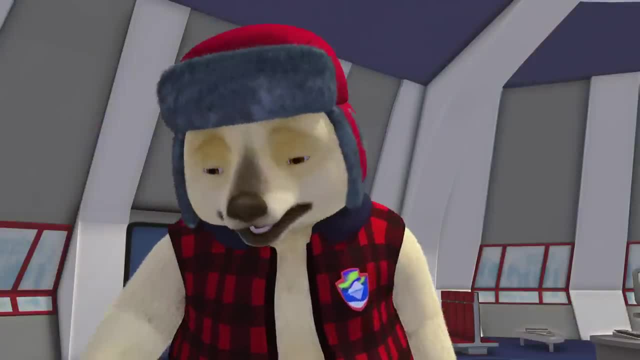 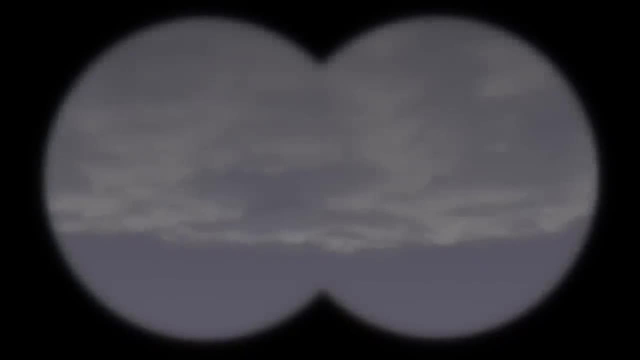 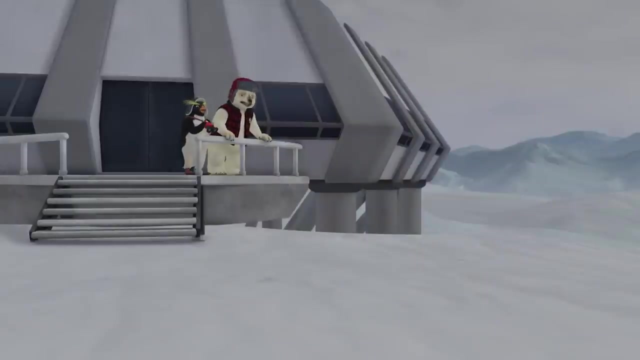 Satellite's telling me a real nasty blizzard's moving in, Could be heading for the turtles. Let's take a look outside. There I can just make it out- Weather's turning to custard. Yep, you're right, Blizzard's on the way. 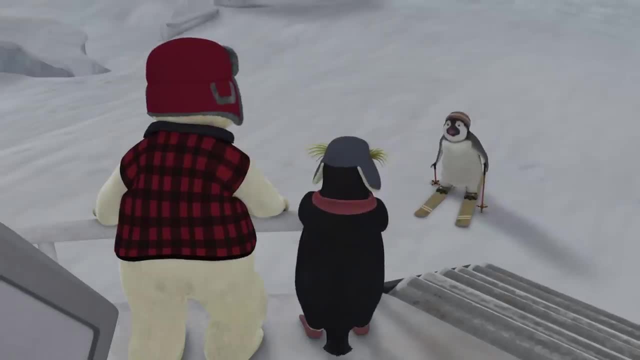 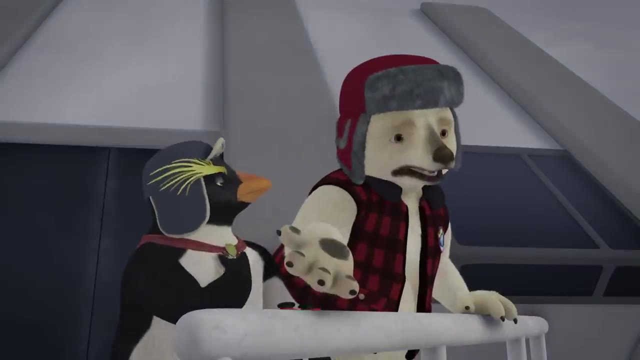 Hello, Huh, Do you have a copy of Franklin's map in your scanner, Pip? What are you doing back here? I skied all night. We lost Great Aunt Harriet's map in the wind. Oh no, What about the turtles son? 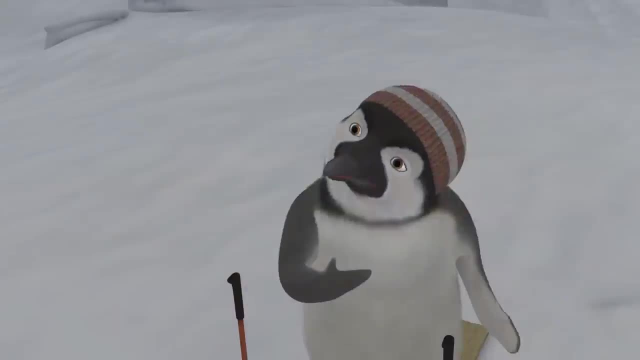 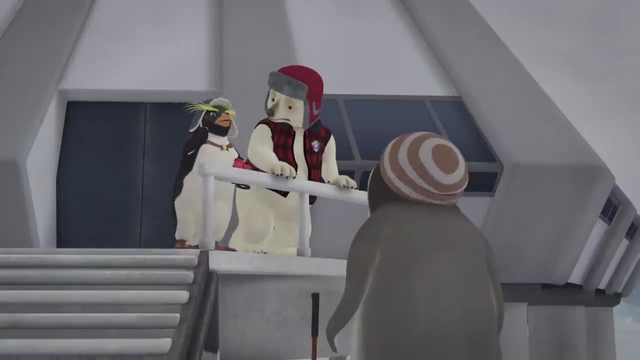 Are they out there on their own? It's okay, I told them to wait for me. I'm going back right now, As soon as I get your copy of the map. We've got to go get them. Barry. Antarctica's no place for a family of turtles caught in a blizzard. 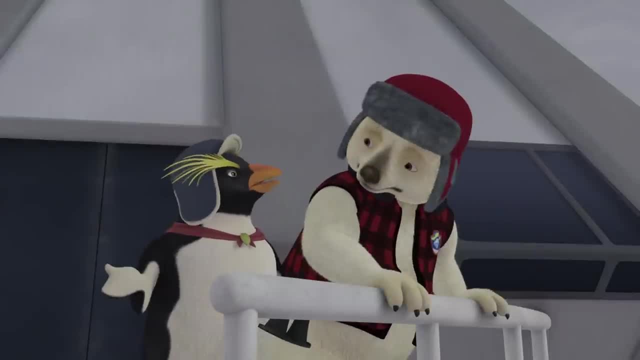 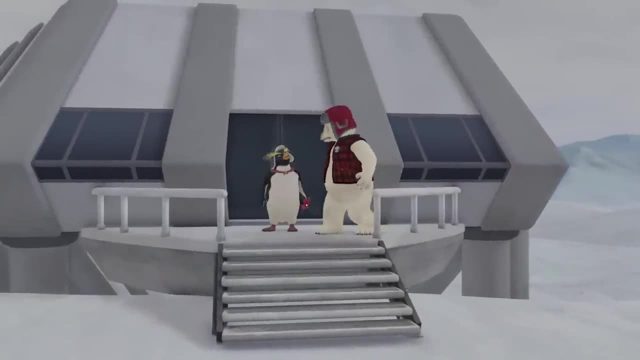 Blizzard. Oh no, I'll gather some supplies and get my copy of the map. Pip, you go fetch your parents, I'll get the skis. This is an emergency. We'll need something faster than skis Rangers, We're here. 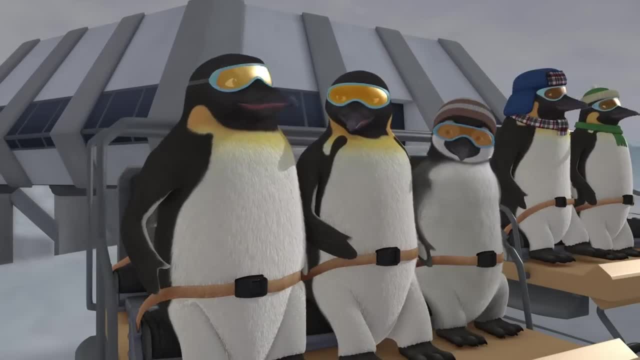 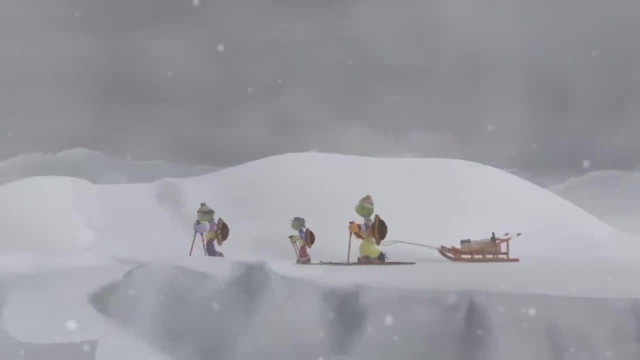 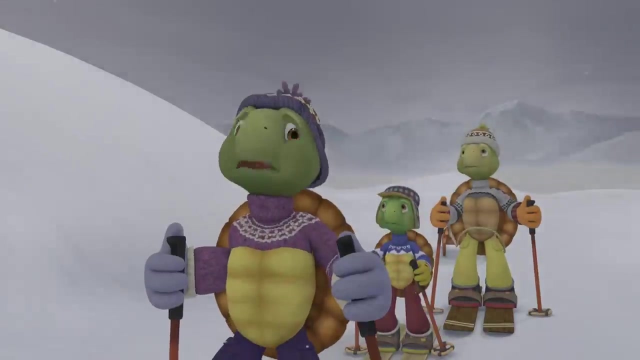 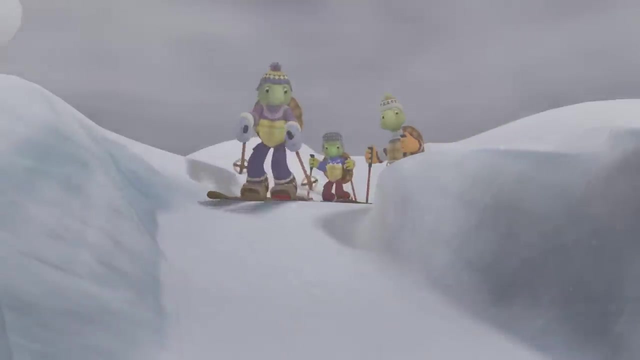 We're ready to help Lead the way. Come on, Let's go. Great, That's a storm coming. Let's take cover down in that ice valley. We should be able to find shelter if the wind's there. Good idea. 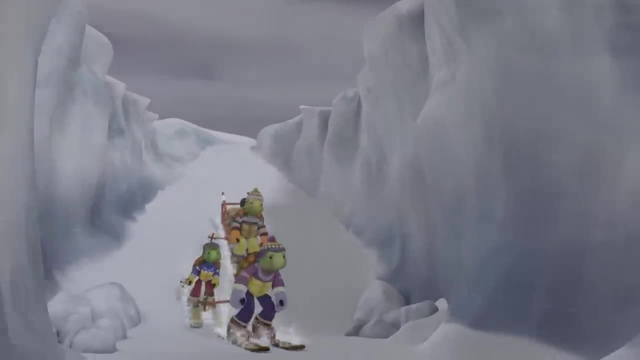 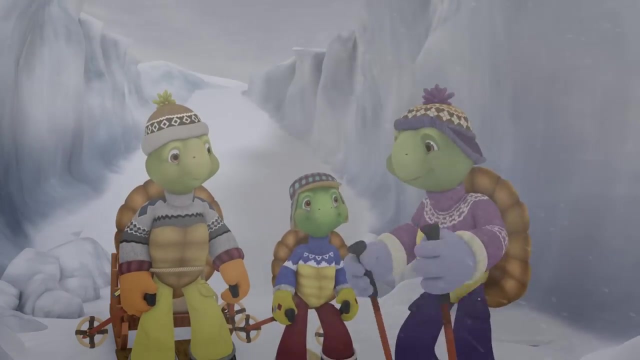 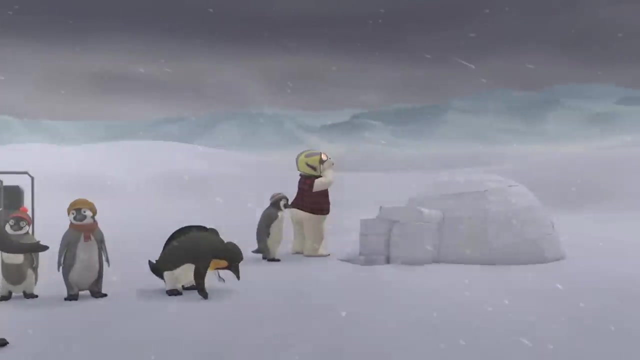 Come on, Let's stick together. Okay, Come on everyone. Look, There's an opening we can take cover in. Good eye, Franklin, You're getting good at this. explorer stuff. Franklin, Mr and Mrs Turtle, They're gone. 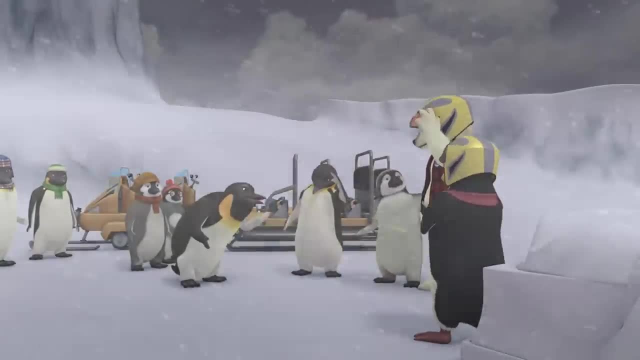 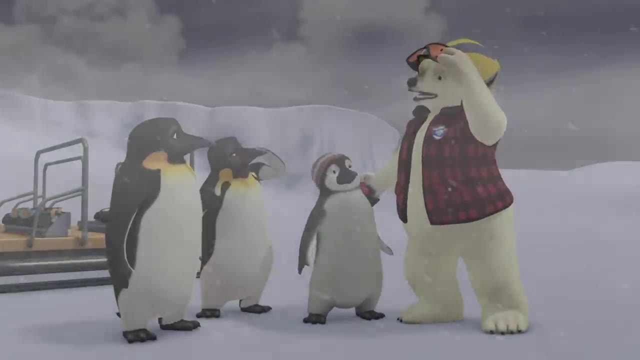 We can't tell which way they're headed. Their tracks have been erased by the wind. If those turtles are as smart as I think they are, they probably took cover when the storm hit, Maybe in that ice valley we passed. You're one clever bear Ranger. 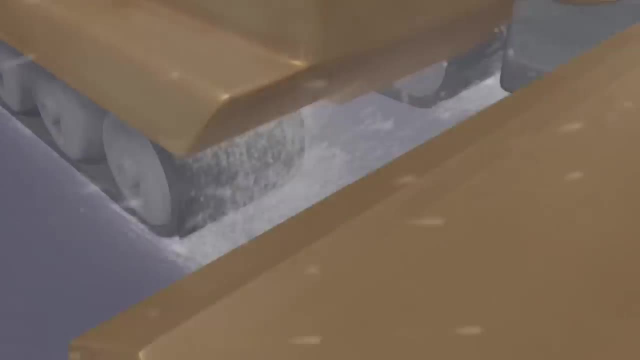 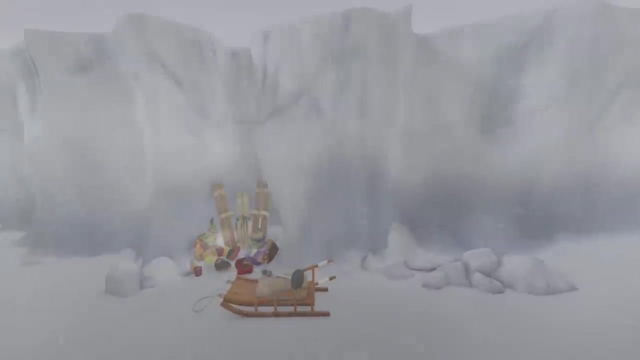 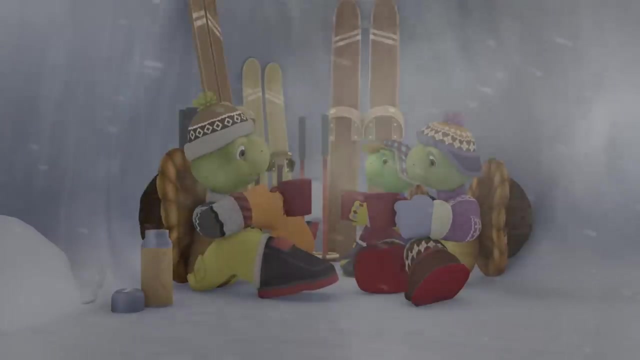 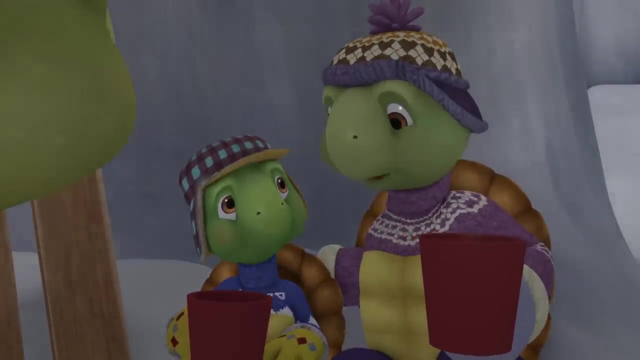 Let's go. everybody Still hot. Let's stay close to stay warm. Well, this is an unexpected adventure. I bet that's Great Aunt Harriet's favorite kind, Don't you think, Mom? do you think Pip is back at the station by now? 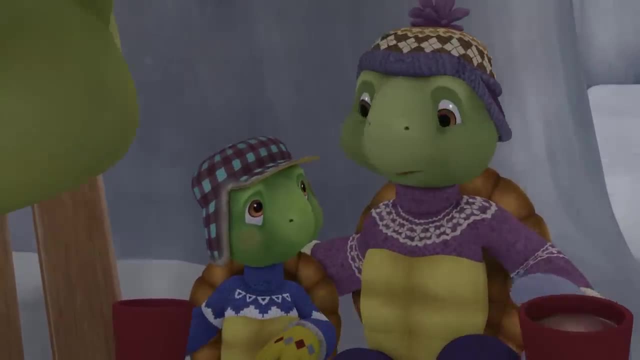 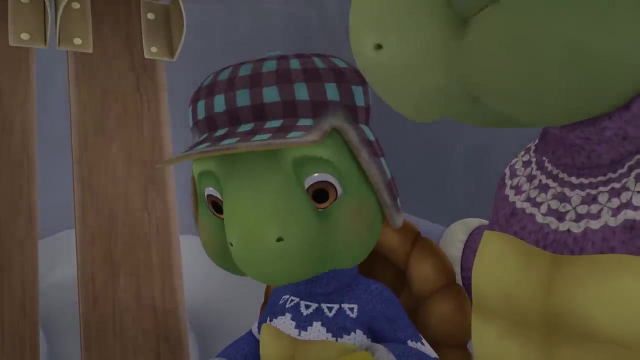 I'm sure he is. If I hadn't made such a big deal about the map, he never would have gone off on his own. This was supposed to be our adventure together. I'm gonna tell him that when I see him As soon as this storm passes. 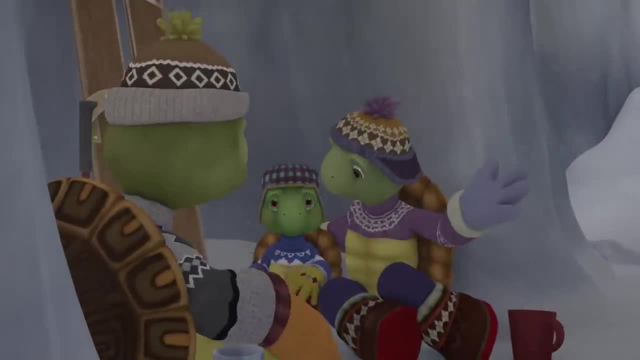 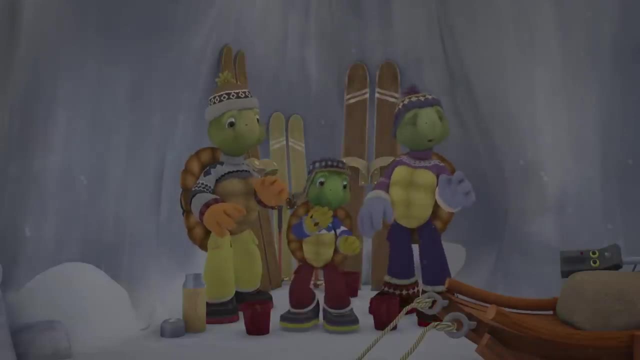 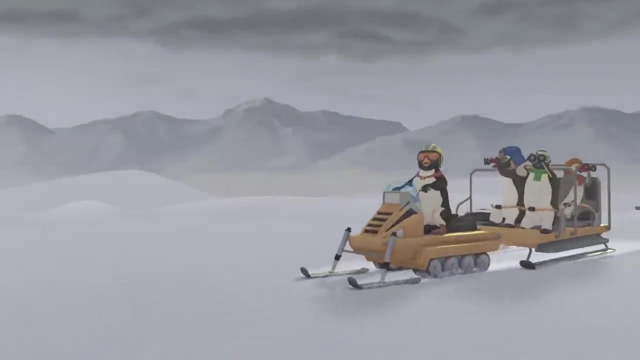 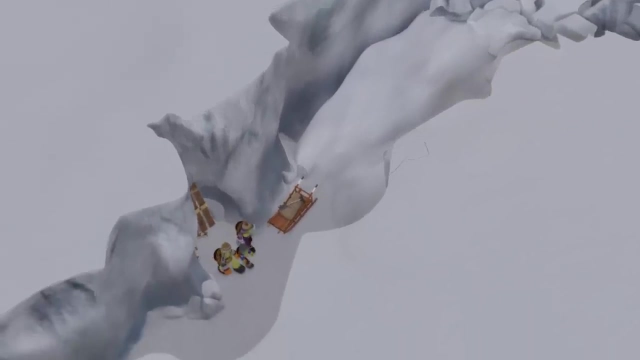 we'll ski back to the ranger station and, Whoa, What was that The path? It's gone. It's okay, We'll find another way out. Turtles, Turtles, Franklin, We need to find a way out of here. 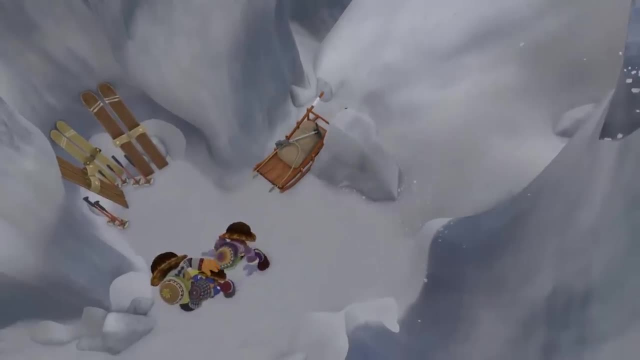 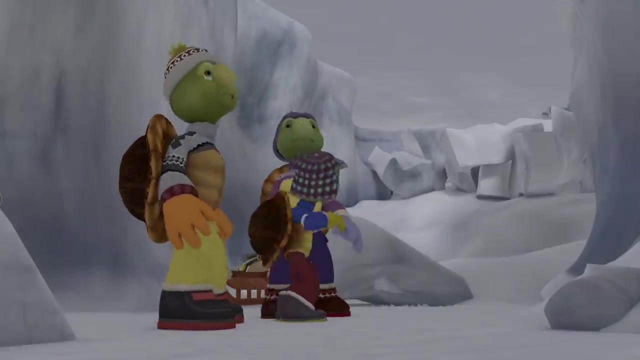 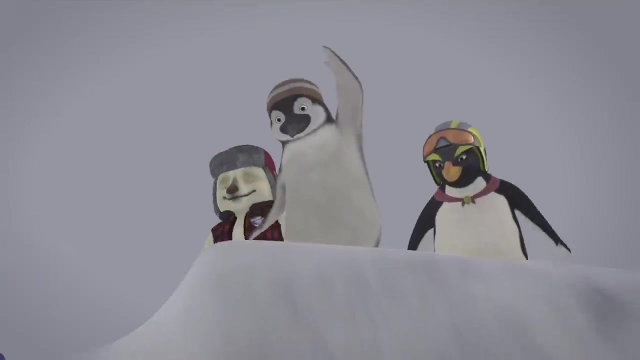 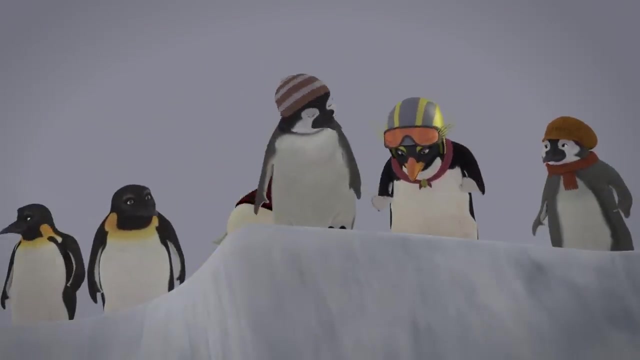 Look out, Phew, Everyone. okay, Hello, Franklin, Mom, it's Pip Pip. We're down here In the valley, Hey guys. Well, hello, Are we ever happy to see you, Pip Woohoo. 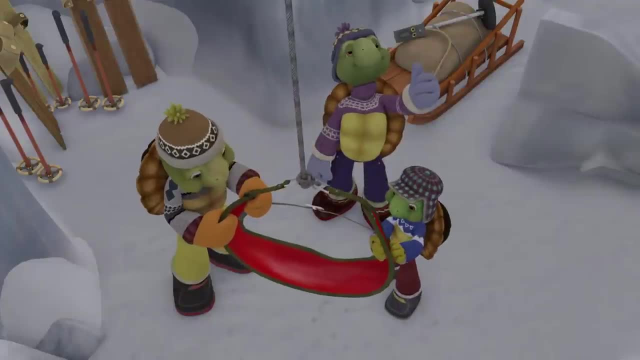 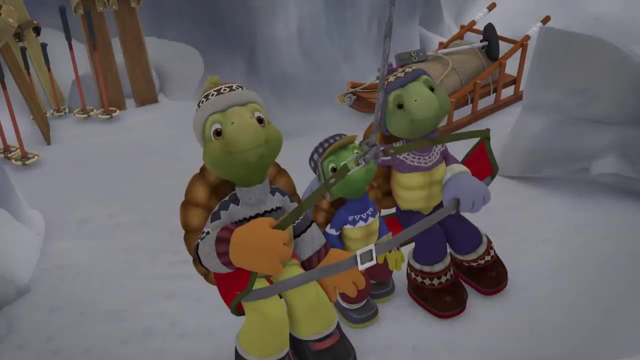 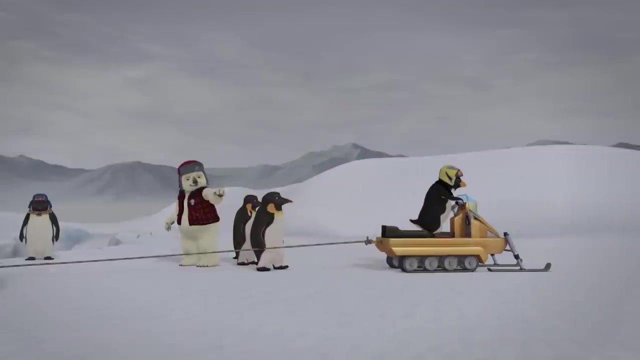 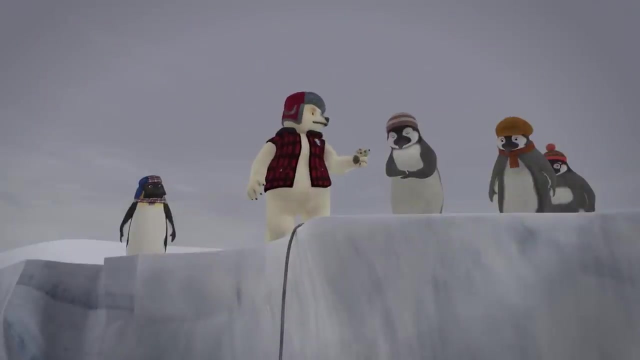 Hi everybody. Oh, there you are All set, Ready turtles All set. Hold on. All right, Here we go, Steady, Steady, Here we go. It's working Almost there. Hang on, Franklin. 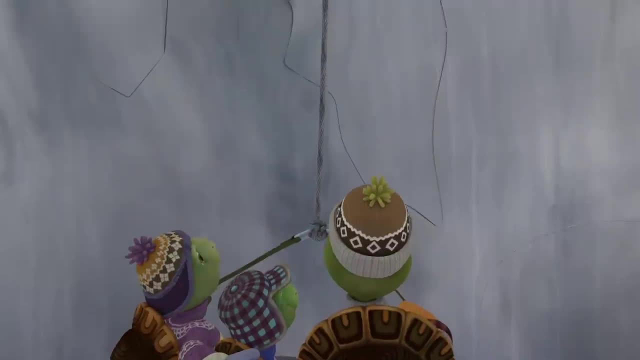 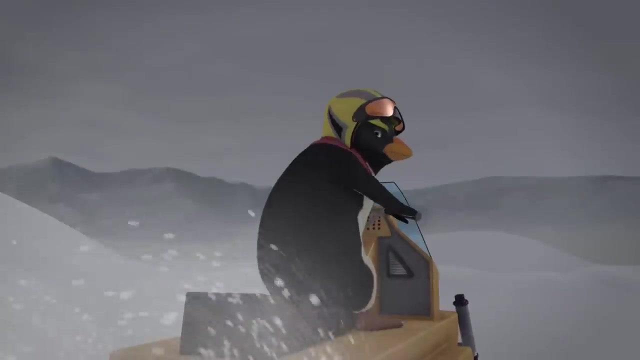 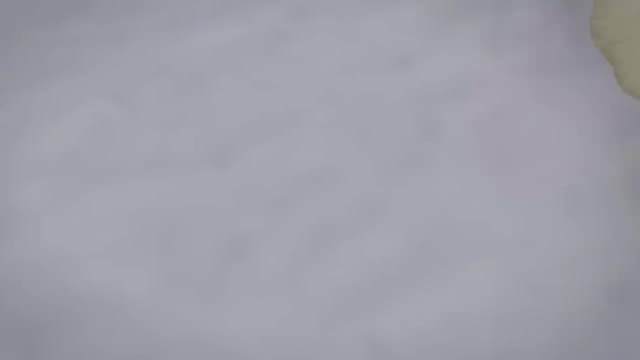 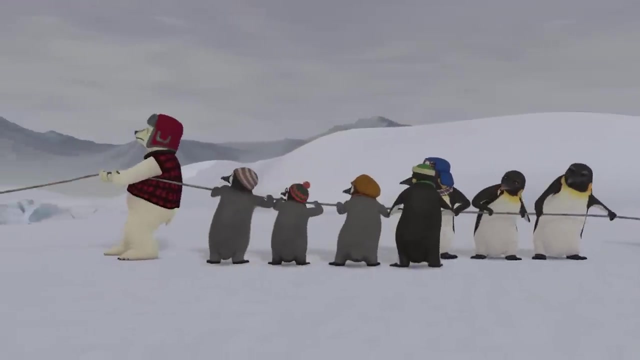 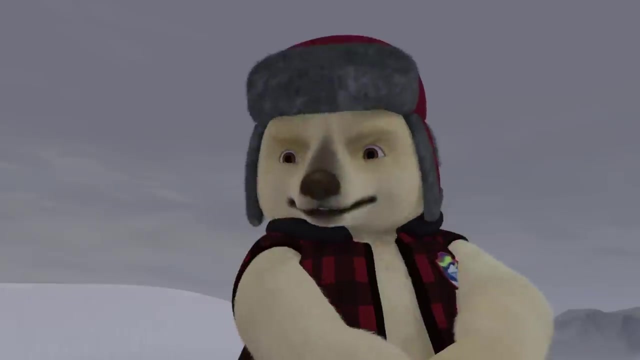 This is not so bad, huh? Oh no, Hurry, I'm stuck. Come on, We gotta help Ranger Bear. Hold tight, Don't let go. That's it Come on, Hang on. Yeah, You can do it. 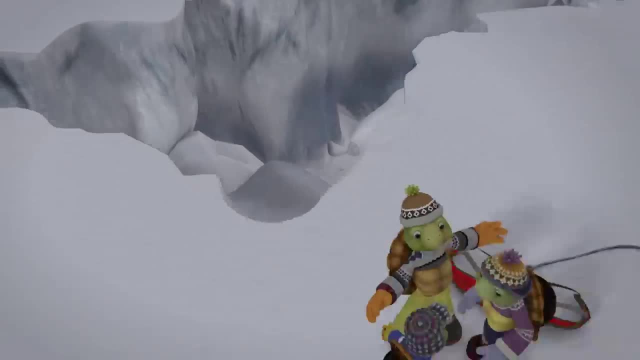 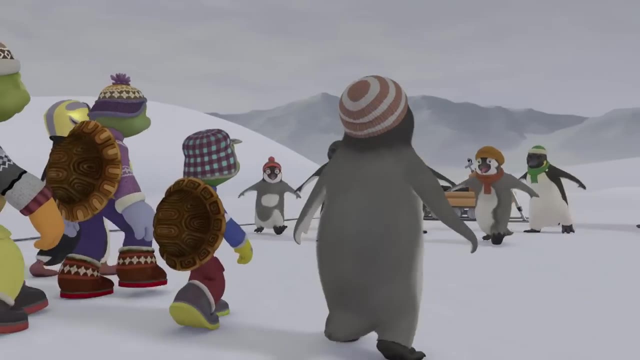 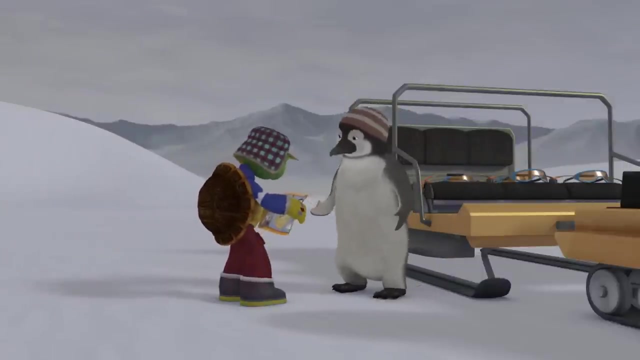 Yeah, Hold on Everybody. okay, We're so happy. you're okay. That was scary, We're just happy. everyone's safe. Franklin, follow me Right behind you. Pip, What is it? Look, I got the map. Um, that's great. 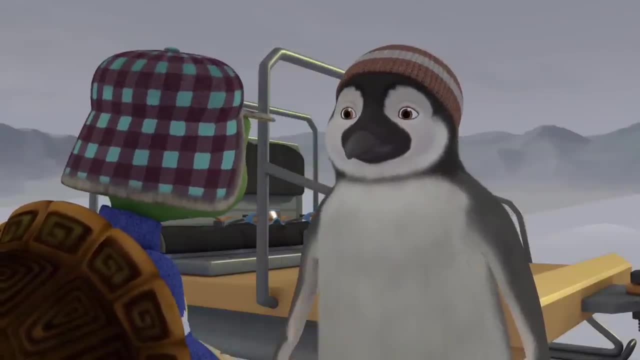 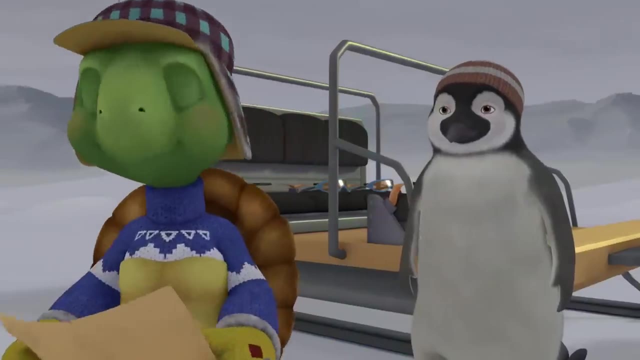 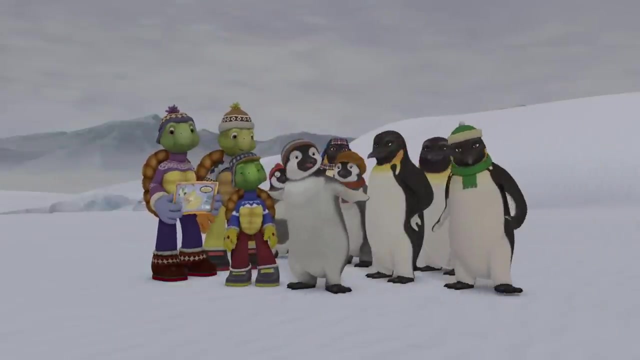 Thanks, I'm sorry I made such a fuss about it. I'm just happy you're okay. Right back at you, mate. Wow, Mom, Can you take the map from now on? Of course, sweetie, Come on Franklin. 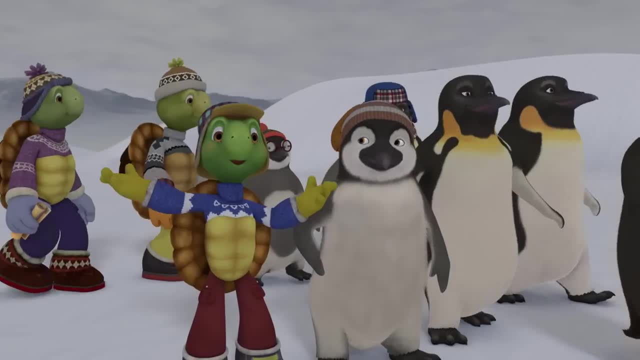 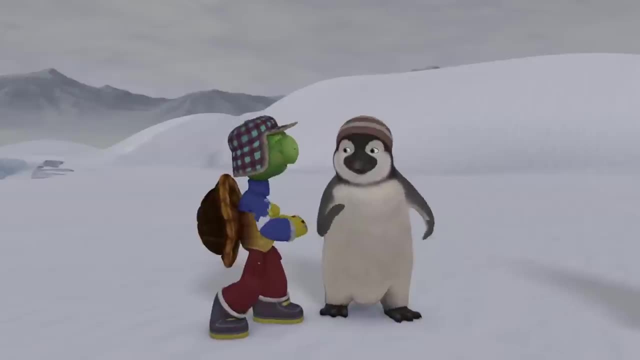 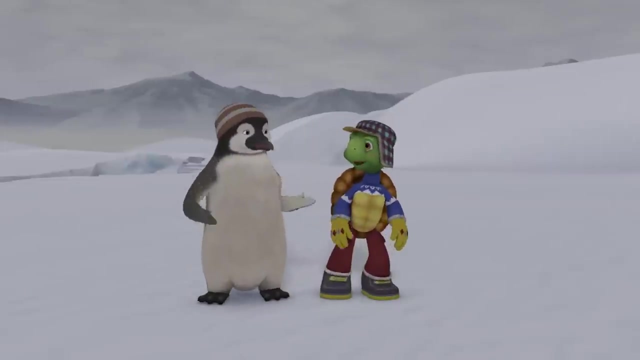 We can still find the treasure. Okay, folks, All aboard Treasure. here we come, Explorer handshake. You bet Wiggity, wiggity, wiggity, wow Zing Hop. Hey, we did it. 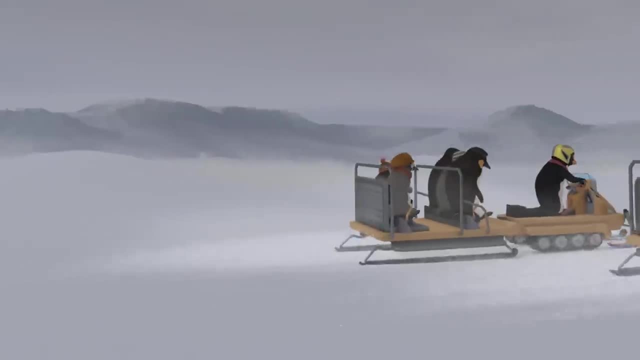 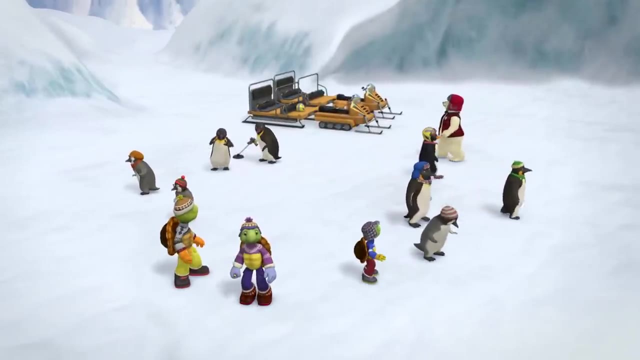 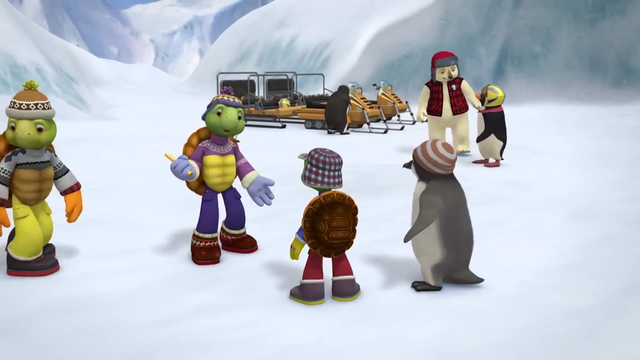 Yes, Any luck over there, Mr and Mrs Penguin. Not yet No treasure of the South over here. I don't see anything, Me neither. Well, the map shows that this is the right spot. It's odd for Great Aunt Harriet not to leave us some sort of sign. 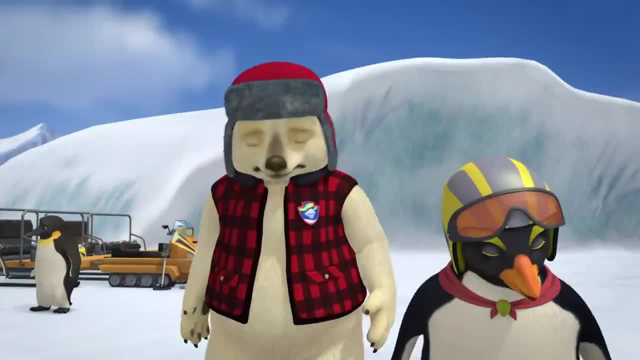 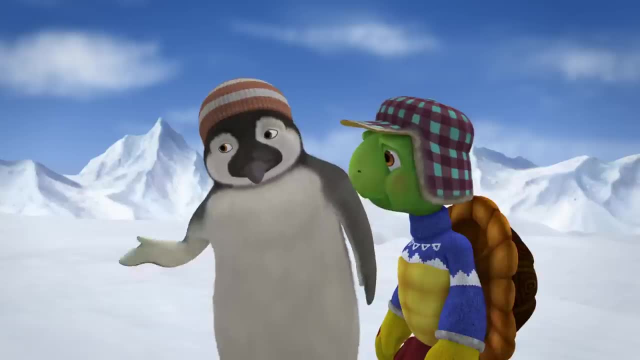 I'm afraid there's nothing here. Oh no, Oh, such a shame. Sorry, mate, I guess our adventure is over. Wait a second, guys, Don't be sad. It doesn't matter that we didn't find any treasure. 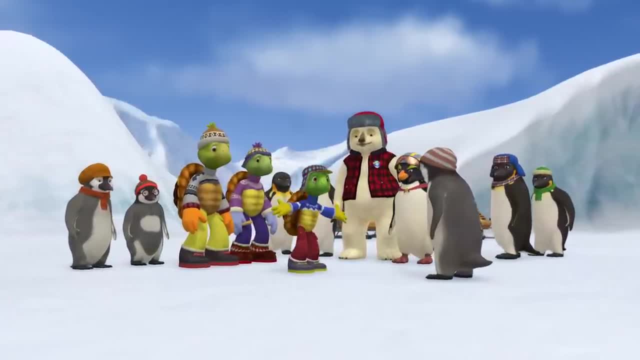 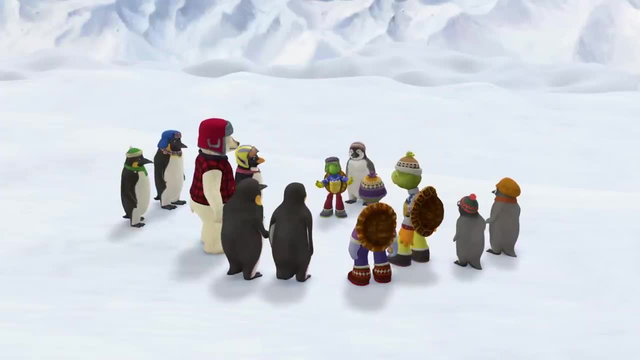 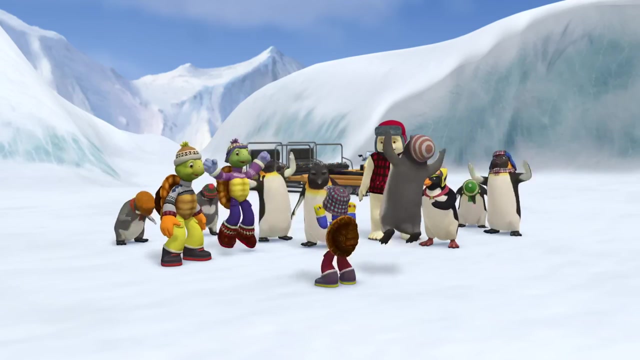 We still had an amazing adventure, built an igloo, rode awesome snowmobiles, made great new friends, and now we're here together on this cool little mountain. That feels like a treasure to me. Yeah, me too. Good on you, Great Aunt Harriet. 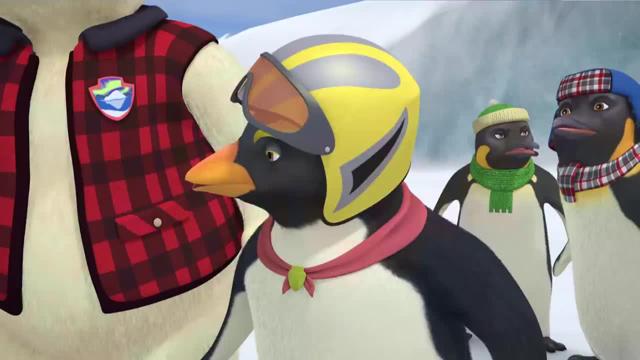 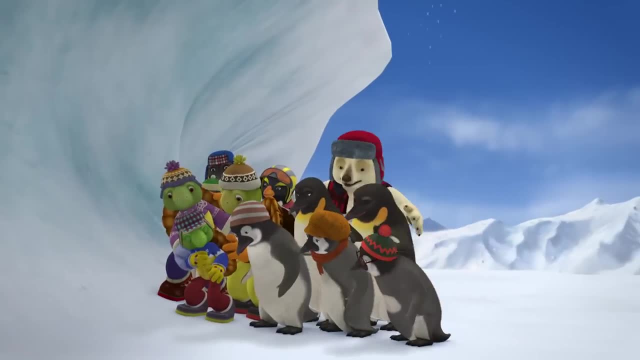 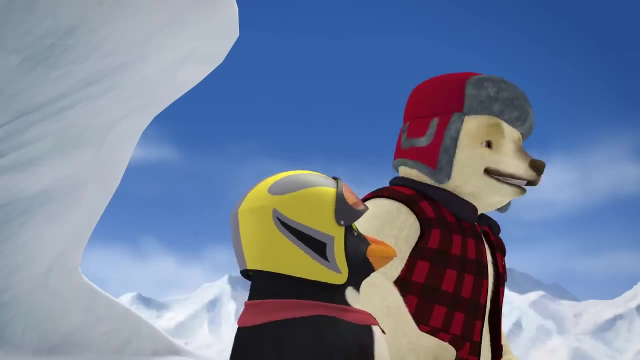 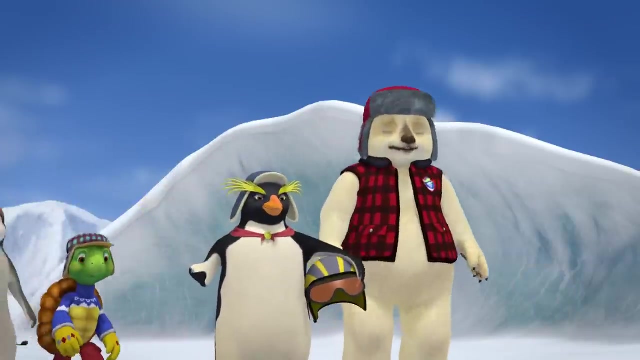 Yay, Oh no, Avalanche, Take cover everyone. Come on everyone quickly. I think it's over, folks. Come on, Grinny, Let's check it out. Wow, Kids come, look Awesome. 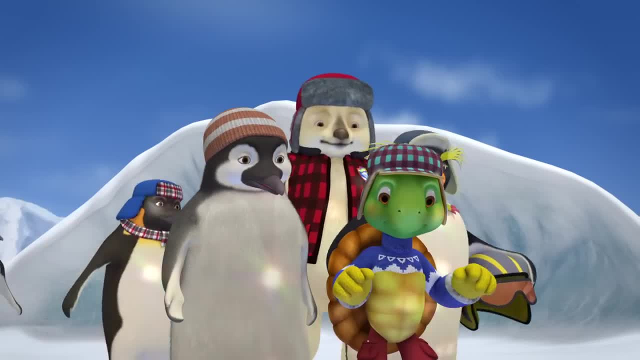 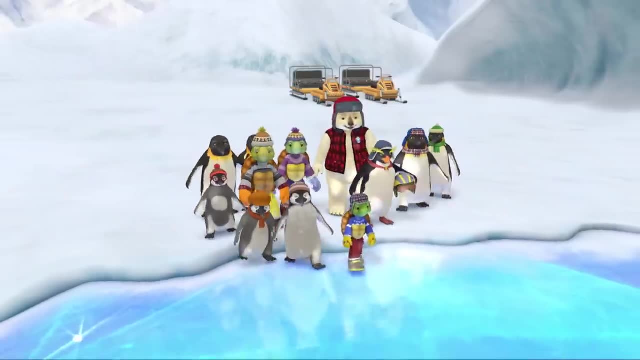 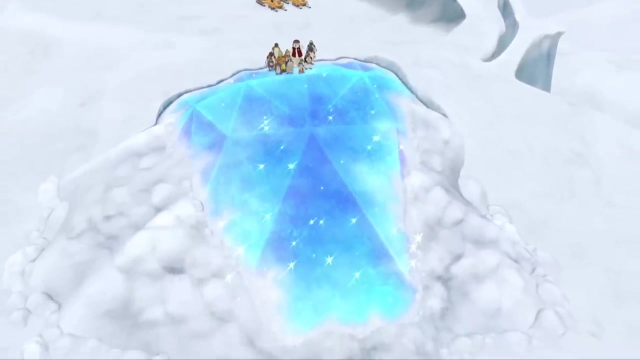 It's so bright. I've never seen ice that shines so bright, Like it's made of jewels. The treasure of the South. The treasure of the South. This is what Great Aunt Harriet wanted us to find Wonderful. I've never seen anything like it. 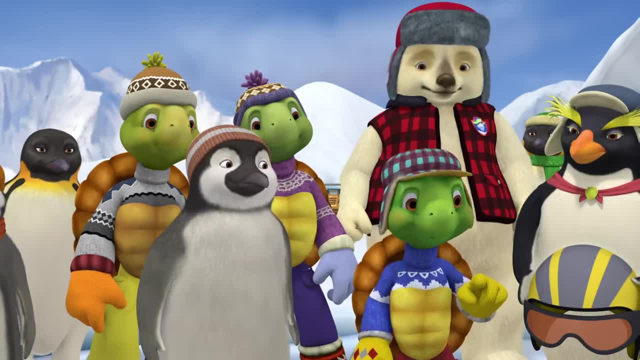 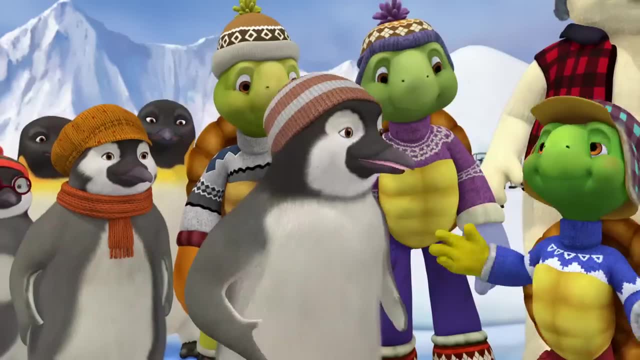 Nicest ice I've ever seen. We've seen northern lights and southern gales And so many coolio sights. We flew, we skied, rode snowmobiles, Built an igloo for the night. I've always dreamed I'd explore the world. 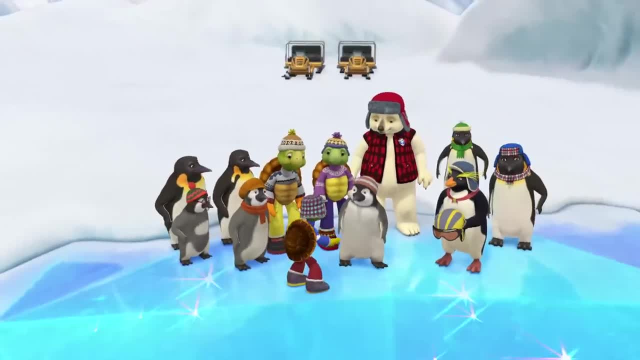 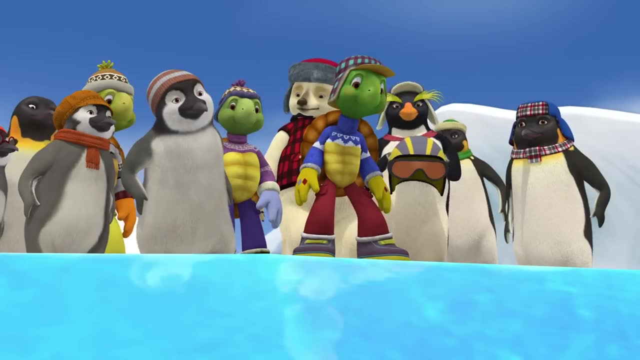 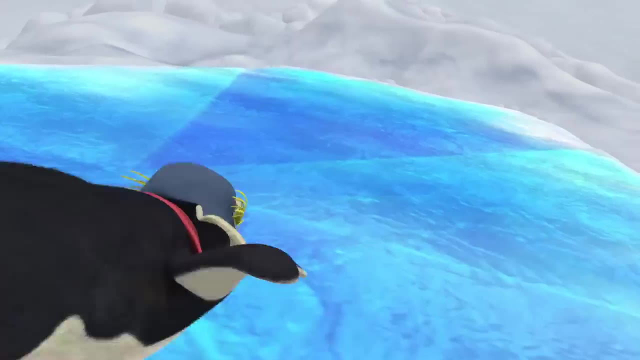 All the cool stuff you'd see, But being here with all of you Feels like treasure to me. Beautiful, Well said sweetie. Here you go. mate, I don't know what your Aunt Harriet did when she found the treasure. 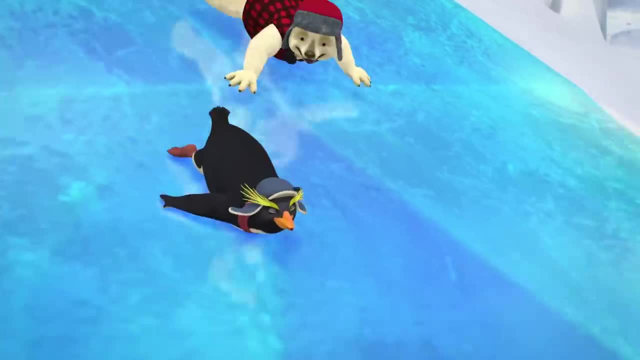 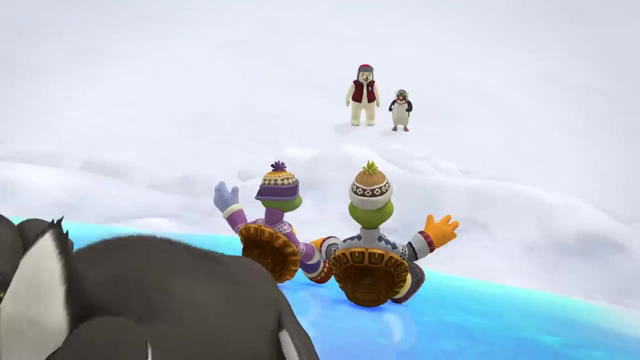 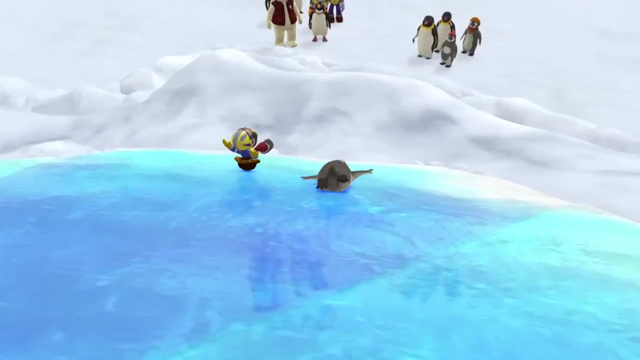 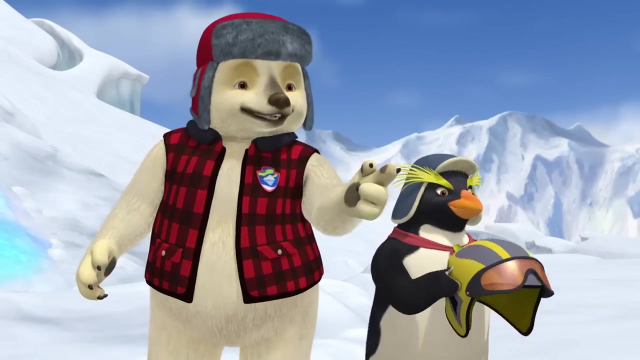 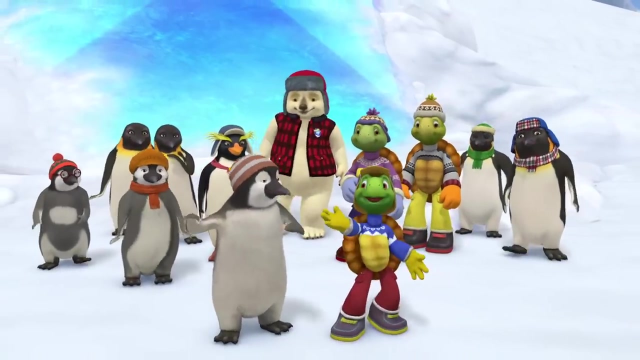 but I know what we can do. Wait for me, Winnie Explorers away. Franklin, you led the way. You were the one who made the day. We stuck together. That was the key to solving Harriet's mystery. 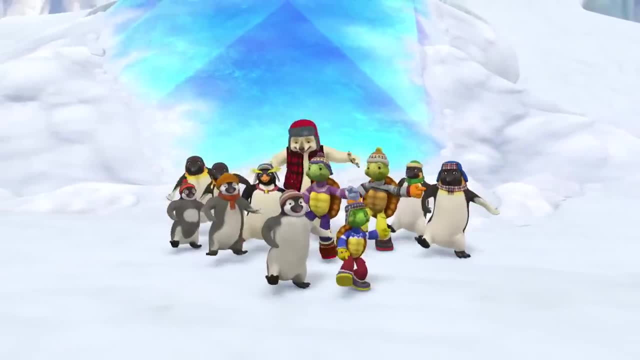 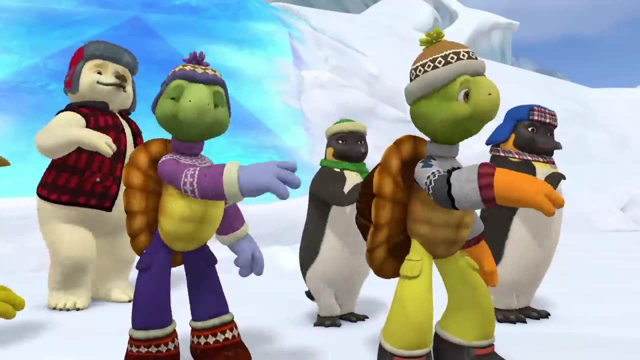 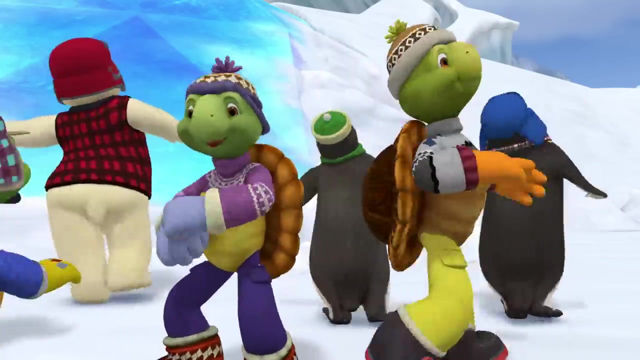 Treasure doesn't come with a key. It's in the world around us. Now I see We've followed the map, We've followed the signs. We've found jewels of many kinds. The shine in the eyes of friends I see feels like treasure to me. 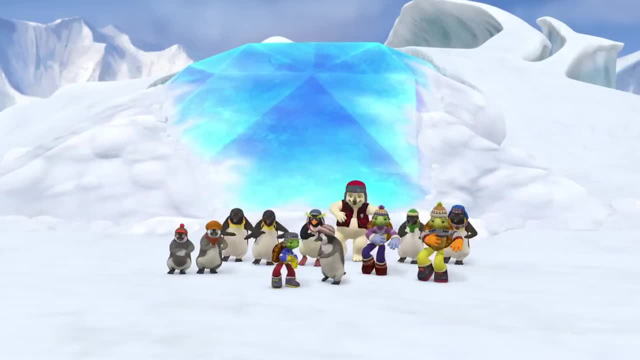 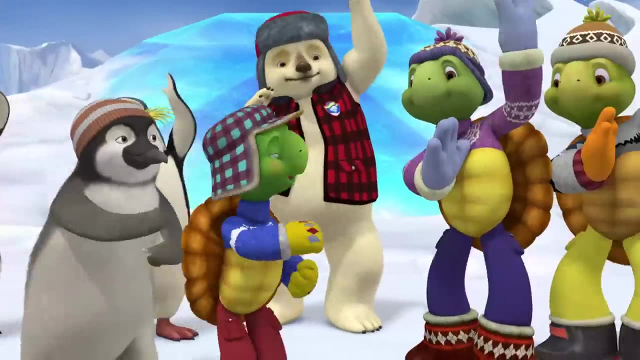 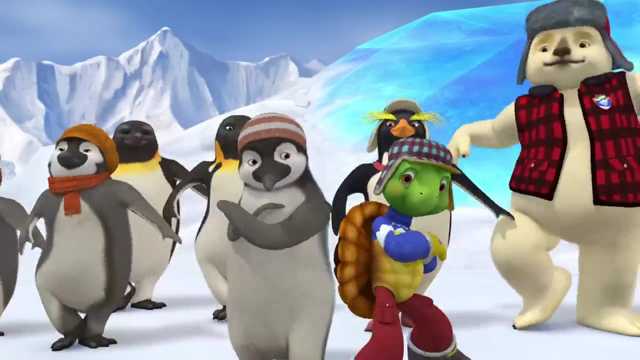 Treasure doesn't come in a chest, It's in the people around us. And you're the best. I learned to enjoy the ride with Mom and Dad and a buddy at my side. The very best part: in the end I made a new friend.